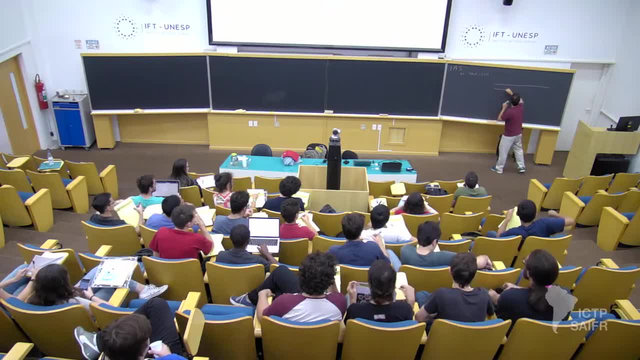 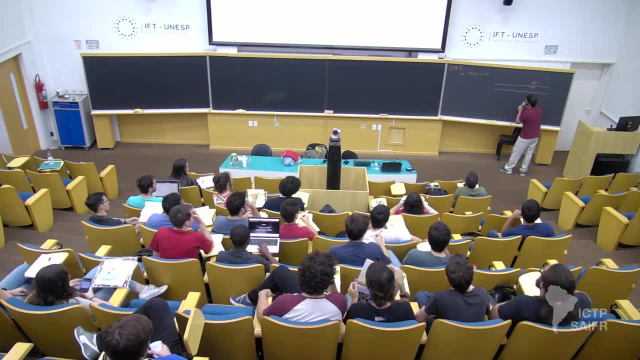 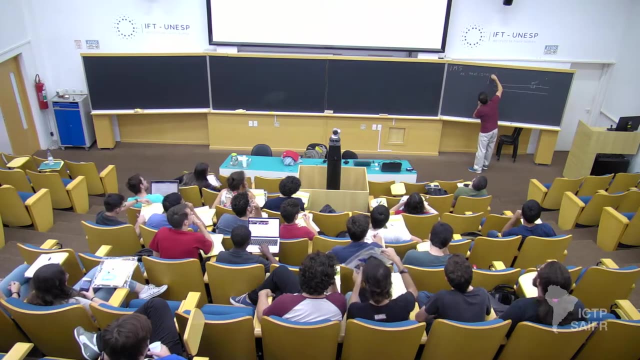 So if this is Paulista and this is our hotel somewhere around here, okay, This is the Trianon Maspi. There is also a good museum. I personally am not fond of it, but it's nice. And here is Consola South, is the Rua Consola South. 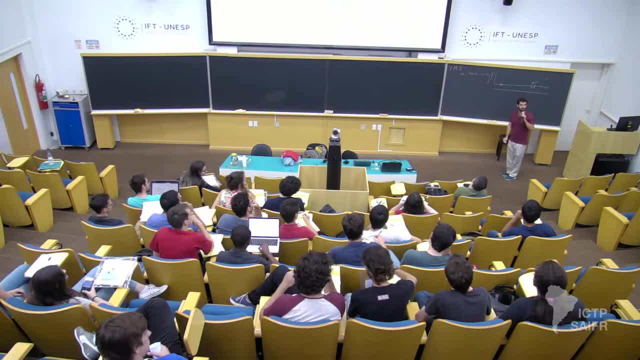 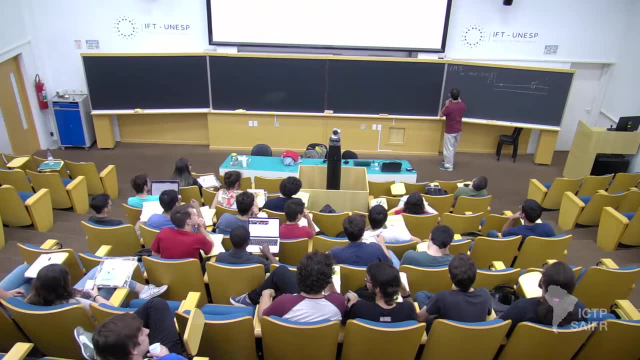 The Instituto Moreira Salles is somewhere over here. okay, I like it very much. There is also Museu da Imigração that I personally enjoy a lot, So you can check it out online. I think it's the stop. the metro stop is Bracer Moca. 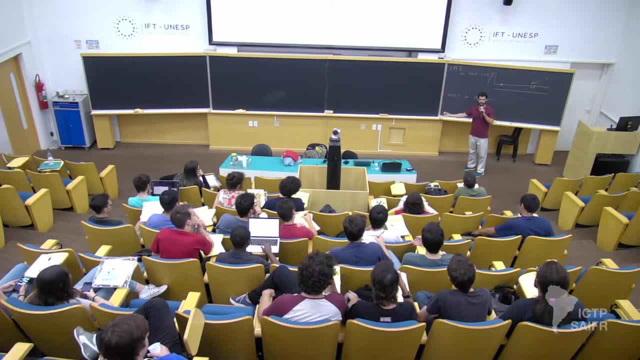 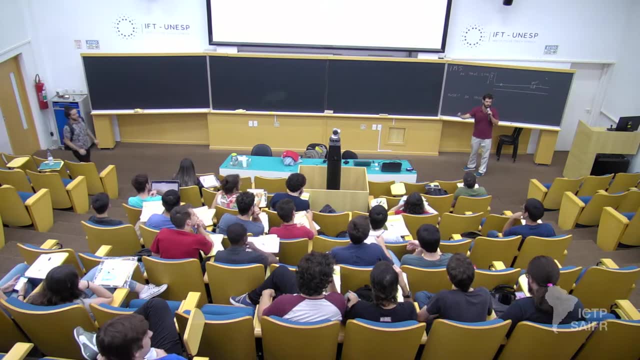 It's a safe walk from the metro And it's a big building: the villa where the immigrants were taken off the boats on the train from Santos to there And they were screened and the documents. So it's actually quite interesting. You have documents belonging to 100 years ago, 120.. 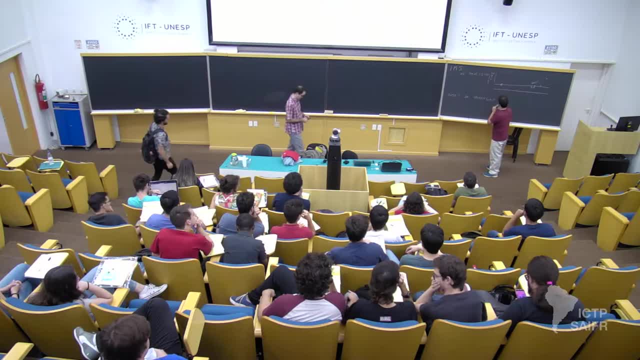 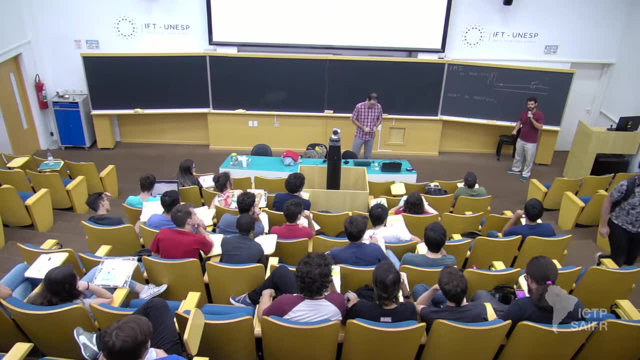 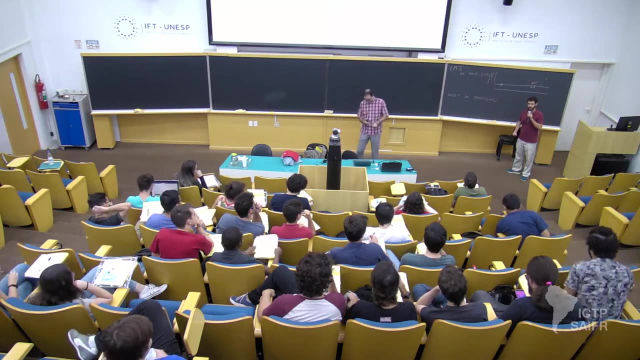 And there's videos, interviews to these people. Okay, so these for what concerns the museums. Then the city center. the historical city center is an extremely interesting place, but I would recommend actively not to go there, Especially not alone and especially not at night time. 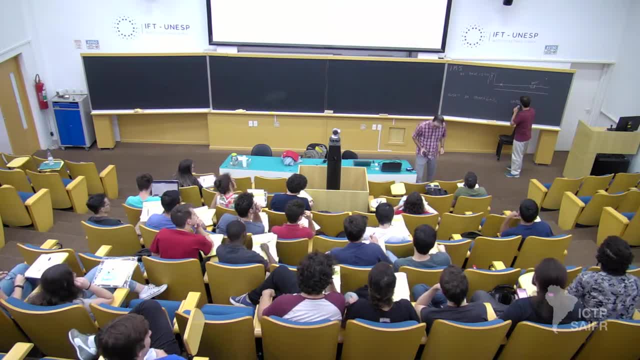 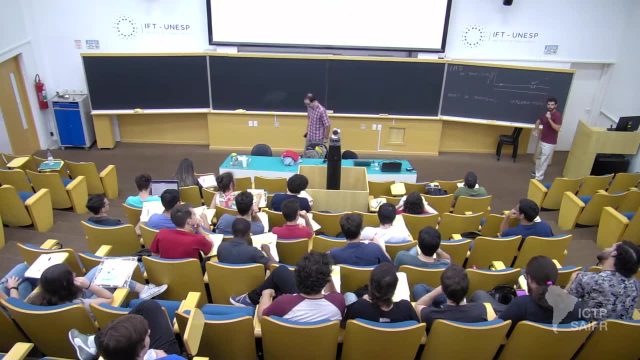 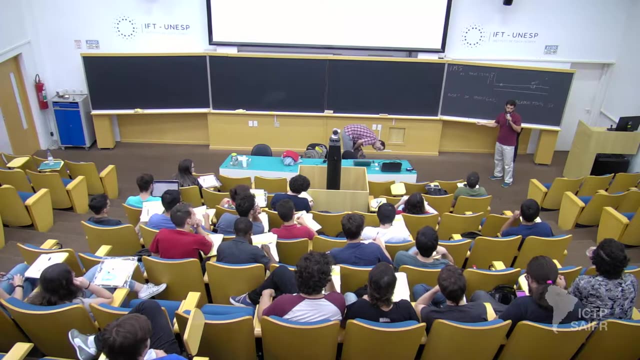 One very good way to take a walk there and enjoy it is to check the walking tour Sao Paulo or Sao Paulo walking tour online, And there is always a guide giving a talk either in English or in Portuguese in the morning or in the afternoon. 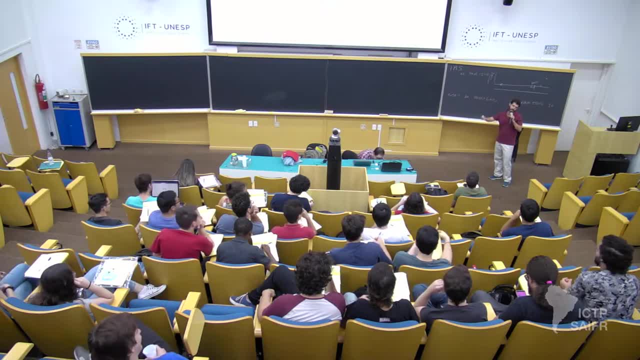 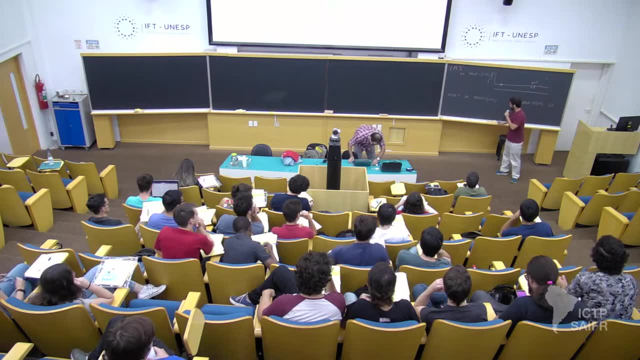 not after sunset, okay, And it's a safe. it's a big group, All right. This is for what concerns like more cultural events And since some of you didn't give me your word, I'm going to give you some different type of information tomorrow. 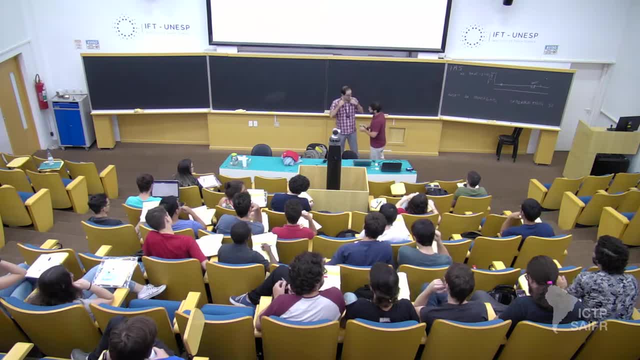 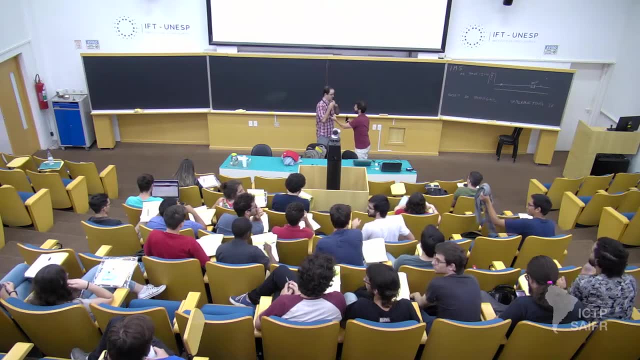 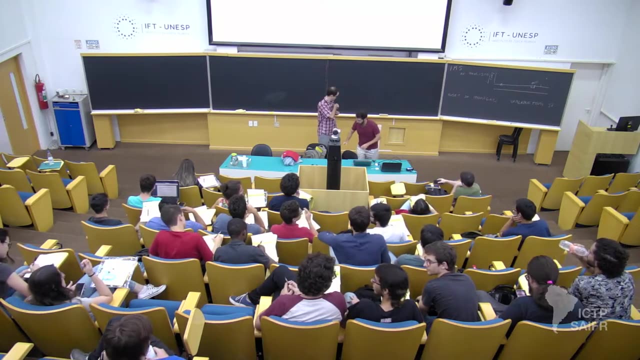 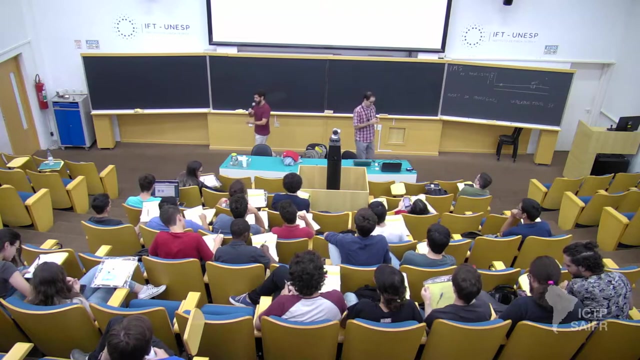 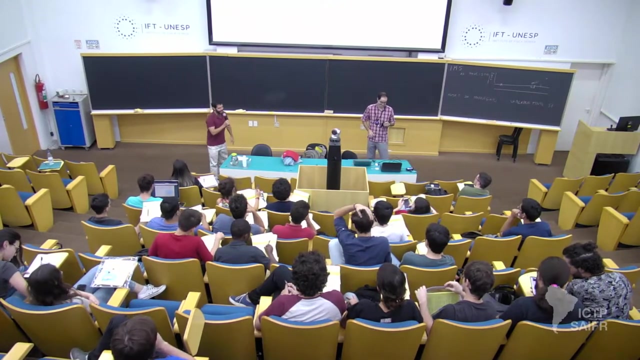 So Professor Neyman is currently professor at University of Sao Paulo, here in Sao Paulo, because University of Sao Paulo is also not in the city of Sao Paulo, but he's here in Sao Paulo. He was a graduate student in Porto Alegre, UFRGS. 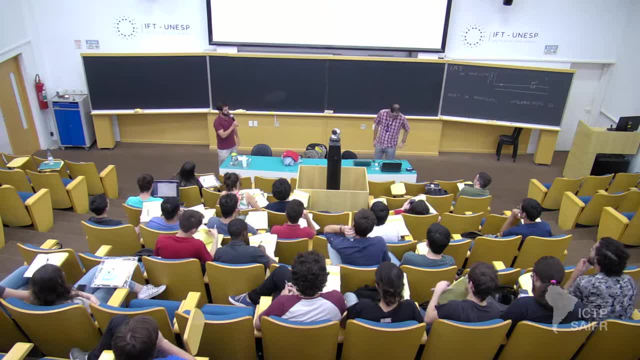 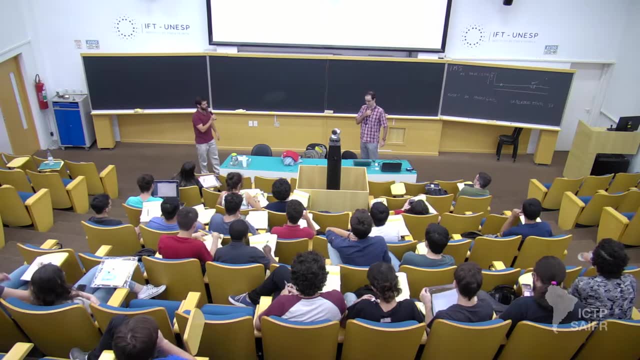 so Universidad Federal do Rio Grande do Sul, where he did his PhD, although he actually spent some time in the United States during his PhD, I think at Penn State, And he moved for a postdoc at NASA Goddard in Washington DC. 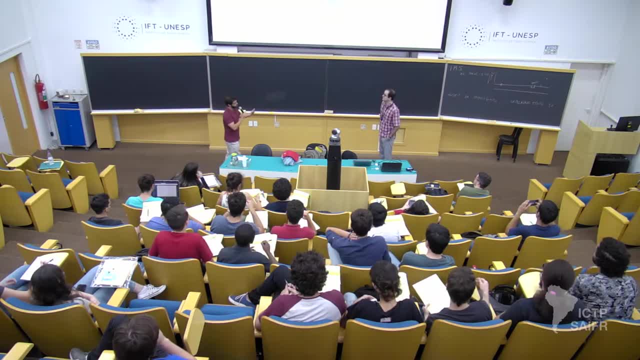 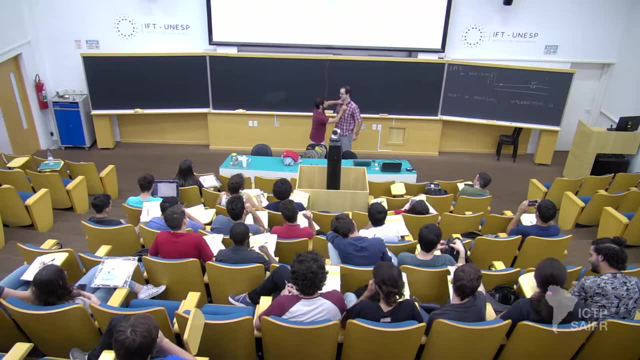 And then he actually got a professorship at USP. so he's back And he's going to tell us about AGNs and maybe I'm going to adjust your mic. So thank you, Rodrigo. Probably this way works slightly better. 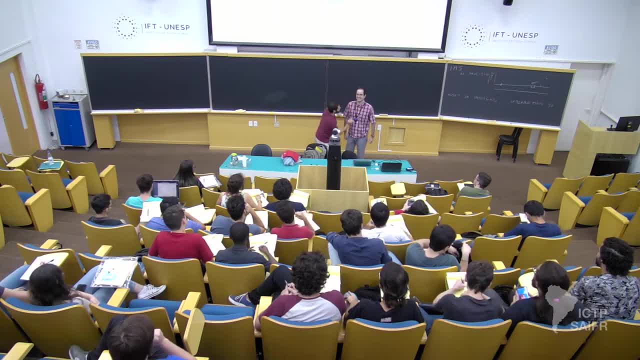 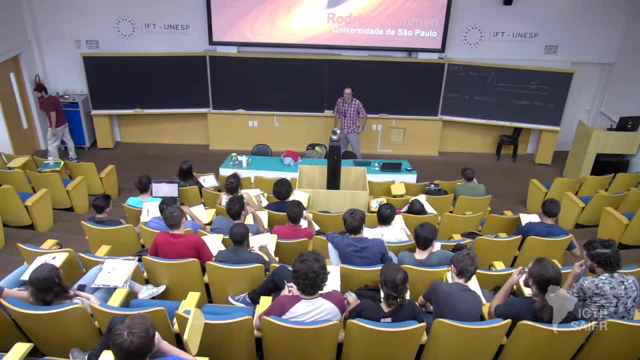 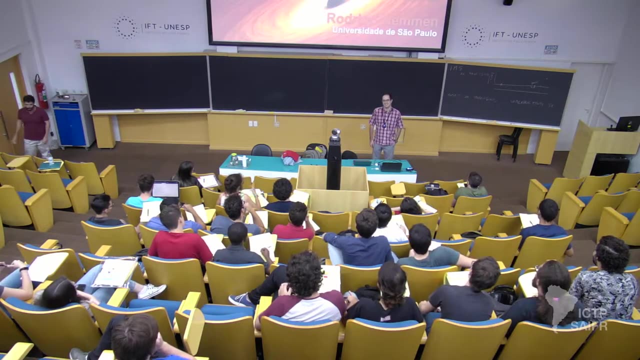 Yes, try it. Okay, Can you hear me? And I am well, this is being recorded right. Yes, Thank you, Fabio. Thank you for the invitation. Good afternoon everybody. Boa tarde, Buenos dias. 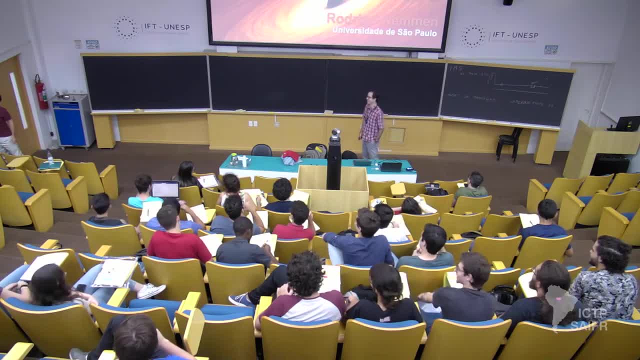 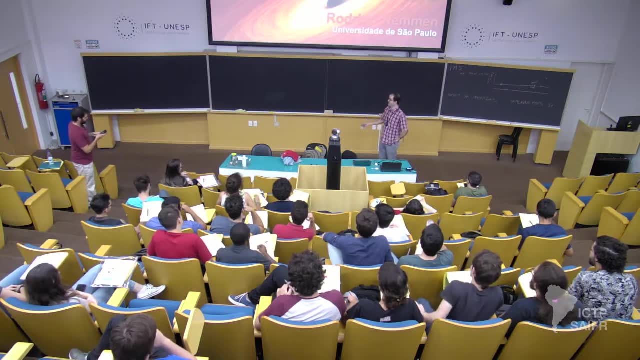 Ni hao, I guess I don't know. Konnichiwa Kalimera, Is there any in Greek here? No, no Greek, Okay, Ciao, right, Yeah, Okay, And that's it. That's it. 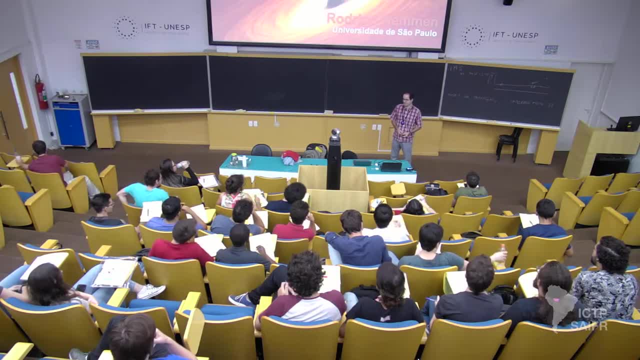 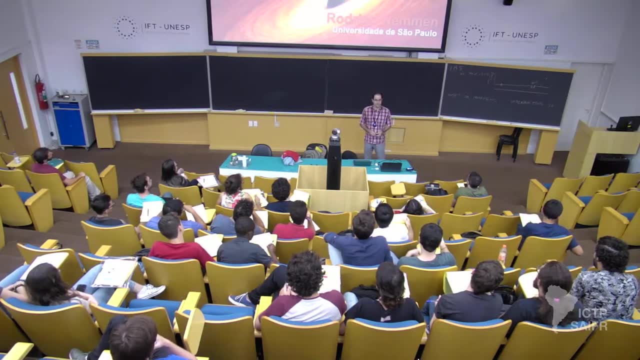 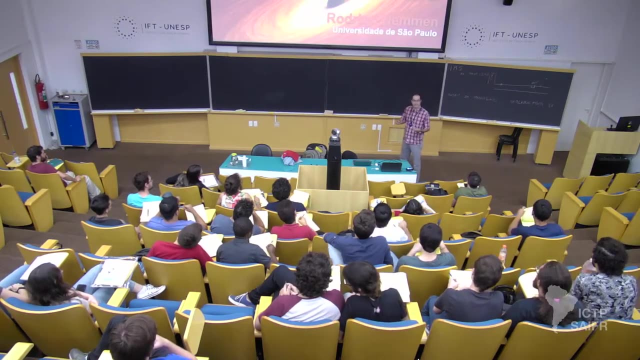 So today, we would like to give you, today and tomorrow, a very broad overview about active galactic nuclei and blazers, And I'm 100% sure that you are very excited with everything you are learning. Now you know how to accelerate things. 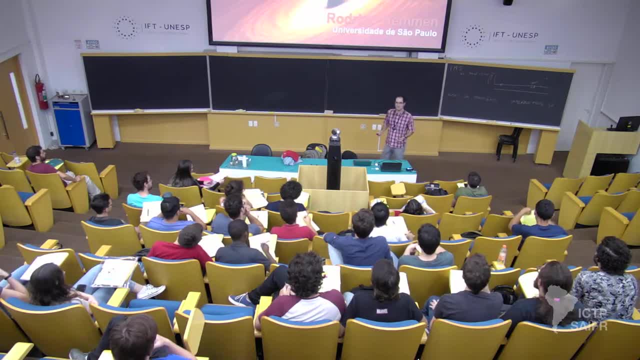 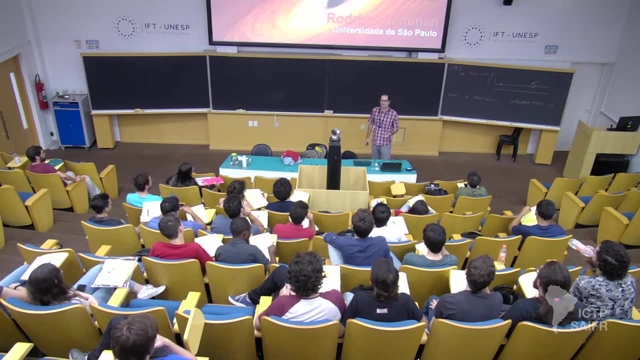 to take particles and put them in non-thermal distributions. I presume You know how to produce cosmic rays. You know how to produce neutrinos, You know the relevance of neutrinos. What else do they know? Fabio, They know a lot of things now. 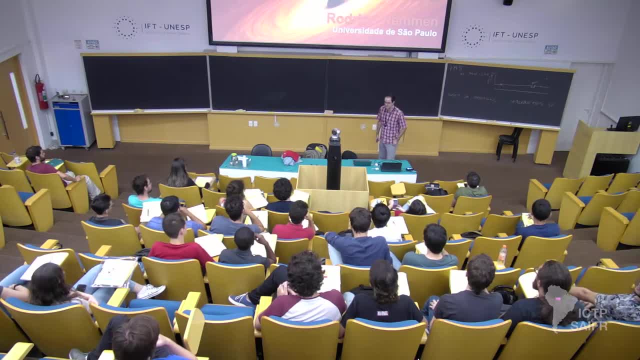 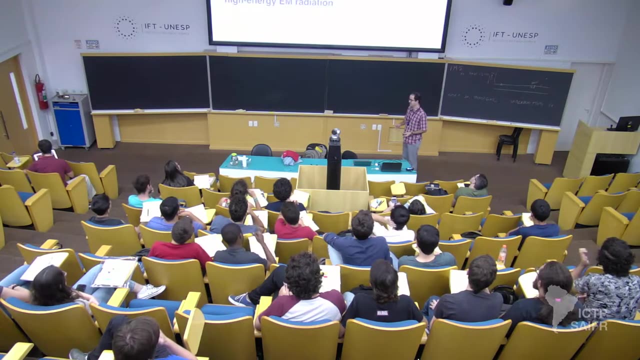 I'm sure you are very excited, And now let's see how some of this theory applies to the extreme universe. So the content of this lecture is the following: I will give the idea here in the next- well, in the next three hours, today and tomorrow. 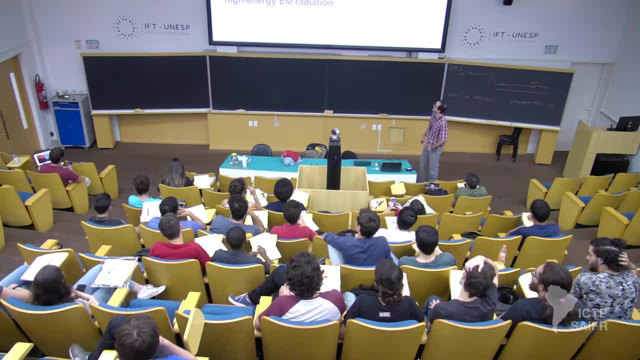 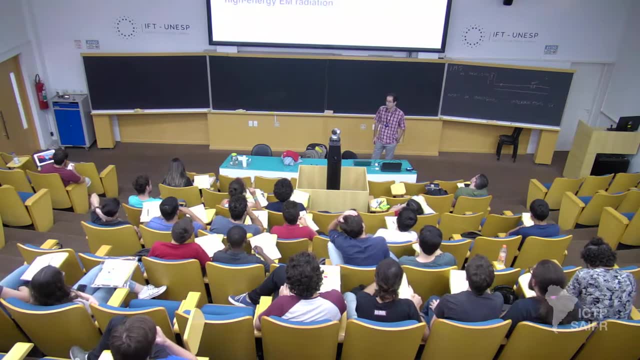 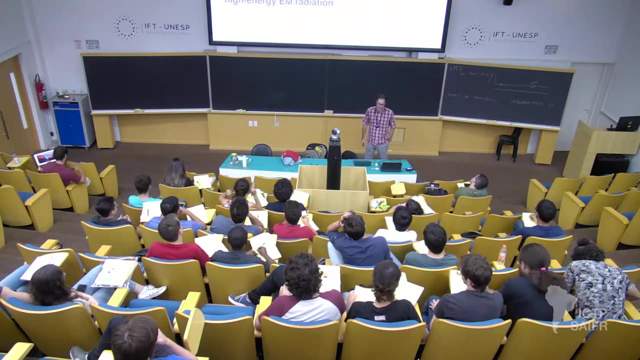 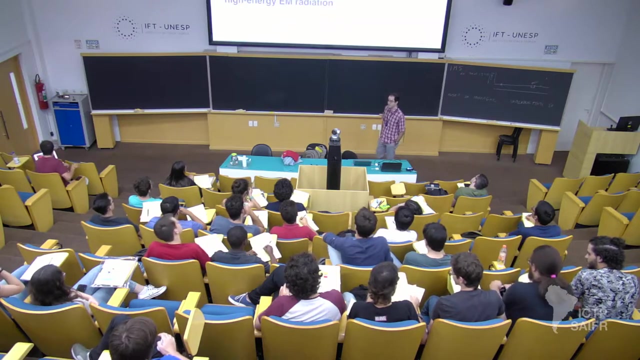 Right Today and tomorrow. So I will give a broad overview of the observations and theory of active galactic nuclei AGNs And I will put some definitely some emphasis on AGNs which produce relativistic jets. They are extremely interesting sources. 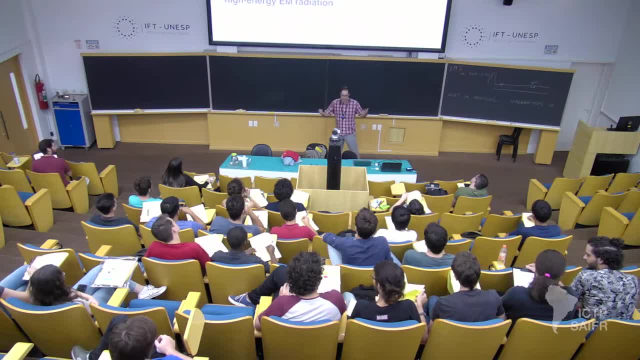 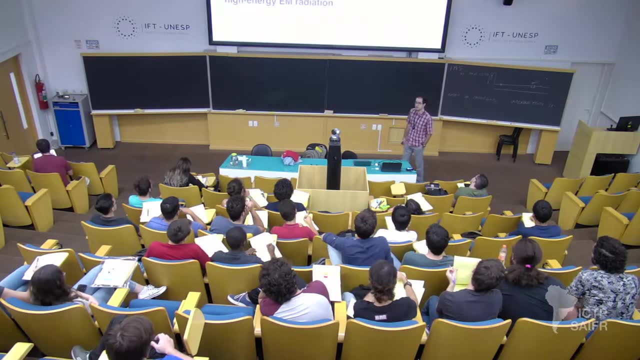 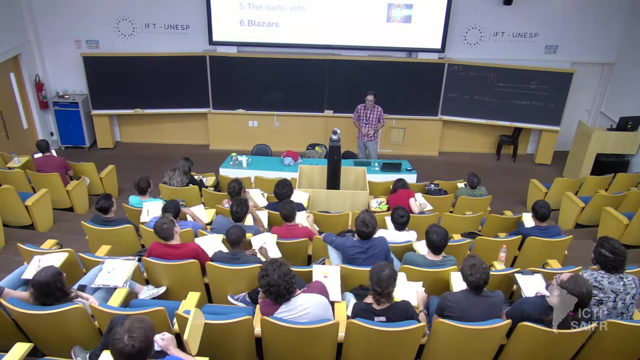 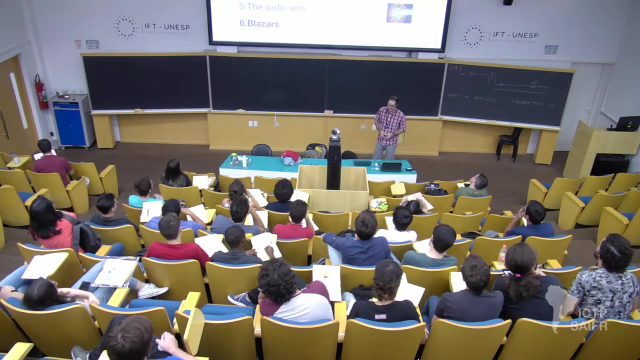 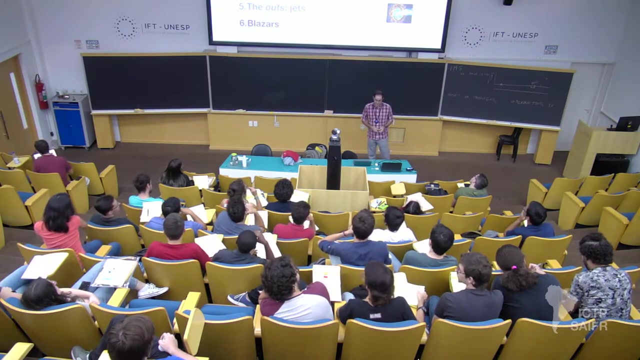 for the newborn, multi-messenger astronomy, And also some focus on high energy electromagnetic radiation in particular. The outline of these lectures is the following, So I will begin with historical perspective, Then some basic definitions about of black hole physics, Followed by a tour. 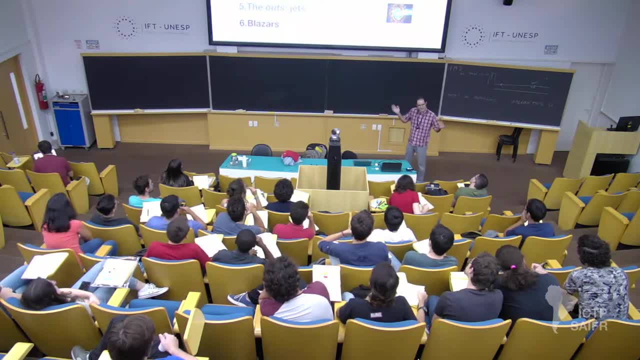 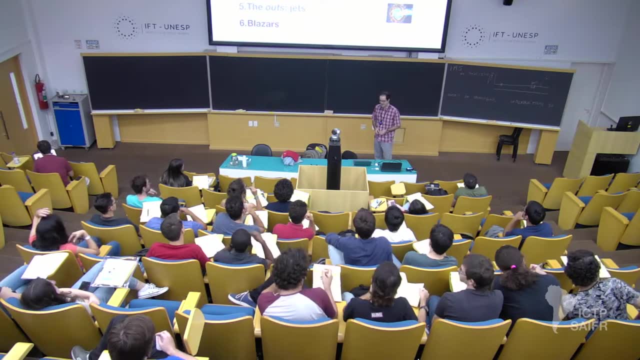 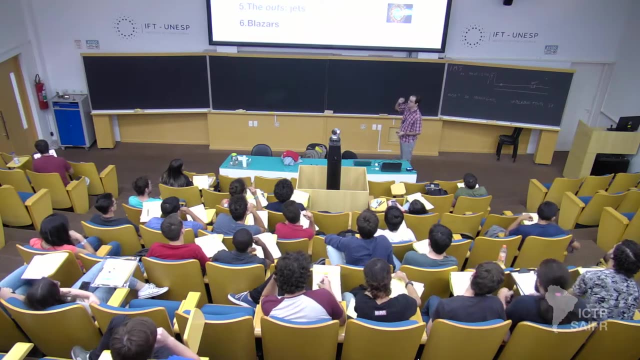 We will all go to a zoo, To the zoo of the extreme universe, And we will see the different kinds of creatures, animals we see there, The zoo of AGNs And well. so I don't know if you can see. 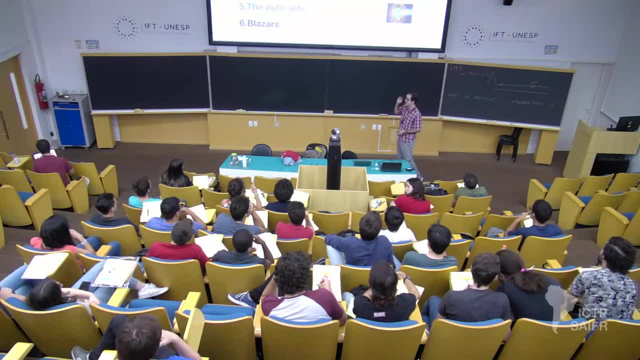 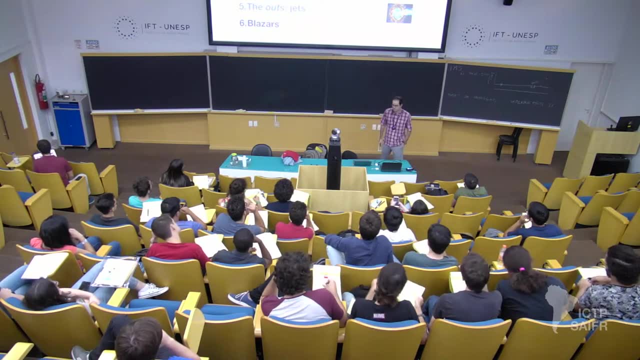 but I put in slightly different colors here. If I had more time, I will tell you a bit more details about the physics of black hole accretion flows And the physics of relativistic jets, But probably there won't be enough time. 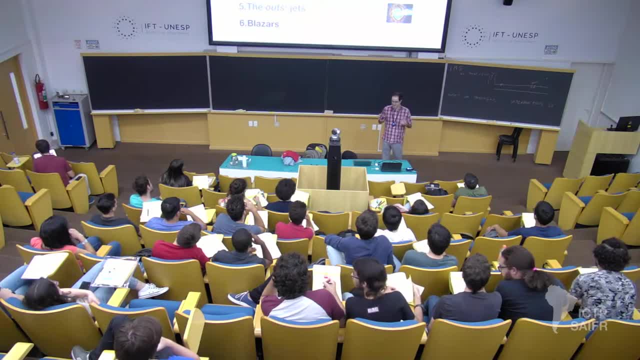 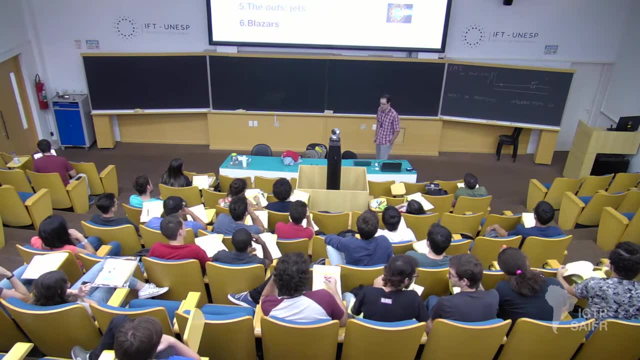 I will try, but I am already anticipating there won't be enough time to talk about accretion physics and jet physics- just a little bit. But let's see what we can do. And blazers: We will talk. we will spend some time talking about blazers. 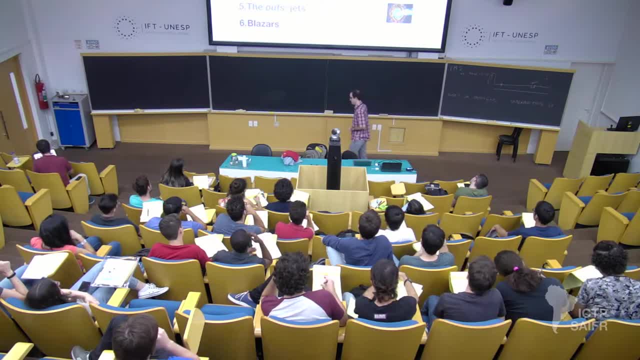 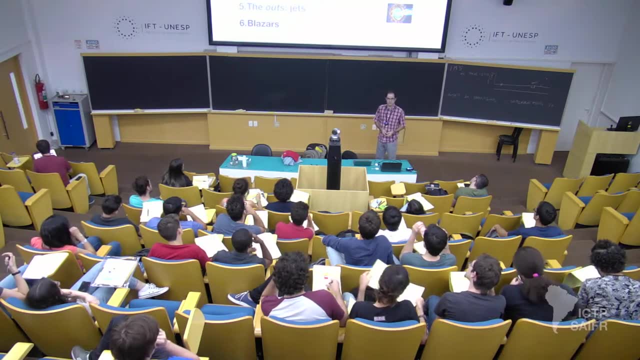 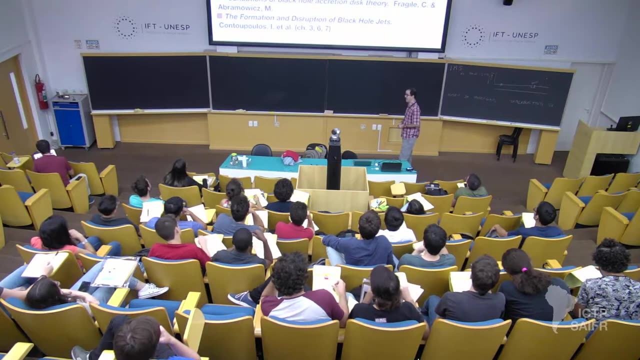 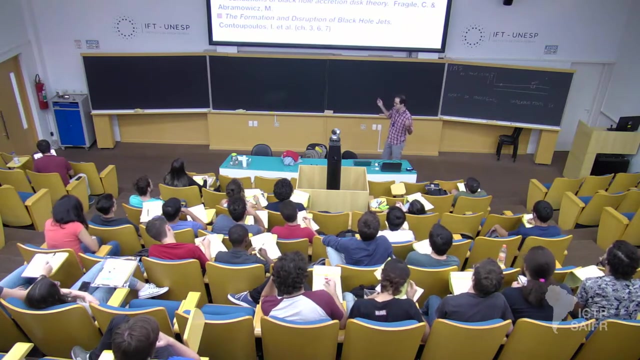 Sources of jets, Black hole bazookas pointing in our direction Here, towards our planet. So I thought it would be interesting to, before proceeding, to give you some references that you can go and study after the lectures are over Or, you know, tonight, tomorrow, on the weekend, if you want. 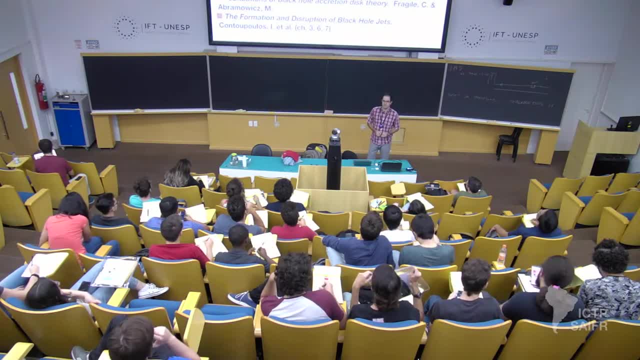 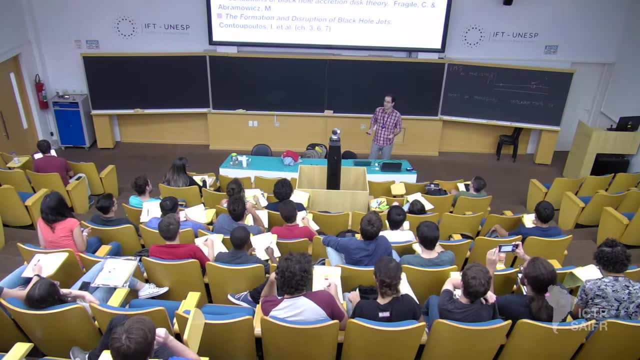 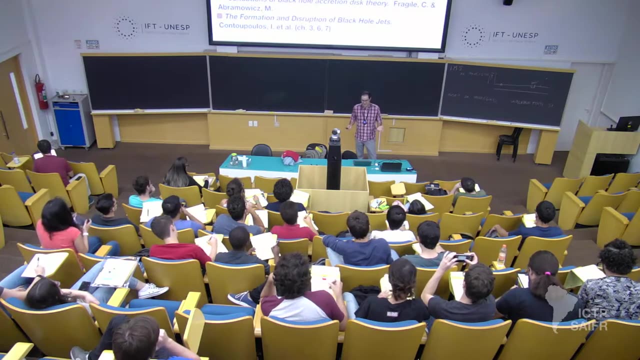 So for the theory of AGNs? well, the theory of AGNs is general relativity. It's a combination of general relativity electrodynamics- Yes, general relativity electrodynamics- well, radiative processes affecting radiative processes. 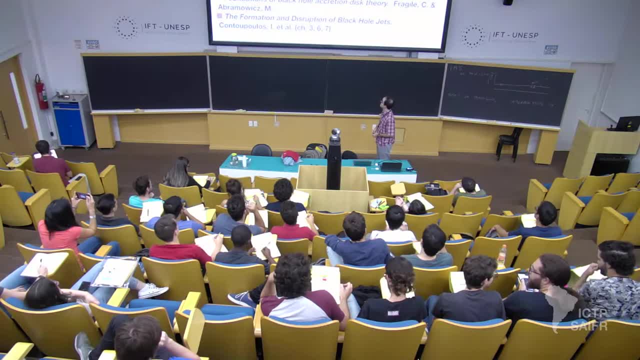 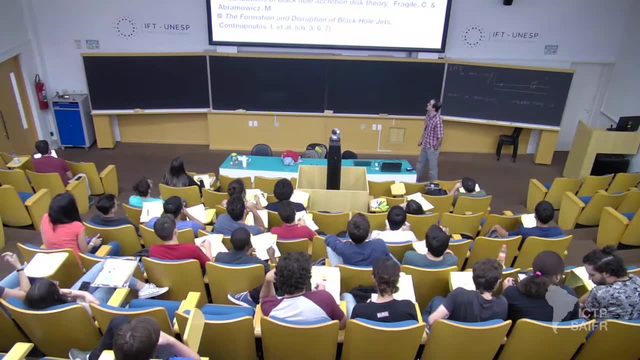 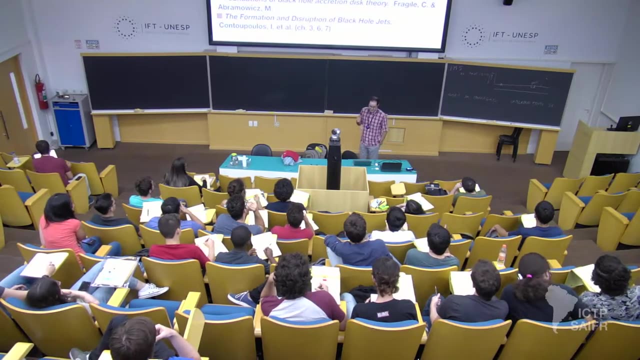 which is, you know, somehow, electrodynamics. So you need to study these things. This is the theory of AGNs, But there is a very nice summary of the theory necessary to understand AGNs in this old review by Roger Blanford. 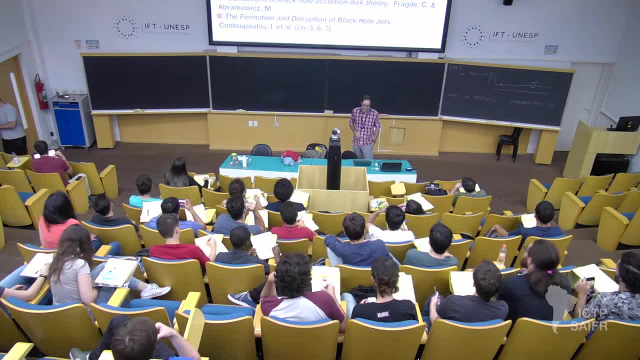 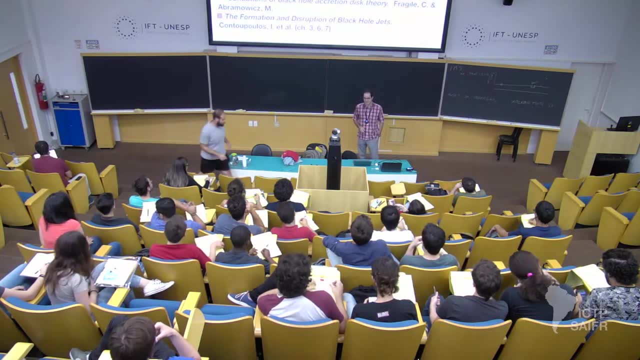 This review was published in these lecture notes that he gave at the Saas-Ferre AGN school 30 years ago, okay, 1990.. So well, the physics didn't really change, okay. What is improving following Moore's law? 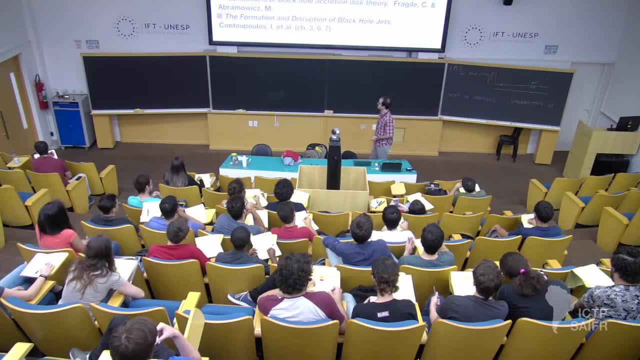 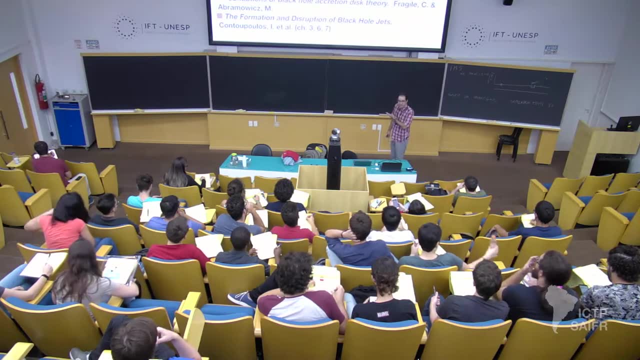 are computational resources, We are having insights, But general relativity didn't change And electrodynamics didn't change in the last 30 years. okay, And Blanford gives a very nice review, a very nice summary of the physics of AGNs. 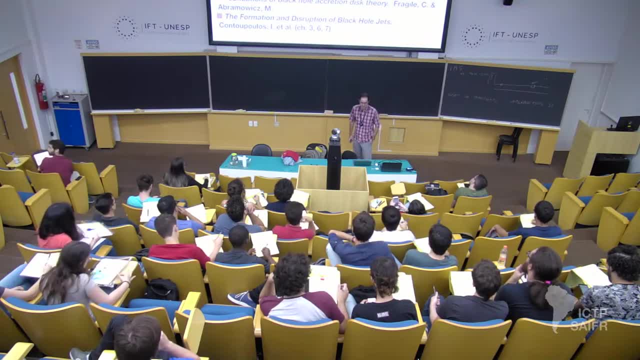 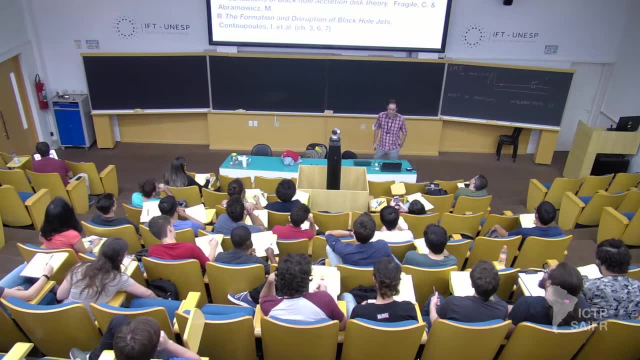 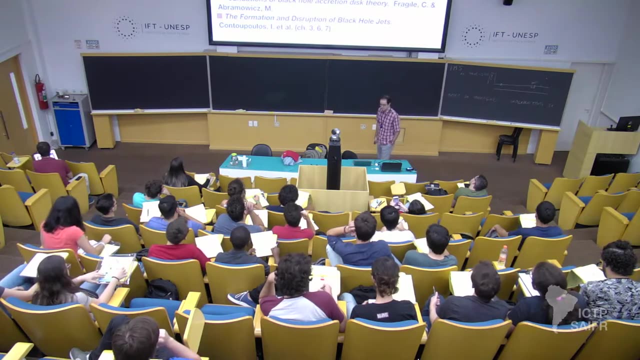 in these lecture notes physical processes in active galactic nuclei. The second work is a standard reference for compact objects. It's the book called Black Holes, White Dwarfs and Neutron Stars. It's a classic textbook in relativistic astrophysics. 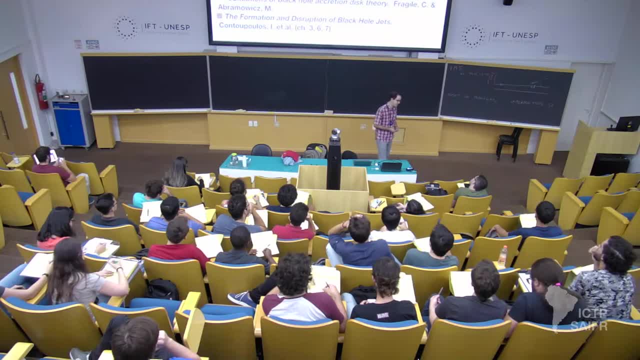 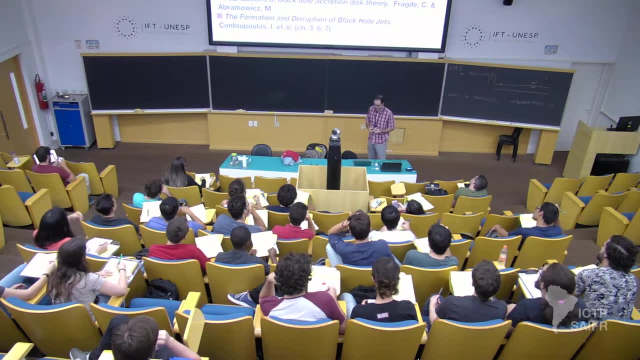 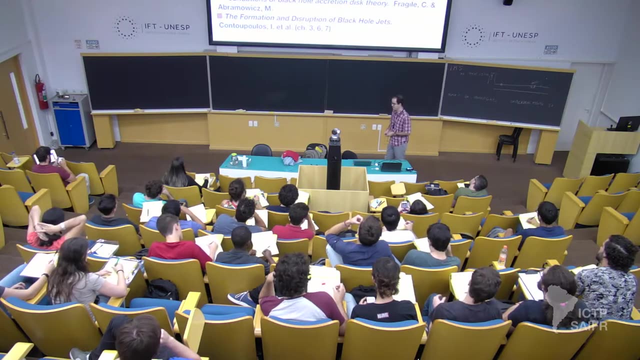 It covers a bit of the physics of black holes, physics of accretion disks. It's a very nice book by Shapiro and Tchaikovsky, And so if you have a look at these two first references, you will definitely get a good feeling of the theory. 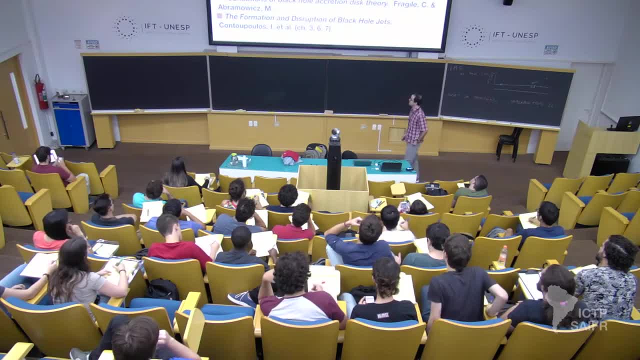 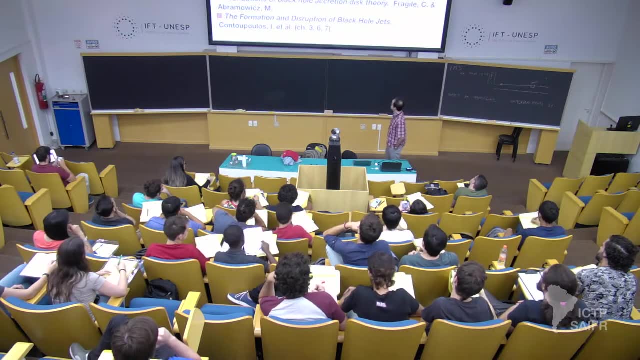 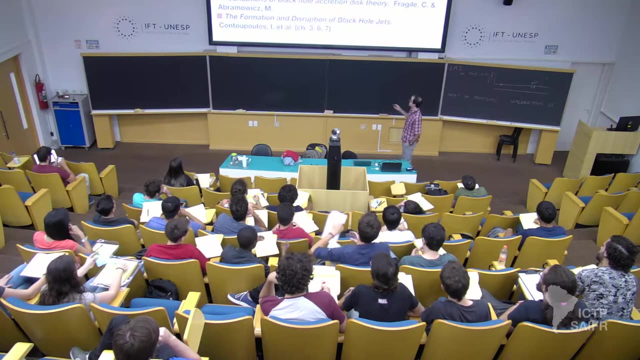 And if you want to get a bit more details, I suggest you have a look at this review paper by two theorists, Chris Fragiel and Marek Abramovich, Foundations of Black Hole, Accretion Disk Theory, And this is a review which has about 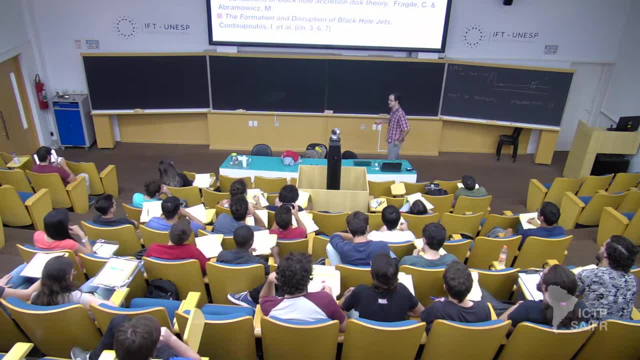 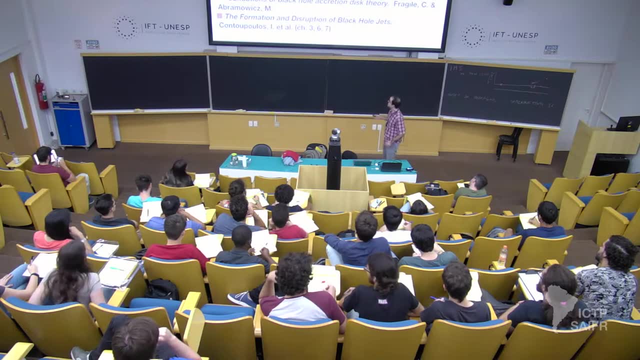 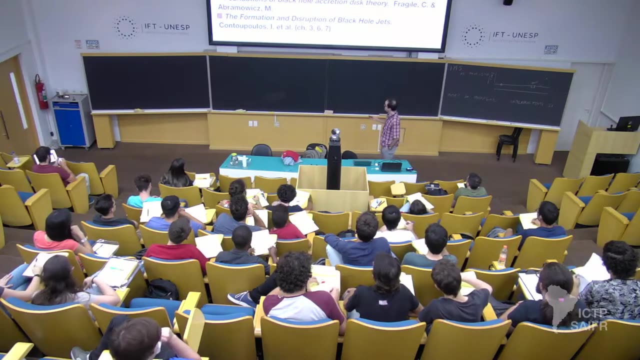 I think 20 pages. They use GR, they use the covariant equations to tackle the physics of accretion disks. And the second review is: if you want to have a good idea of the physics of jets, It's a book: The Formation and Disruption of Black Hole Jets. 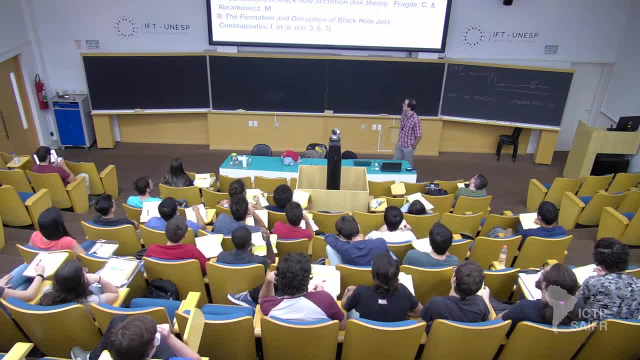 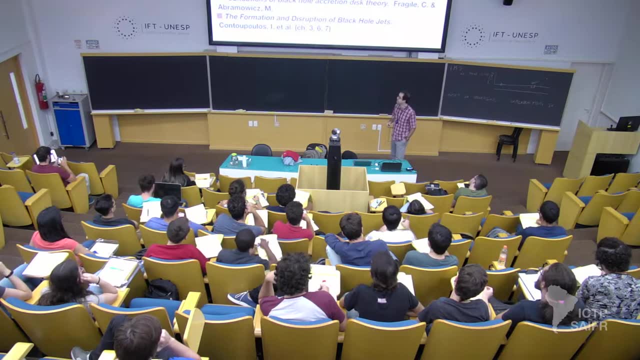 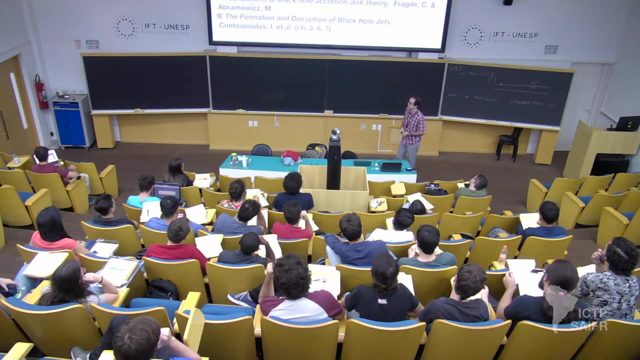 One of the editors is Kontopoulos, And in particular I suggest chapters 3,, 6, and 7.. They talk about launching of jets, the physics of propagation of jets. This is a really nice book. It has some of the leading figures in the field. 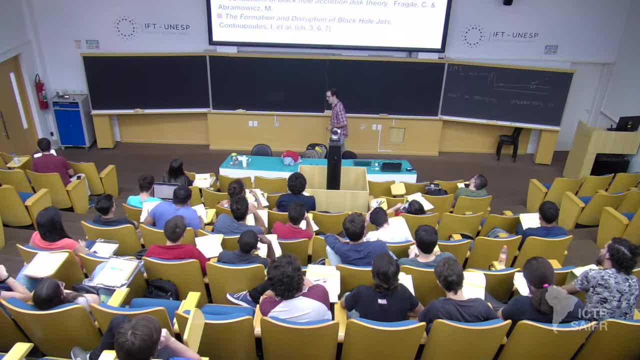 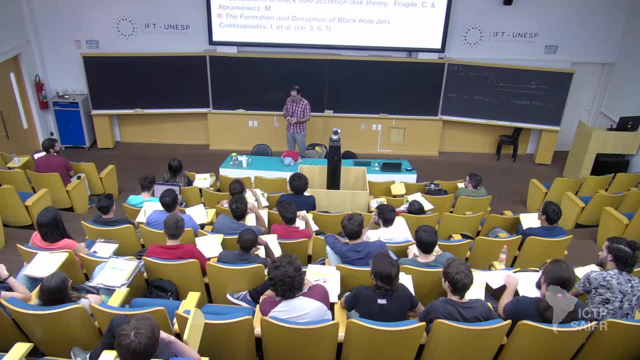 talking about these topics. Fabio, do I have like one hour? You have one hour and 15 minutes for the class. Okay, This thing is going to produce an annoying sound. Oh, really Great. Okay, I'm going to put the timer myself here. 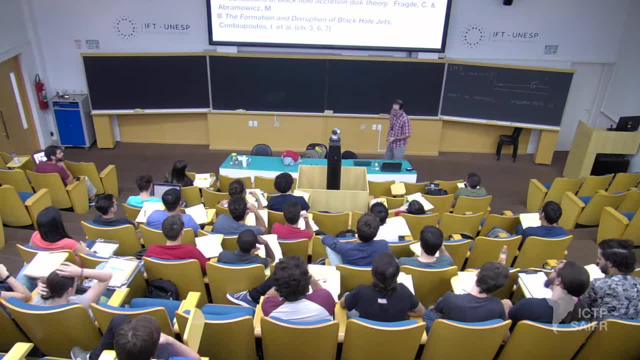 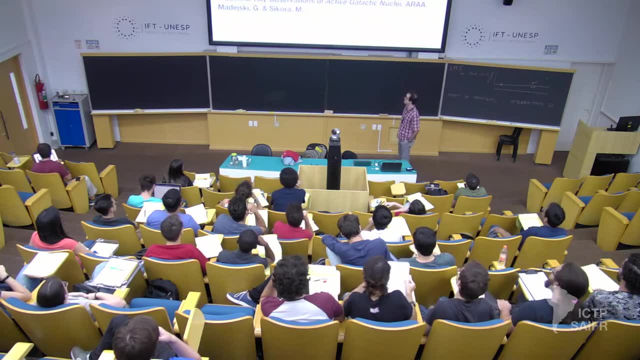 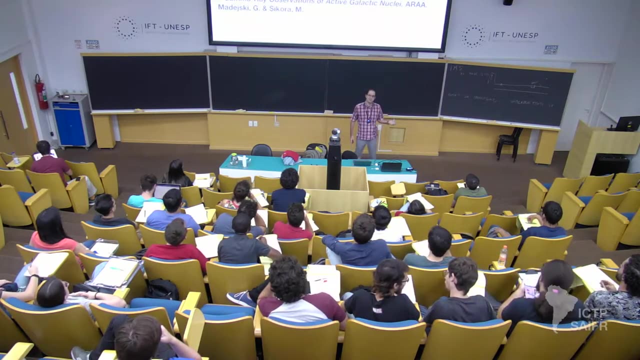 Cool, Awesome, All right. So these are some suggestions of references for theory And if you want some references for the observations, observational overview, well, at least from the electromagnetic point of view, okay, of AGNs, But also a bit of cosmic rays. 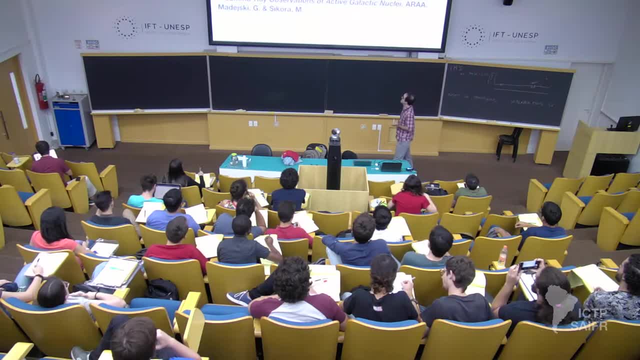 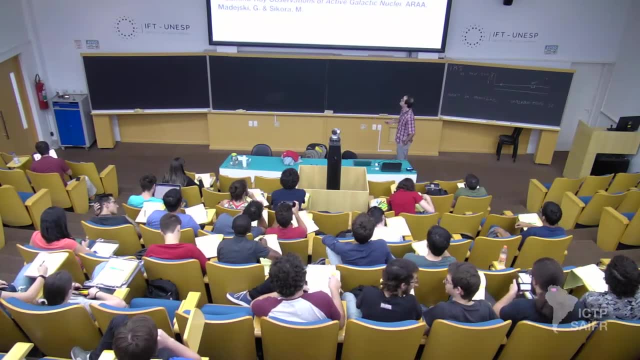 I'm not so sure about neutrinos. in this case It's basically a new field, Observing neutrinos from lasers basically. But there is this book by Volker Beckmann and Chris Schrader: Active Galactic Nuclei. It's a very nice book. 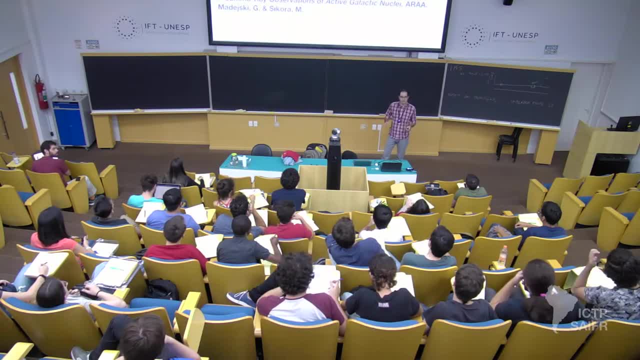 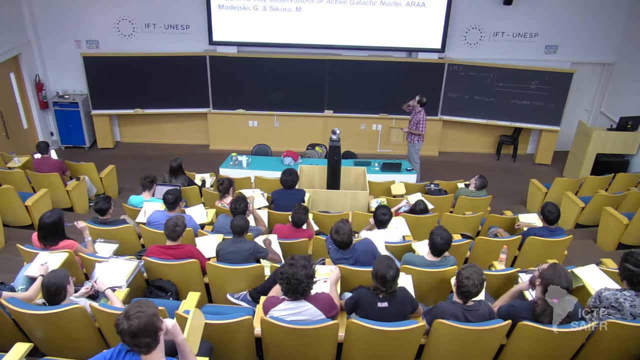 We'll give you an updated understanding of the observations of AGNs. And then I also suggest these review papers. The first one is Low Energies. It will teach you about unification of AGNs- Relativistic Jets- a very broader review paper. 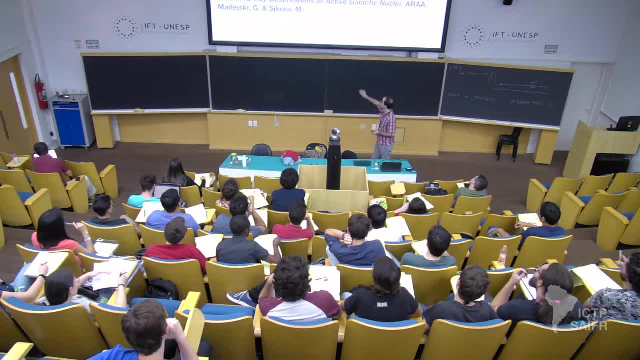 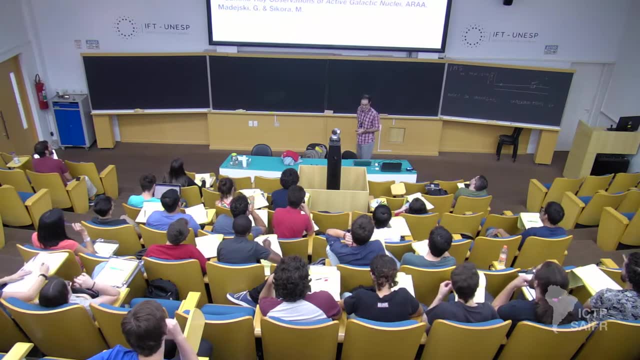 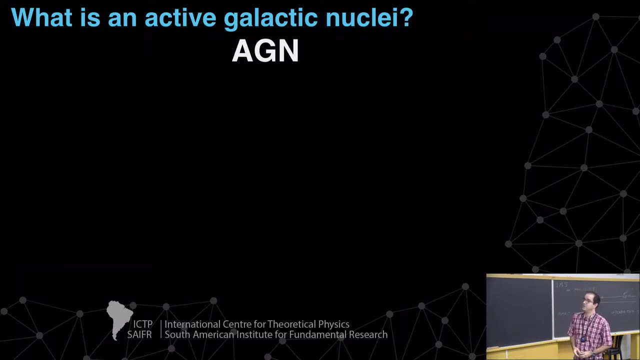 A very broader review by Roger Blanford again, And then the review by Madeschke and Sikora for gamma ray. Gamma ray observations of AGNs, mostly blazers. So let's begin here with the first question that we need to address. 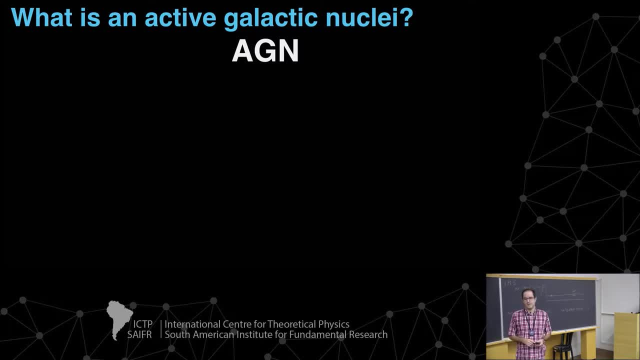 What is an AGN? So let me have an idea here. If I asked you, If we did now an interview outside this room and I call each of you and we'll give you some financial reward, let's say, Maybe, I don't know. 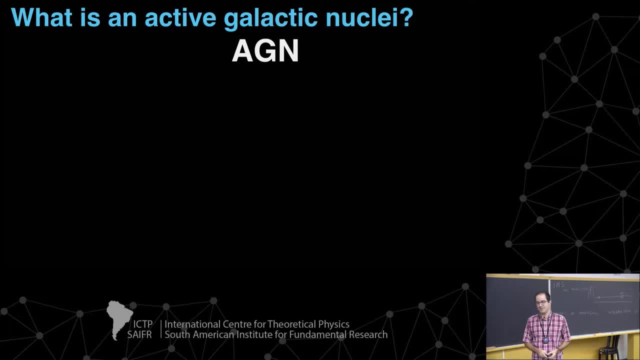 Or some candy. I don't know How many of you would know how to define an AGN, Could explain to somebody. It could explain to a graduate student what is an AGN. Can you Well, can you, raise your hands? 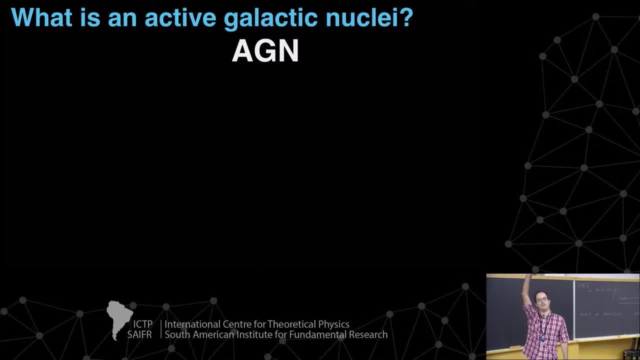 Who would know how to define an AGN. I think we are suffering in this audience. We are suffering in this audience for something that psychologists they have a name for: this Pluralistic ignorance Where you think everybody knows and you are the only know that doesn't know a topic. 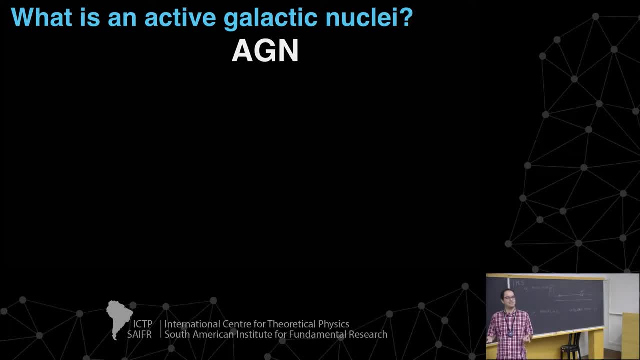 when in fact nobody knows very well, but you are too shy to admit. You know there is Psychologists. they know very well this kind of dynamics. We can talk more about this after the lecture. Don't worry, I'm sure some of you, at least two of you. 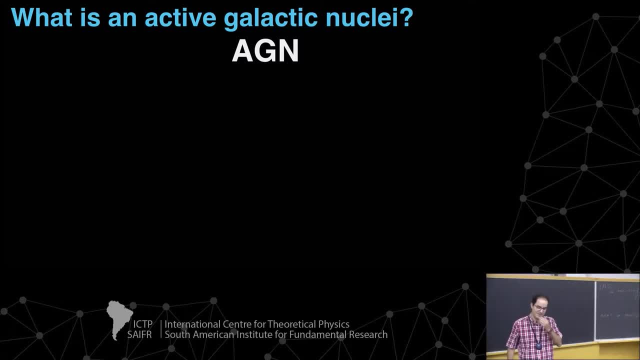 know what an AGN is and would know how to define an AGN. So my working hypothesis here is that I will assume that you know very little or you never heard about an AGN. Well, you heard, but you don't really know how to. 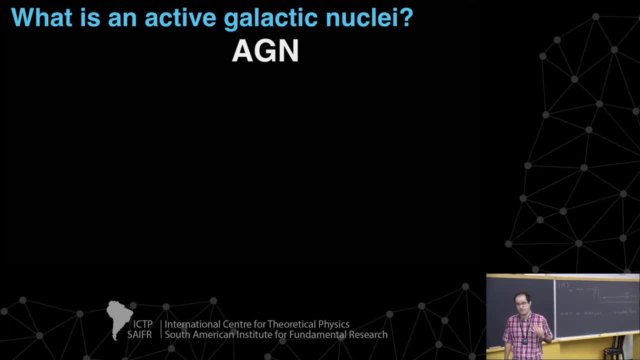 explain to a fellow grad student what an AGN is. Okay, So this will be my hypothesis here for these lectures, given the lack of reply. But I was shy as well. when I was a graduate student I was. I started grad school very shy and I ended. 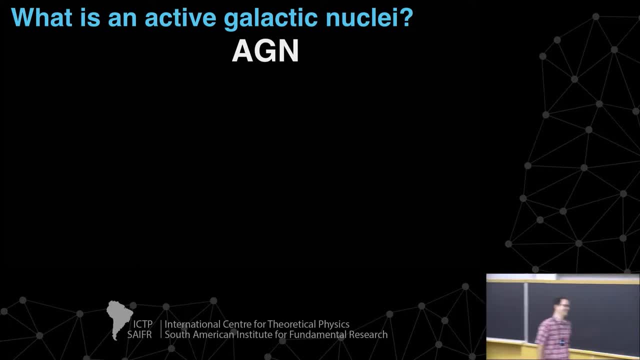 I don't know, I ended like this, dancing in public. No, I'm kidding, It was not so. That did not escalate so quickly, okay, So okay, let's What is an AGN? Okay, so we have three words here. 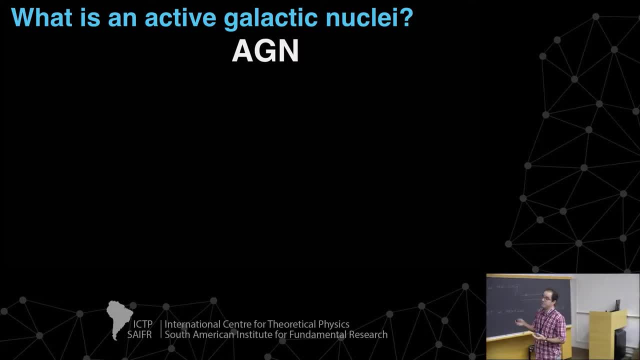 Active Galactic Nuclei, abbreviation AGN. Let's begin with the Galactic Nuclei part. okay, So Galactic Nuclei are the central, the very central regions of galaxies. When I am talking about Galactic Nuclei, I have in my mind a spherical cow region. 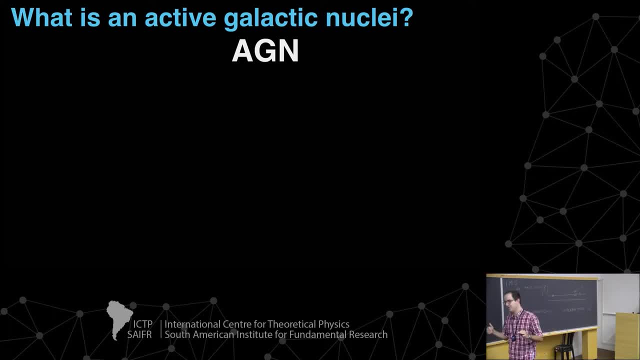 the central region of the galaxy with a radius smaller than about 10 parsecs. okay, 10, more or less 10 parsecs. One parsec is about three light years, If you ask me to tell you how much a parsec is in meters. 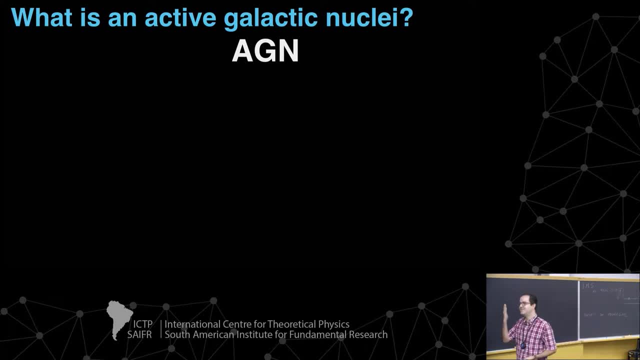 I will not know what to tell you. Probably 10 to the 11 meters To the 18, man To the 18, see, Wow, Okay. 10 to the 18, okay, See, because my mind is tuned to work in parsecs, okay. 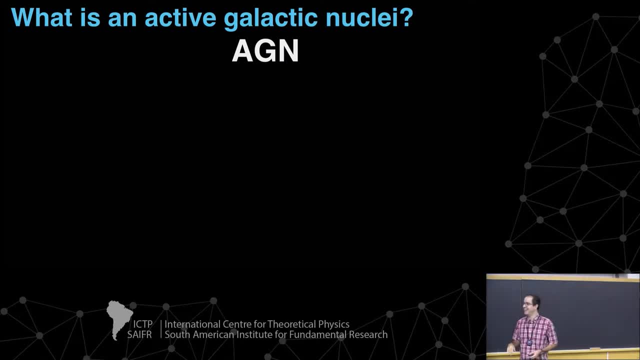 So I don't care about meters. I don't care about meters anymore. Tell them how to convert. Parsec is three light years. That's easy to remember. Yeah, that's easy to remember. okay, 10 to the 10 by 10 to the 10.. 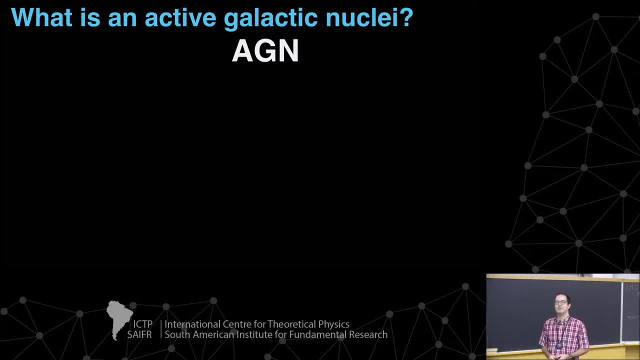 10 centimeters per second. Thank you Right, We will be. we will have our. we will have our eternal gratitude to you, professor. Thank you, Okay, 10 to the 18 meters, one parsec great. 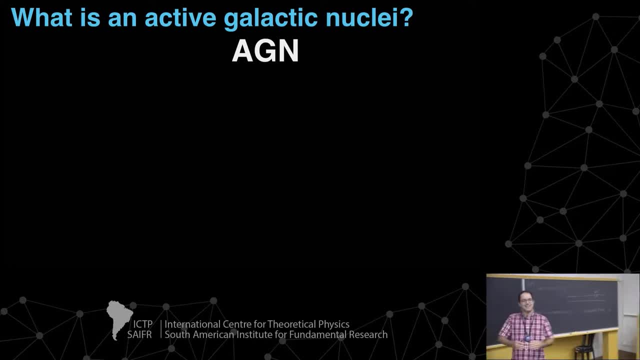 Centimeters, Centimeters, okay. Anyway, it's a huge distance for human scales, So, okay. so this is what I just told you is what I have in mind when I think about what is a galactic nuclei- okay, The very central core regions of a galaxy. 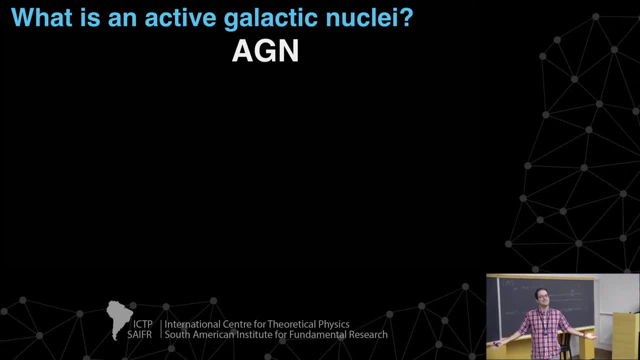 and galaxies, as you know, are cosmic islands. okay, So this is so. we covered the words number two and number three here, and now let's cover the word number one: active. okay, What does an astronomer mean when they say that the galactic nuclei are active? 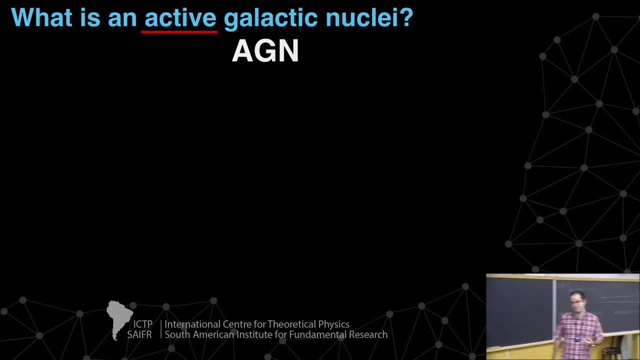 Is active. And then I have a. well, it will be a rhetorical question, given the lack of participation, but do think in your minds and run a simulation in your minds. Is the Milky Way, an active galaxy, The cosmic island that we inhabit? 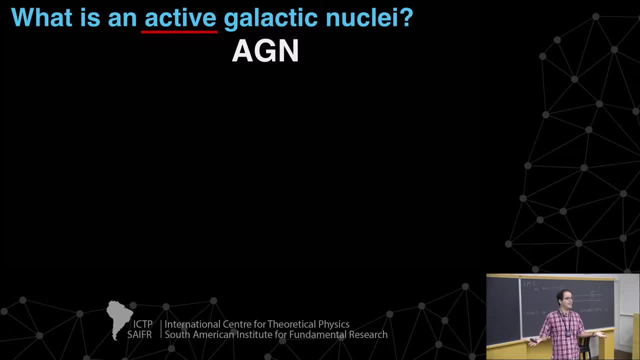 is it an active galaxy? Well, we are still alive here, so it's not an active galaxy. Okay, so what is active? What does activate the nucleus of a galaxy? okay, So what activates the nucleus of a galaxy is the presence of a super. first of all, 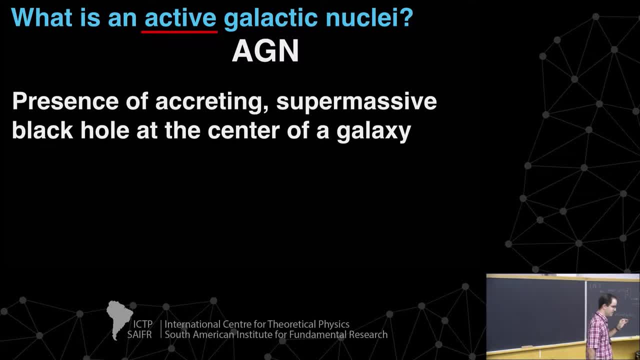 you need a supermassive black hole there, sitting near the center of mass of the galaxy. That's not a problem. The universe somehow manages to put one supermassive black hole, or more than one supermassive black hole, at the centers of evolved galaxies. 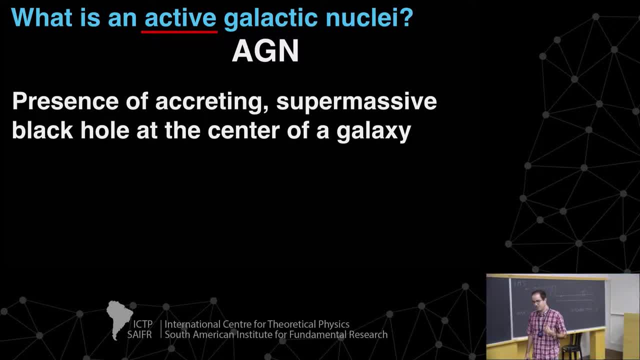 This is a topic of a lot of study. you know the formation of the seeds of supermassive black holes, But okay, so most galaxies evolved galaxies. they have supermassive black holes at their centers. So what activates is the fact that you. 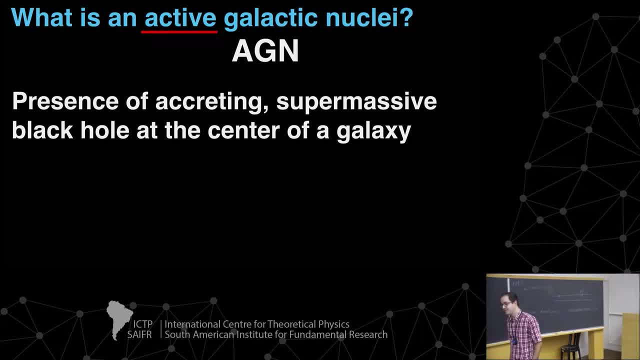 the galaxy is somehow providing vast amounts of gas particles to the black hole, providing the space-time of the black hole with huge amounts of test particles. okay, And it turns out that black holes have a lot of free energy. okay, And so nature manages to use these test particles. 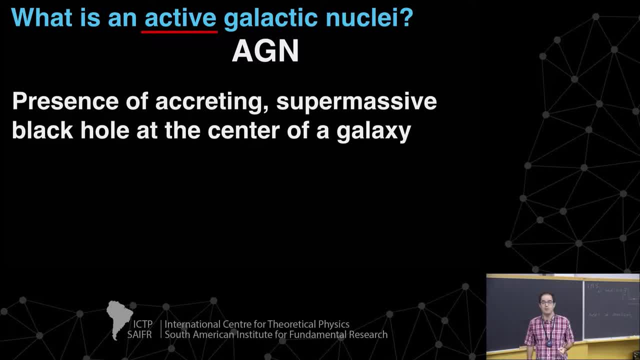 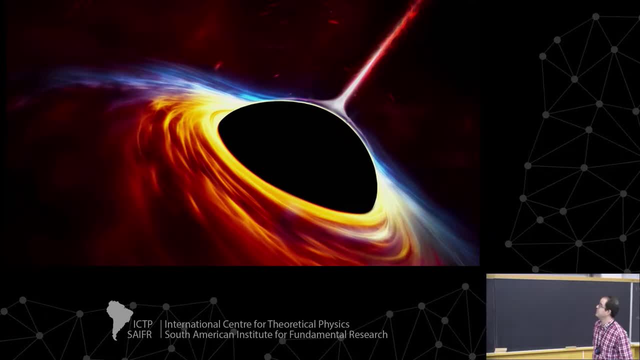 to extract the free energy from the space-time of the central supermassive black hole. okay, This is what activates a galaxy. So here is what we have in mind. So this is a cartoon version. this is not a numerical simulation of a supermassive black hole. 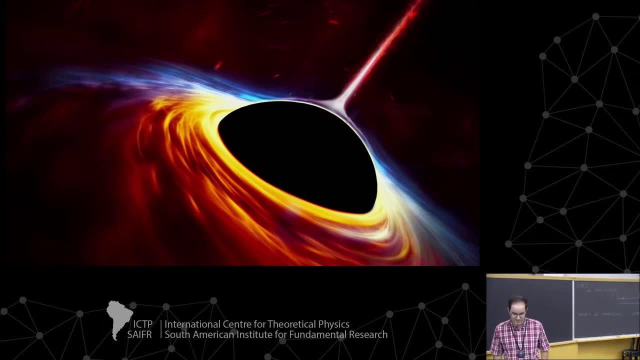 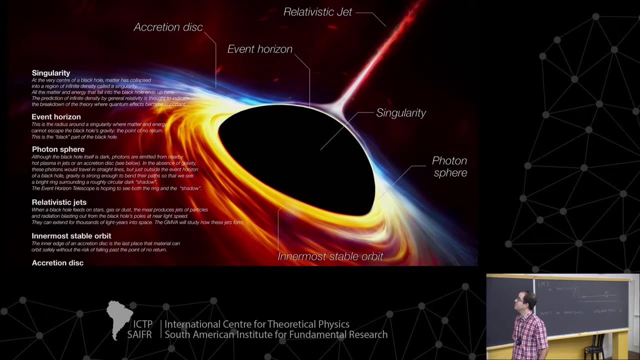 You have here trillions of particles, ionized particles, swirling in the accretion disk, around in the accretion disk, around a supermassive black hole. These are the relevant ingredients of the central engine of AGNs. So, of course, the event horizon. 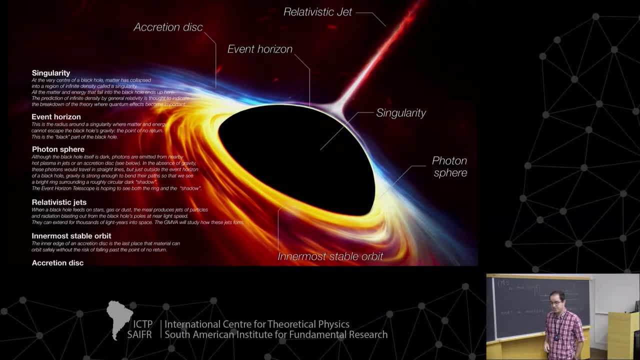 Inside the event horizon, there is this mysterious point, the central singularity, which has all the mass of the black hole concentrated in the central singularity, the realm of quantum gravity. We do not have equations to treat the central singularity. What else? 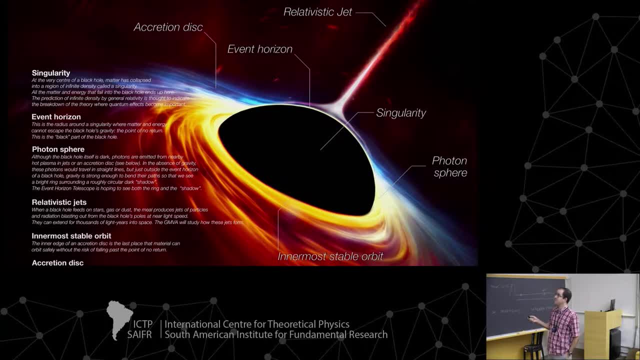 So here, as I mentioned the accretion disk, There is an important concept which this cartoon gets right as long as this: if this black hole is maximally spinning, then the cartoon is correct: The innermost stable circular orbit. if this was a Schwarzschild black hole, 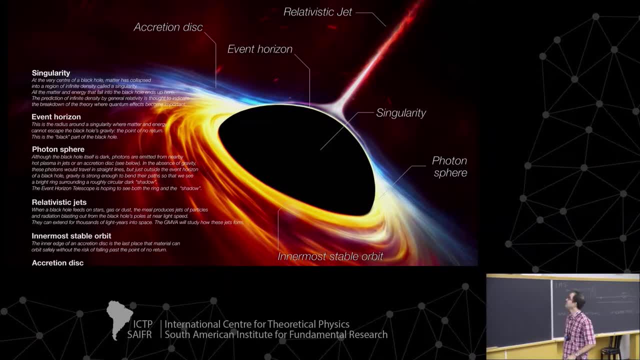 the depiction of the innermost stable orbit will be wrong. And the photon sphere, which I will also describe very, very soon in the lectures. So these are the important ingredients, as well as the relativistic jet which produces high-energy radiation. 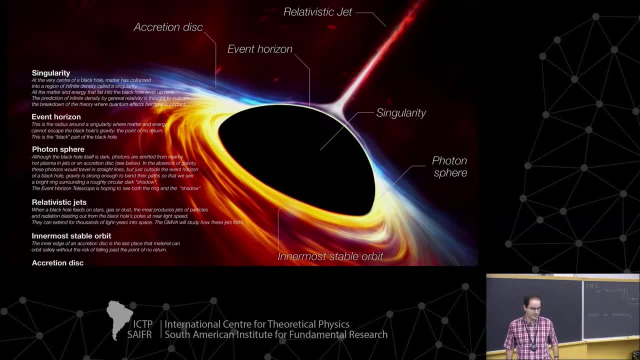 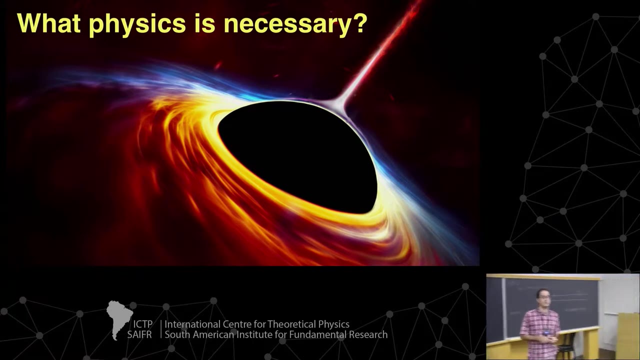 high-energy particles that we love to observe here and spend hundreds of millions of dollars building space missions and ground-based telescopes to observe these particles. So what is the physics necessary to understand to properly model and describe these objects? So, first of all, generally, 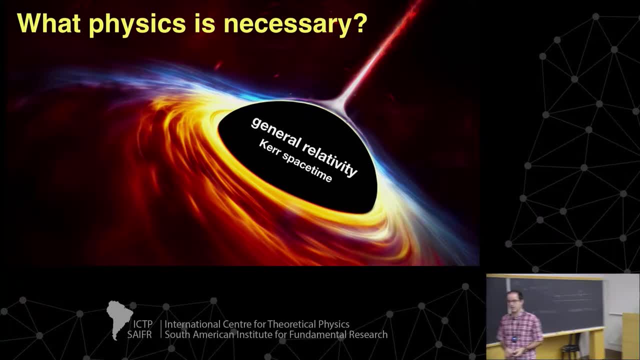 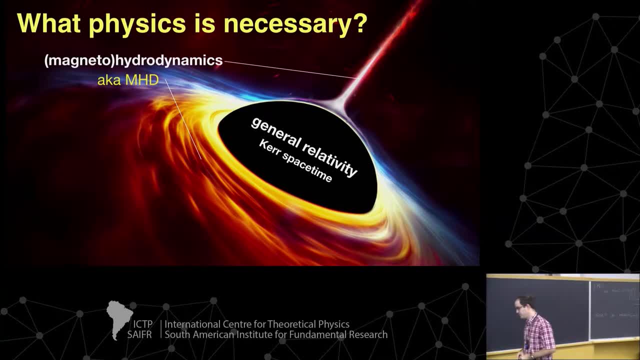 you need to combine the conservation equations of fluid, of charged fluids, magnetohydrodynamics, MHD and with general relativity. So the name we give to the resulting set of equations, the covariant version of the conservation equations for a charged fluid. 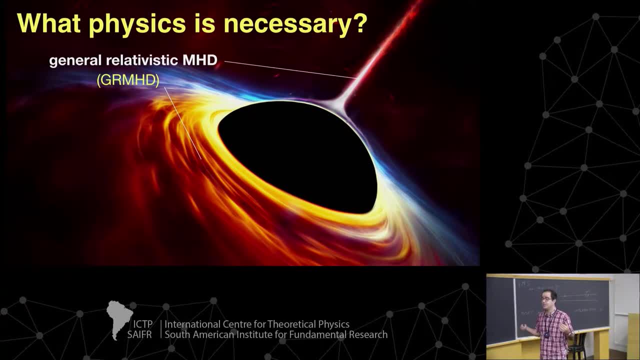 we call it general, relativistic MHD, GRMHD. There is a catch, however. I don't know if Blasi is not here. The two Pasquales are not here in this lecture room right now. Okay, okay, Pasquale squared. 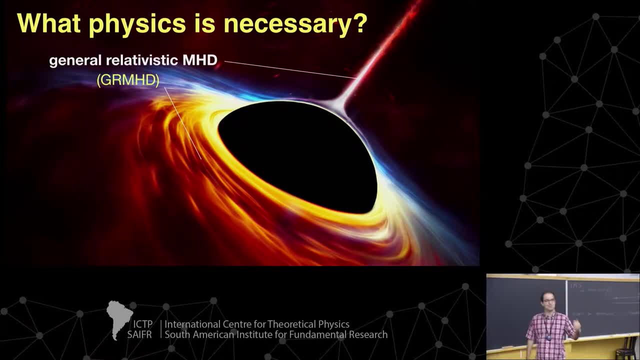 You were. you got Pasquale squared in the school. Okay, There are two, at least two Rodrigues in this lecture room. by the way, How many Rodrigues are here? More or less you. no, you are a Rodrigue. 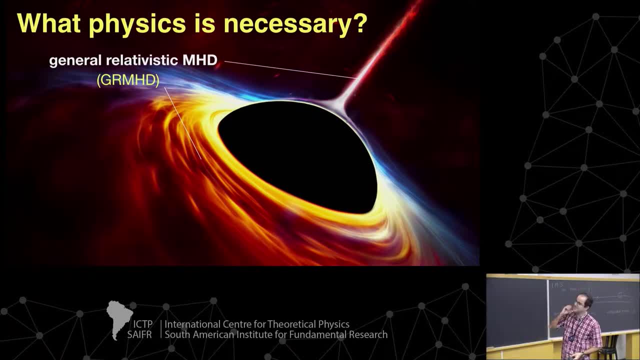 Just two Rodrigues here, okay, Right. so because in many cases, in many of the systems of interest, the plasma density is very low, you get into the so-called collisionless regime of plasma physics, and then the MHD approximation is not necessarily a good approximation anymore. 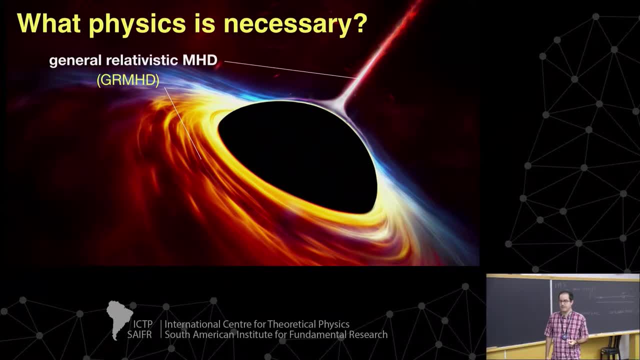 Okay, You need to to do kinetic theory, which you have been solving- Vlasov's equation, I heard. right, Right, Okay, okay, So you are dealing with some kinetic theory here. So it turns out that for some of the, for instance, 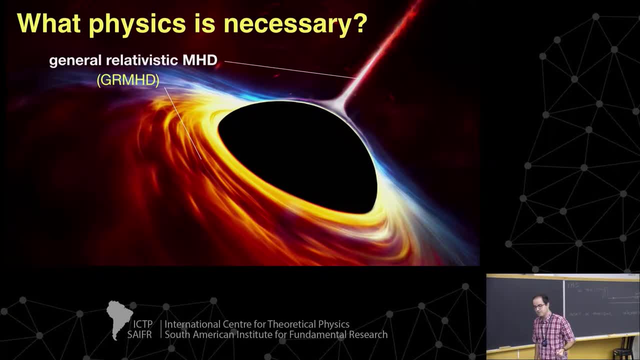 the black hole at the center of the M87 galaxy, which was imaged three months ago, more or less four months ago. you need to- you actually need to do kinetic theory to properly describe the flow around the black hole, And it turns out that we do not really have a good general relativistic kinetic theory. 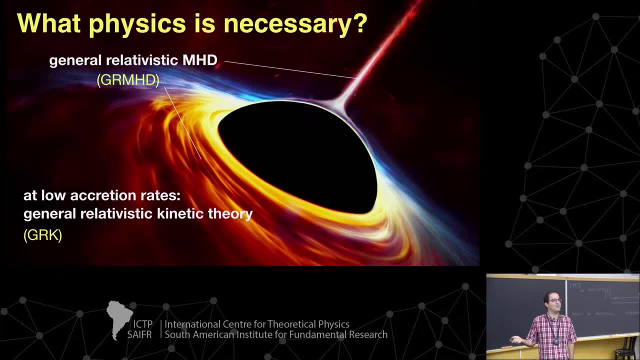 which I will call GRK, but nobody. there is basically no acceptable code that does general relativistic kinetic theory. Okay, so nobody felt the need to create an acronym GRK because there are not a lot of people working on this Right. 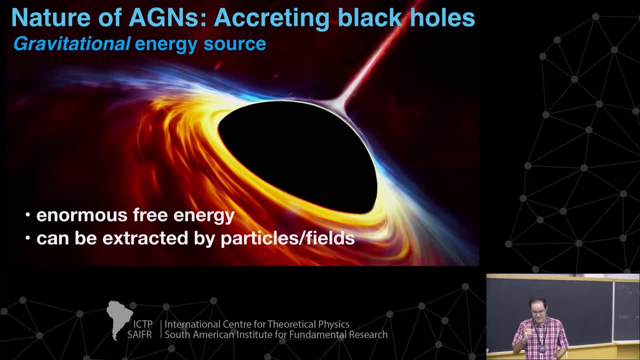 So so the nature, it is really central, literally central to the concept of AGNs, that you have a creating black holes and the source of the huge amounts of energy we observe with our telescopes is the electromagnetic energy, for instance. 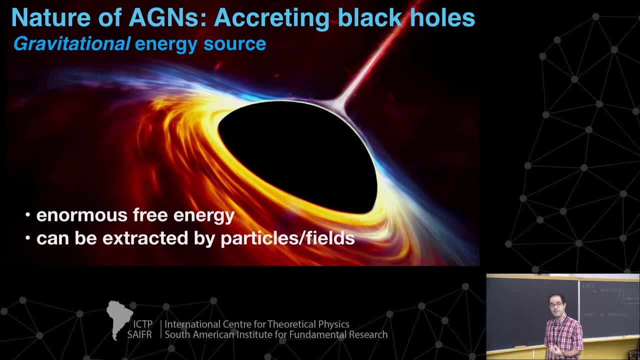 The source of this energy has a gravitational nature. Everything is coming from gravitational potential energy of the black hole And, as I mentioned to you, somehow nature is using particles and fields to extract this free energy from the space-time and bring some of it here to our planet, planet Earth. 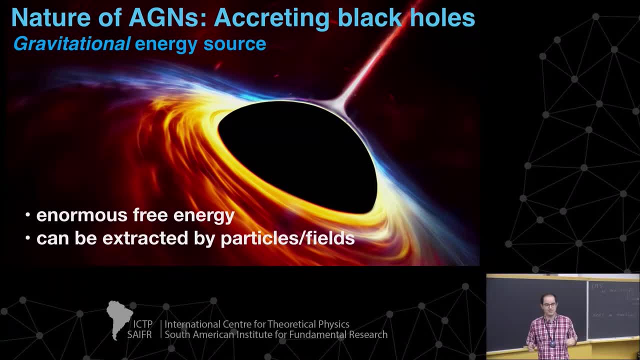 Okay, so now we have a very qualitative idea of what is an AGN. We know that black holes are very important. We know that if you want to understand physically the observations, you need to have some ideas of general relativity. So now let's talk about the challenges. okay. 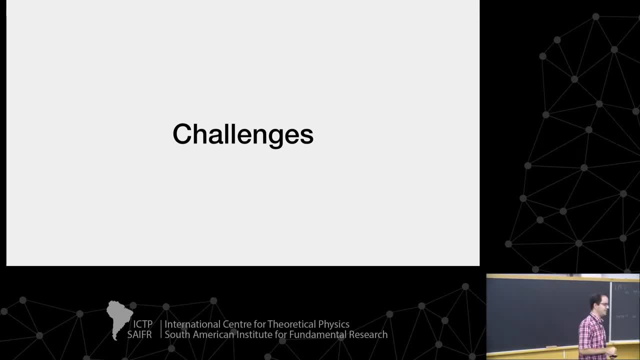 What are the challenges behind observing these systems? What are the? what are the big challenges There are? I will. there are several challenges, but I will point three, specifically three challenges, if you want to observe these systems and try to use your equations to model the observations. 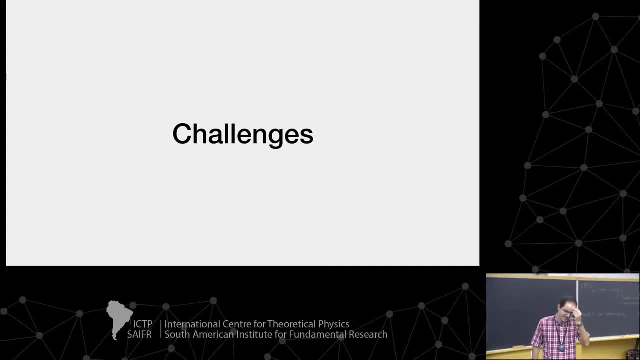 The first challenge is very. I have a story to tell. I will tell you about the first challenge. Have you heard of the tale of the blind man? There were, there were a couple of blind men or blind women or blind robots, and there was an elephant. 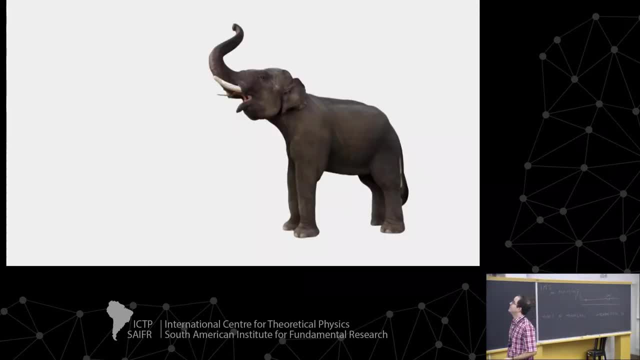 Here there was an elephant, okay. So I think this is a Chinese tale. I don't remember if this is. if this is a Chinese, I think it is Chinese tale And the blind men were asked by the king to go there without seeing. 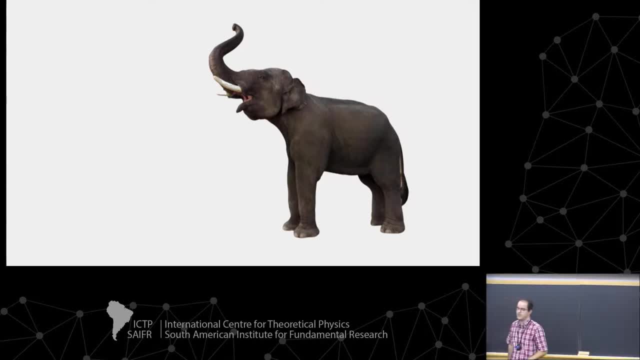 and then touch this creature, this strange creature, and tell the king: bring back, touch one part of the elephant and go back to the, to the king or the emperor, and tell the emperor what they saw, or what they saw with their other senses. okay, 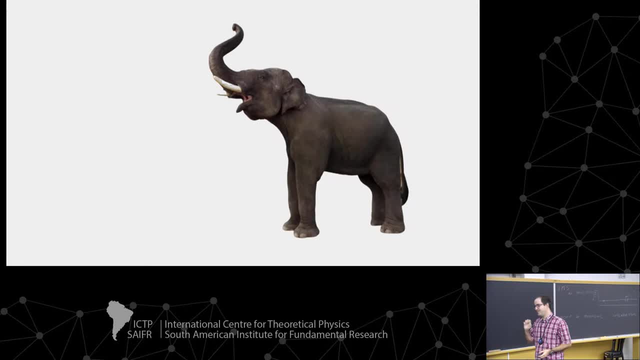 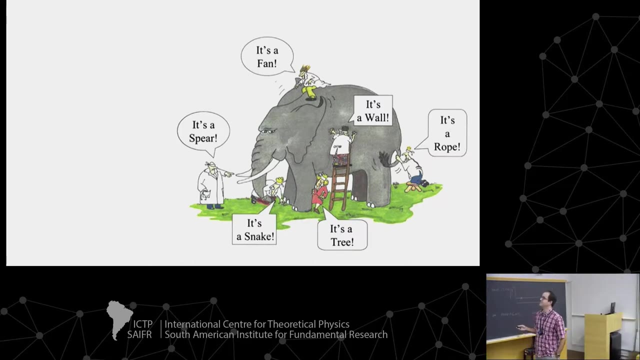 And it turns out that if they have, if they only have access to one part of the elephant, they will get very different pictures, very partial pictures of what they are feeling. okay, And so, as the tale goes, one of the one of the scientists, 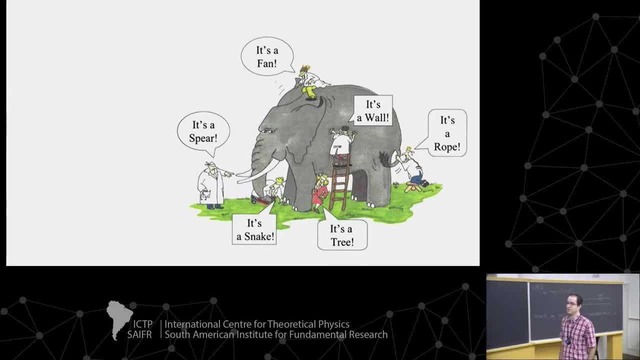 one of the blind scientists touched this part of the elephant. Oh, it's a spear, okay, This one. I don't know what, what he or she is touching there, but he's saying it's a snake, Okay, strange. 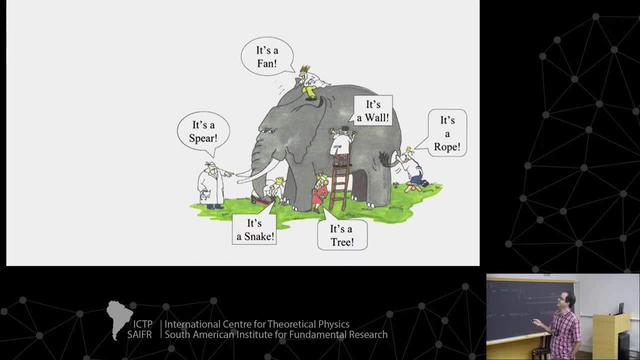 It's a tree: okay, It's a tree. It's a spear: okay, It looks like a tree. No, looks. it's a blind person. It's a fan. It's a wall. It's a rope- okay. 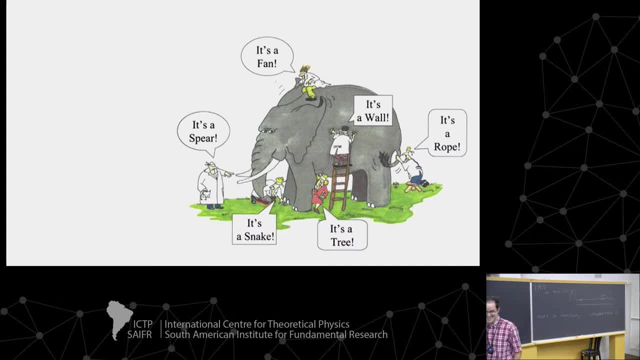 I hope he doesn't stay there for too long- the person with the rope. And it turns out that this is a great analogy to understand the, a great analogy to understand the first challenge behind characterizing AGNs in astronomy. okay, The thing is that AGNs 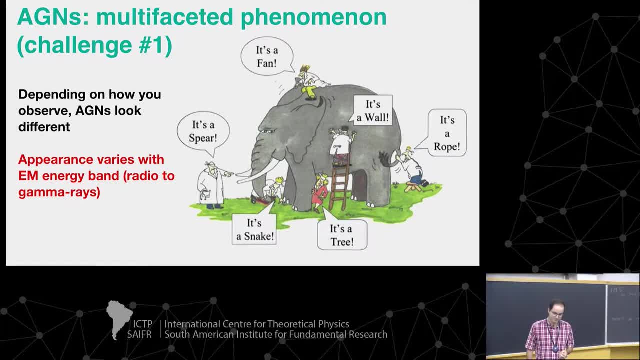 they are a multifaceted phenomenon in the sense that they are our cosmic elephant. Depending on how you observe an AGN, you will see very different things Concretely, depending on what, what energy band you are using in the electromagnetic spectrum. 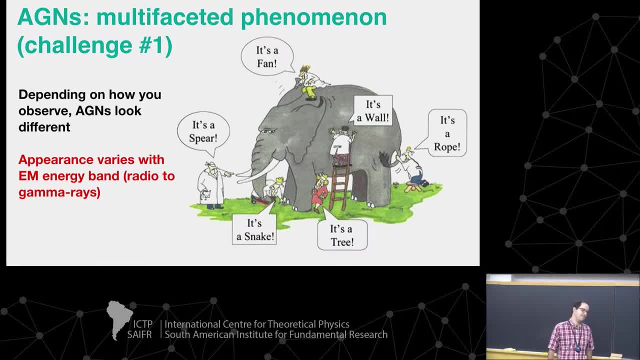 you will see very different things, okay, And because science evolved in this chaotic, nonlinear way, we we did. you know, astronomy was not born with access to all wavelengths, okay, So we were seeing particular parts of the picture, And so this, this did not help putting together. 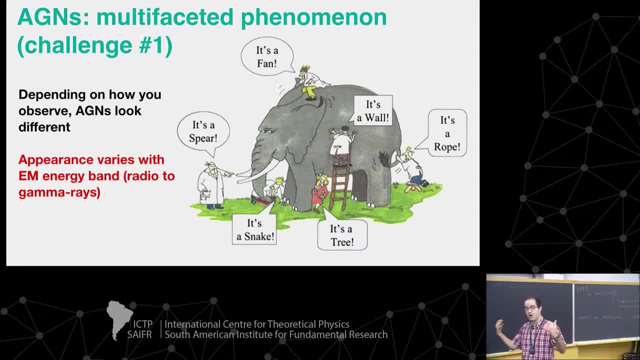 a concise picture of AGNs. It took us a long time to put, to have a narrative, a scientific narrative, for the origin of AGNs. So this is basically what happened in the AGN field. okay, Oh, radio jet- compact radio emitters. 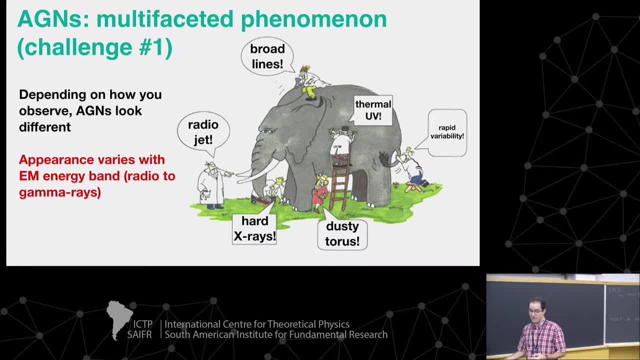 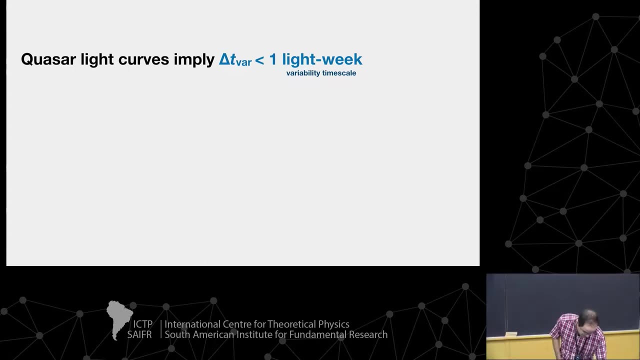 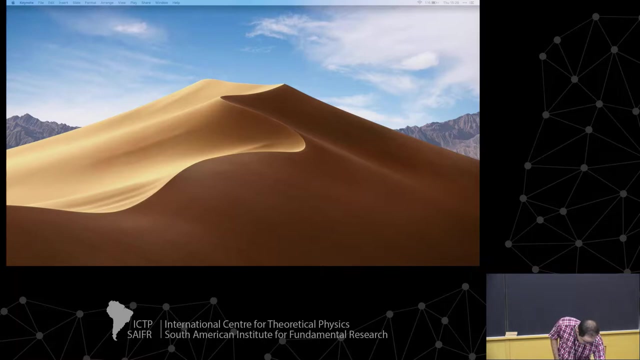 Compact radio emission broad lines, Oh, not broad lines- Hard x-rays, those two towers. So this is the cosmic version of the blind elephant tail. The second challenge. here is the second challenge. here is the following. The second challenge started. 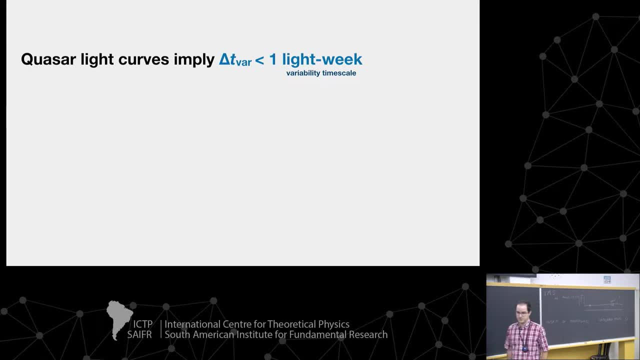 many decades ago, when astronomers were monitoring the variation of AGNs, They started monitoring the time series of flux variations of quasars. We call quasar light curves, And the interesting thing here is that they were seeing that there was a coherent variability in the time series. 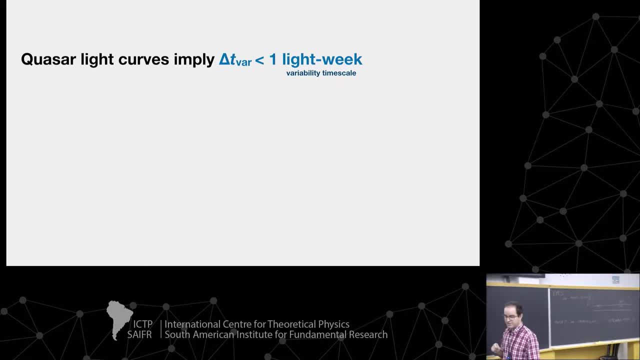 with variability time scales smaller than one week, okay. They would see a quasar bursting in one week and then fading, or in less than a week, okay. And I realized that I made a little error here. It should be week there. 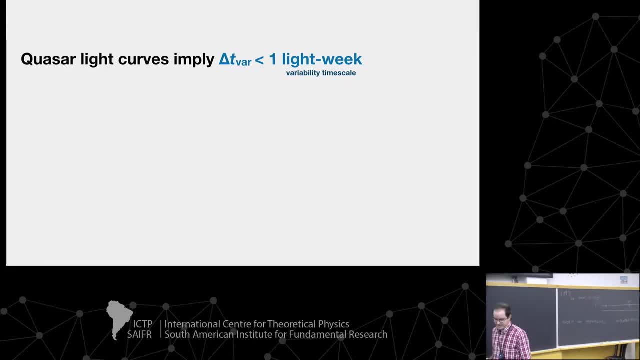 So variability, time scales of less than a week. And when the astronomers went to talk with the theorists- okay, I know, I have the time series of variation of quasars- What is powering these quasars? They didn't know what was powering. 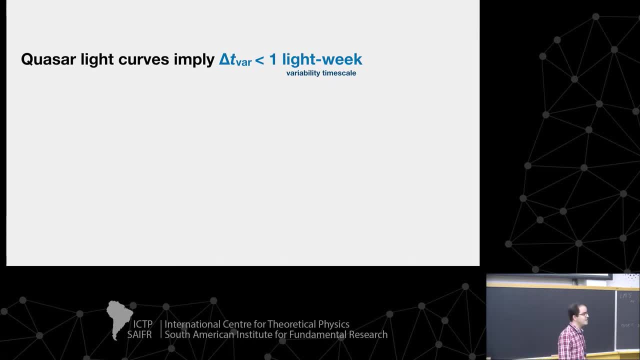 They didn't know it was supermassive black holes powering quasars. But they had this very interesting like time series. They went to the theorists And the theorists. they told the theorists, told the observers that okay, if you have something varying coherently, 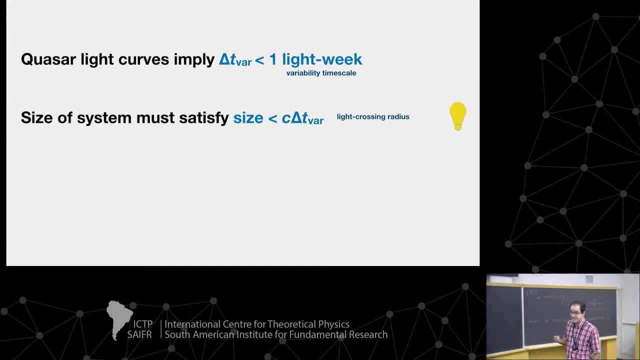 with time scales less than one week, let's say. this implies that the size of the system must satisfy the relationship. There is an upper limit to the size of the system which is less than the speed of light times, the variability time scale. The size is less than one light week. okay. 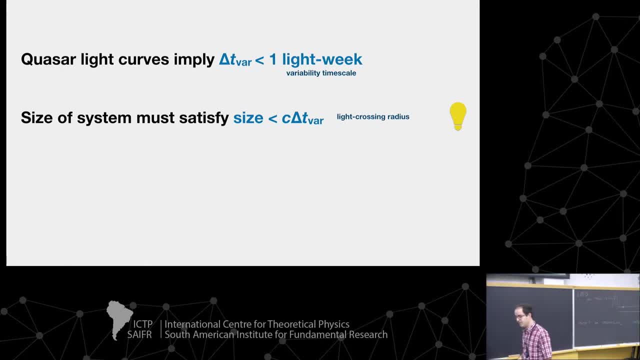 Which is the light crossing radius associated with the variability time scale. Why is that? Why is that So? it turns out that it's quite difficult to build any sort of a plausible model of a luminous astrophysical object that varies strongly on a time scale. 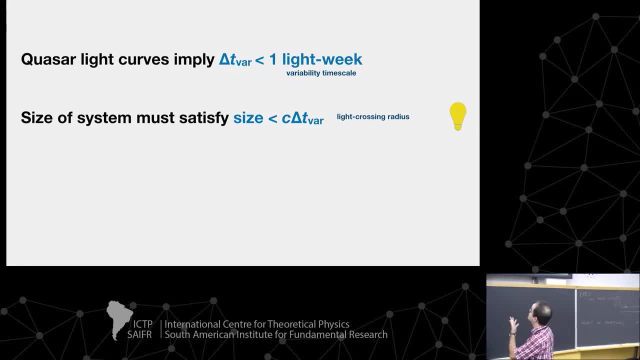 smaller than the light crossing radius. okay, It's extremely difficult to try to build a model to explain such kinds of coherent variabilities with sizes that are bigger than this. okay, And the reason is that the separate parts of the object, if they are separated by sizes bigger than. 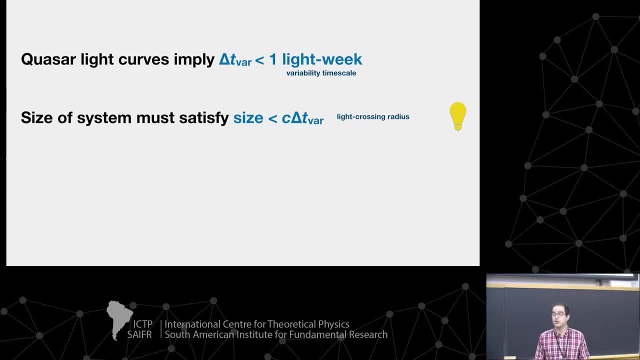 this size scale here, they would not be causally connected on that time scale of one week. okay, So this gives you a very nice idea that something is powering quasars and it's very compact. okay, So if we translate this to more familiar units, 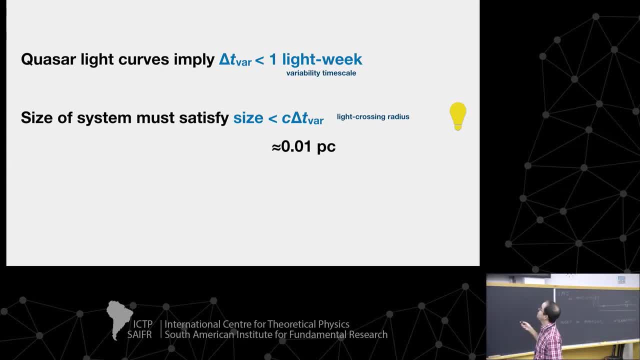 at least to astronomers. this implies that an upper limit to the size of a quasar, the thing powering a quasar, is less than 0.01 parsec. okay, And the parsec units that astronomers love, So a few hundreds of a parsec. 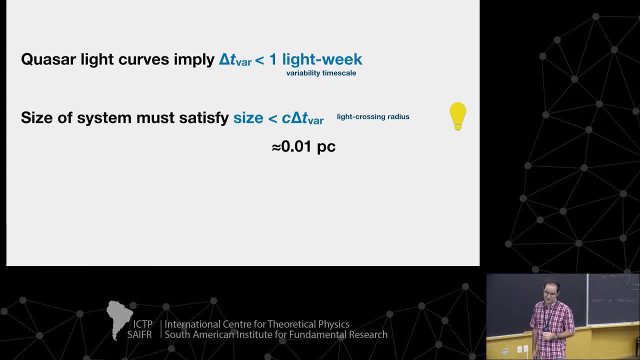 might look large by our human standards- okay, But this is extremely tiny compared to galactic scales. okay, This is extremely embarrassingly small. okay for galactic scales, It's a millionth of a size of a galaxy. this land scale. 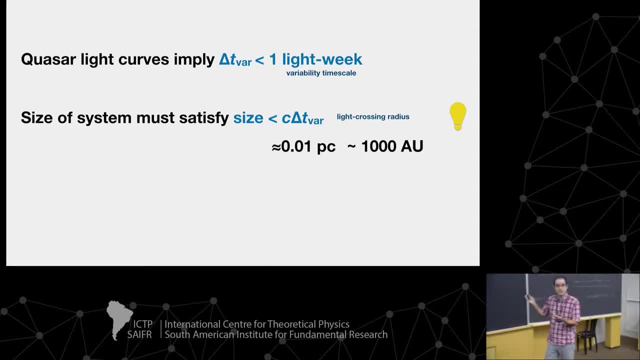 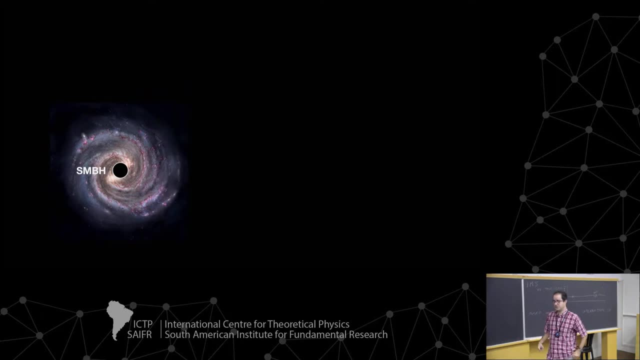 which is about a thousand astronomical units. okay, So one astronomical unit is the distance, the average distance between the sun and our planet. So this is a challenge. this is a big challenge. Why is this a challenge? Because this taught us. 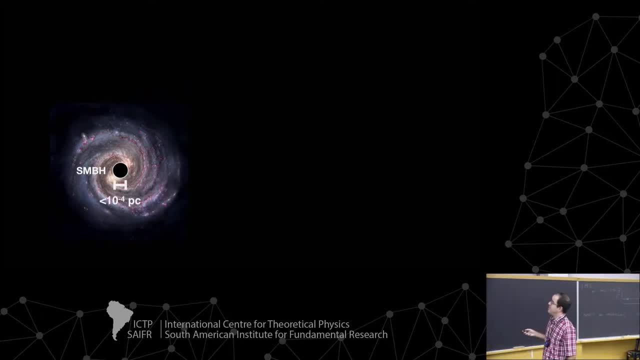 this taught the astronomers that if you compare the size of the sphere of influence of the black hole- which I will give here a rough figure- 10 to the minus 4 parsecs, okay- And you compare that to the typical optical, the typical size of emitting, 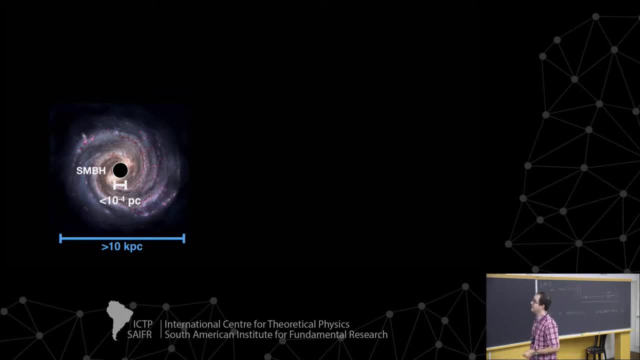 the observed size of galaxies, not taking into account the dark matter halos. there is a huge difference between the size of the black holes and the size of the galaxy. The black holes are extremely small compared to the host galaxy. How small? Well, you can do the calculation here. 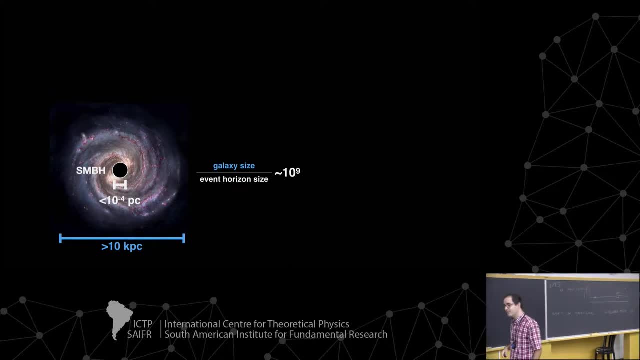 If you do the ratio between the galaxy size and the event horizon size, this ratio is one billion, which is, coincidentally, very similar to the ratio between the classical radius of an atom and its nucleus. okay, This is a very similar ratio between the ratio between the size of a galaxy. 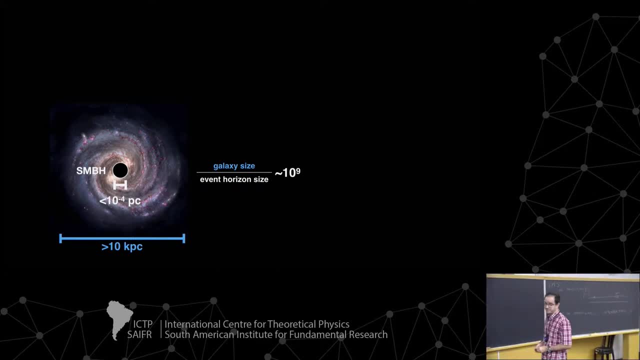 and the event horizon radius, And also there is another analogy here, just for you to have an idea of the asymmetry of scales that we are talking about. If this galaxy was planet Earth, the black hole would be a grapefruit here in this room. 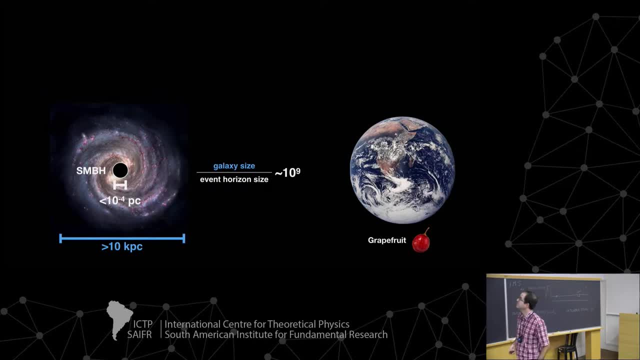 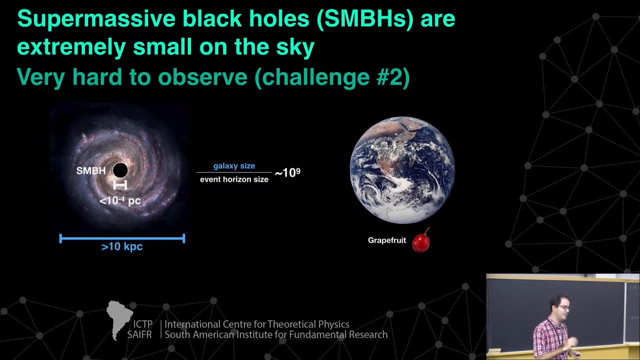 Okay, does anybody have a grapefruit here? No, I don't think so. So this leads us to the second challenge in observing AGN. Supermassive black holes are very they appear very small in the sky and therefore they are very small. 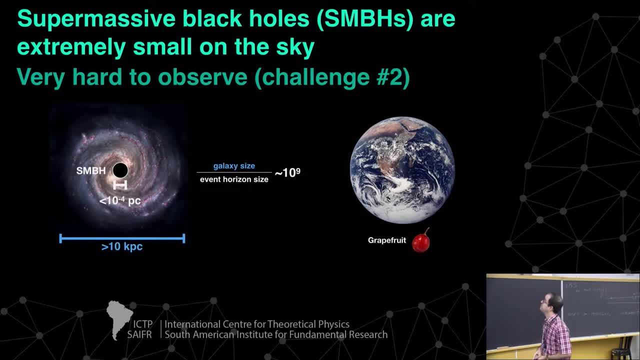 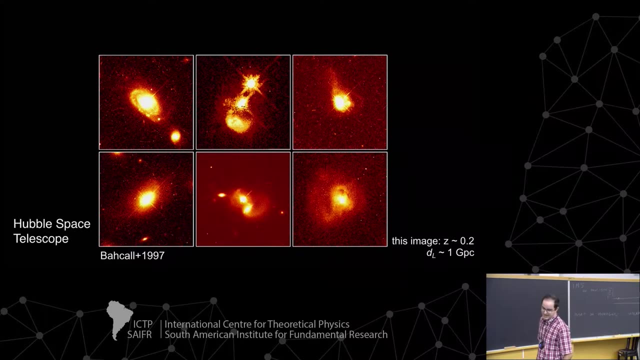 and very hard to observe and characterize, To image. we had to wait a hundred years after Einstein published the field equations to image one event horizon. That's how hard, that's how small they are in the sky. The third challenge is a challenge specific. 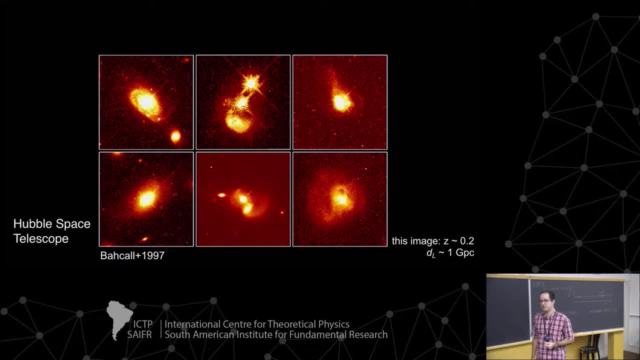 particularly if you are an astronomer and you are trying to characterize the islands in which the supermassive black holes inhabit. So this is one concrete being. concretely speaking, this is a set of six images taken with the Hubble Space Telescope. 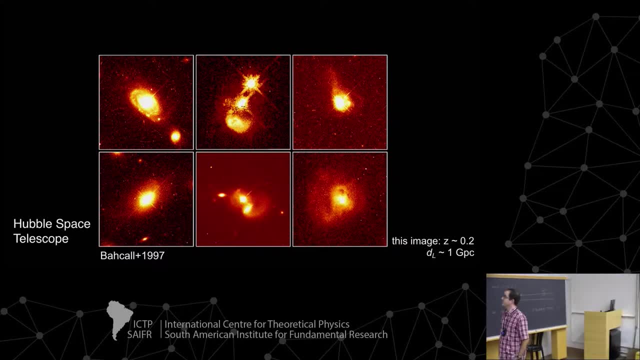 more than 20 years ago actually. This is a very beautiful paper- was one of the was a landmark paper for the studies of quasars. What you are seeing here, what you are seeing, for instance, here you are seeing the image of the host galaxy- 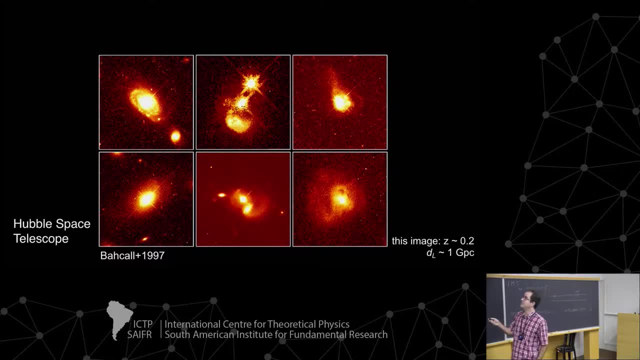 but the problem is, the image of the host galaxy is being outshined by this huge flashlight located at the center of the galaxy, which is the supermassive light emitted by the gas falling onto the accretion disk. And the same thing is happening in all these quasars. 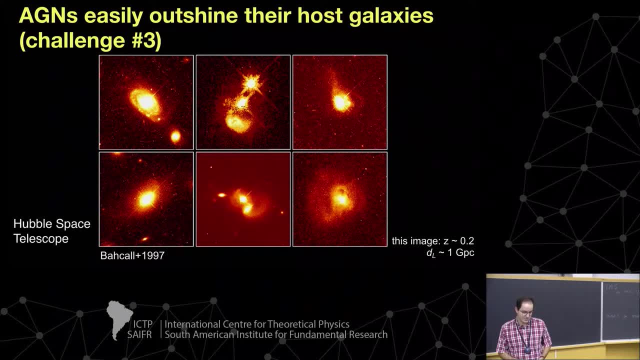 And this leads us to the third challenge. So AGNs: they easily outshine their host galaxies, and so it's very hard to observe what is around. a bright AGN- okay, They are very bright. This is a big challenge as well. 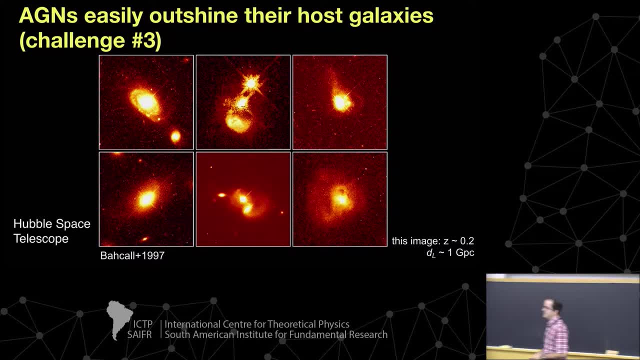 And because we need observations to motivate our theories. we are having trouble getting the observations in many cases, So we will have trouble building theories. This was a huge historical challenge to have a narrative for accreting supermassive black holes Right. so we now know the challenges. 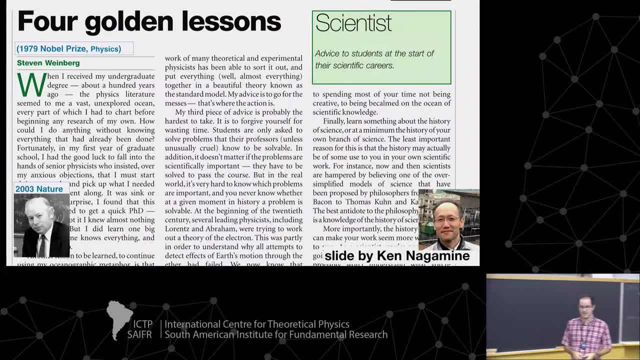 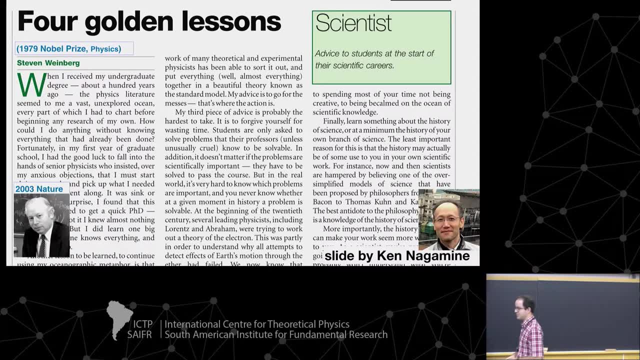 And now that we know the challenges, let's change a little bit gears. now I will do this in this lecture and also in the next lecture. I will do intermissions with things that I think might be interesting to you And I think that every graduate student. 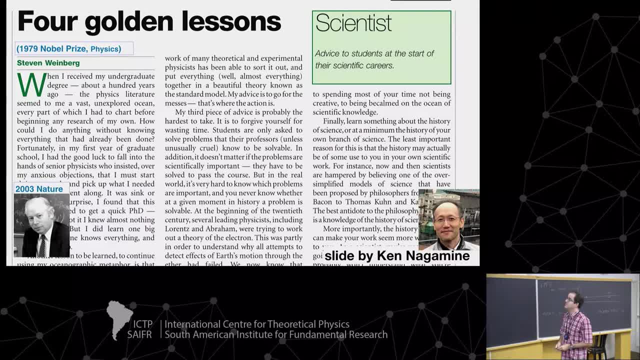 and undergraduate student in physics and astrophysics should read this paper by Steven Weinberg. This article was published. I stole this slide from Kentaro Nagamine. I think Kentaro was lecturing in a school we organized. There is a gentleman sitting there in the back. 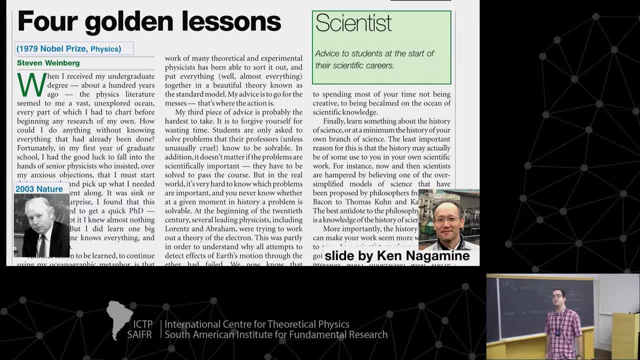 He organized a very nice school on the dark ages of the universe, the re-ionization of the universe, And Kentaro was lecturing And I stole- shamelessly stole- this slide from Kentaro, So I think you should all read this paper. 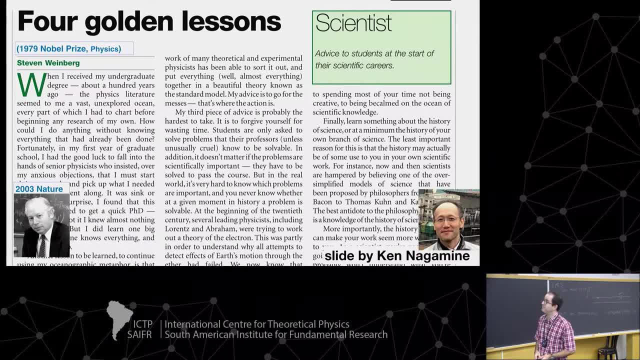 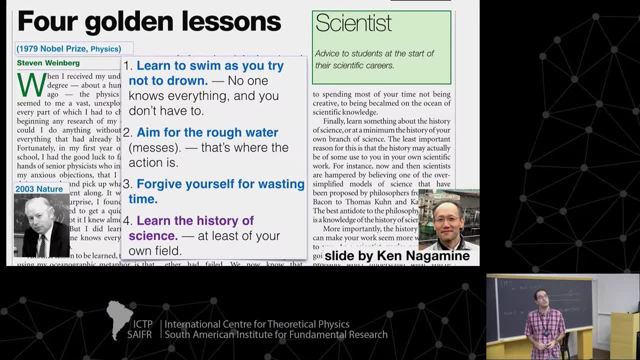 this article by Steven Weinberg, Nobel Prize Physics Nobel Prize from 1979.. Weinberg gives four advices to young science students, young researchers. Lesson number one: learn to swim as you try not to drown. In other words, don't wait to study everything in the field. 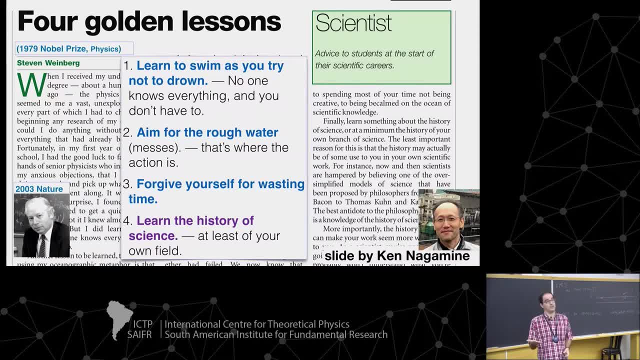 you are working on before you start getting your hands dirty. If you want to learn everything, you will not do anything new. This is especially true in astronomy. Every day there is a new observation. If you wait to study everything, you will not do anything. 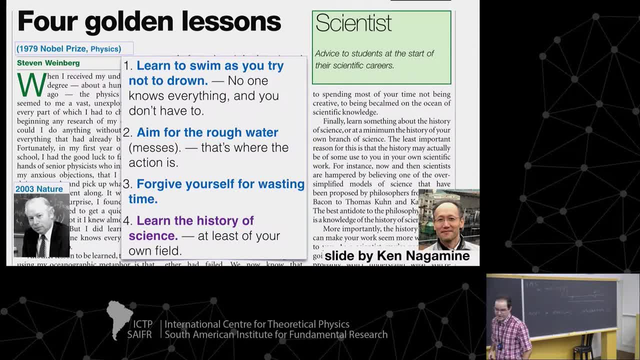 Anything new in science. Number two: aim for the rough water, In other words, try to find where the action is happening in your field. Try to avoid things which are established. You will not get anything new there. Don't go for the boring things. 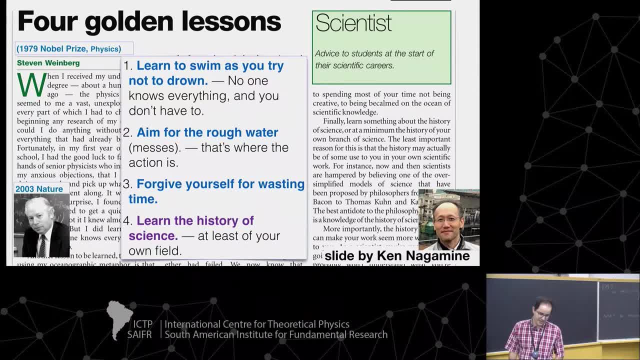 Go for the state of the art. Number three: forgive yourself for wasting time. And number four: learn the history of science, At least the history of science in your field, Because that will give you a perspective of what is happening and what will come. 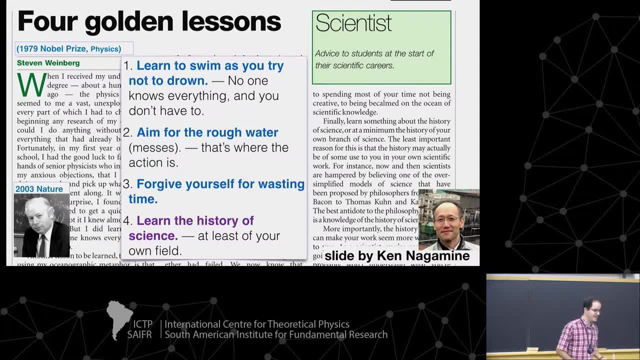 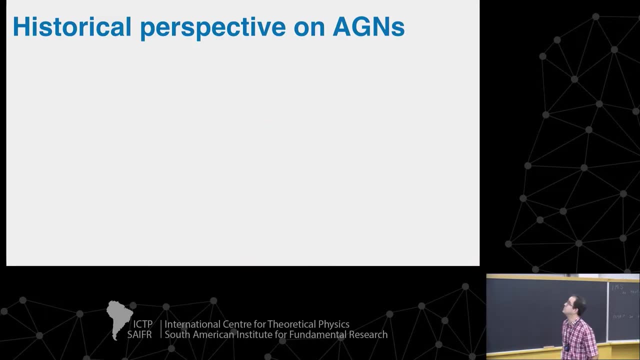 Learning. history is always good, The history of any, particularly the history of science, the history of mankind, humankind. And motivated by point number four that Weinberg is doing here, I would like to give you now a historical perspective on agents. 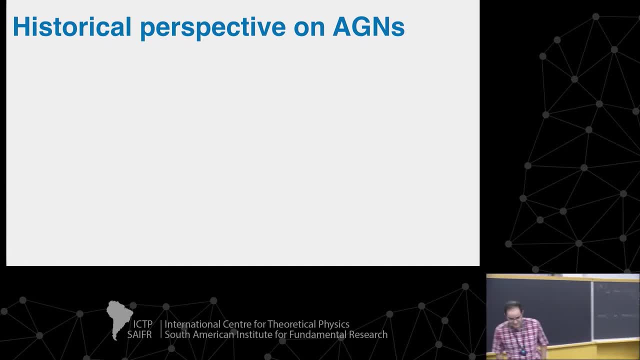 I will summarize here. I will summarize here more than 200, 200 years of history of studies of supermassive black holes, Starting with the first landmark in this historical perspective of agents happened in the 18th century, 1783.. 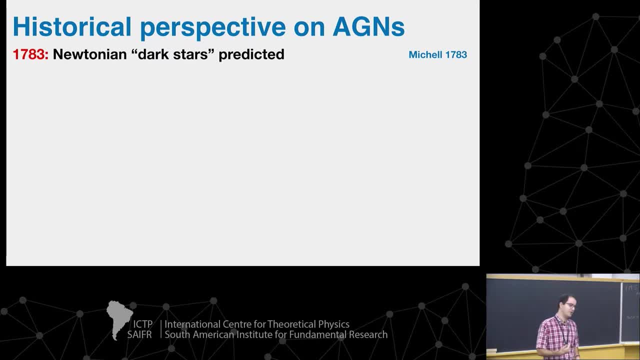 Reverend John Mitchell used Newtonian mechanics and he proposed the existence of mythical dark stars which would have a gravity so strong they would slow down light and imprison light. Okay, so this was the one early version of what we now call black holes. Of course, 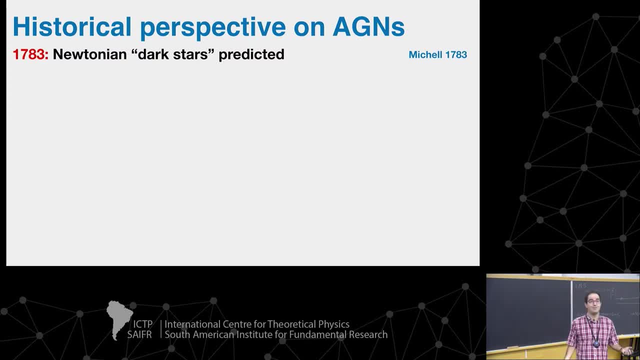 it makes no sense to talk about black holes in Newtonian mechanics. You cannot have a black hole in Newtonian mechanics. Then we have, of course, Einstein publishing the field equation 1915.. And then, shortly after he published the equations. 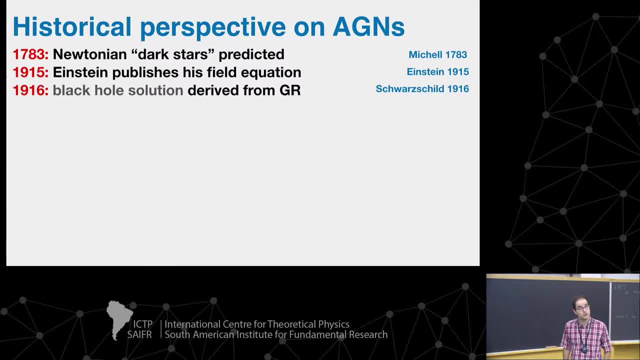 there was this German gentleman, Karl Schwarzschild, working in the Prussian army. finding some free time between calculating ballistic trajectories of cannons, He derived what we now call the Schwarzschild solution of Einstein's field equation, the Schwarzschild metric. 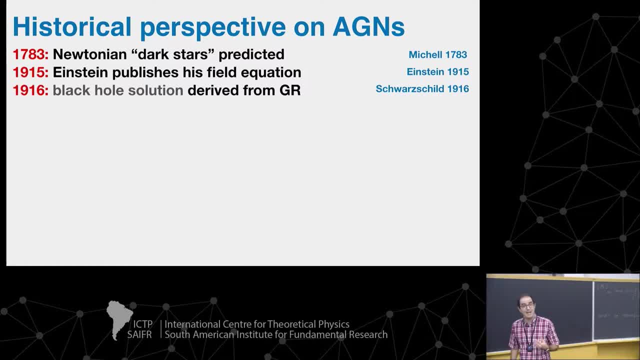 This is really amazing. So this was very important. It's the black hole solution, at least the first and more simple, the most simple black hole solution. And then we have something very interesting: Astronomy starts giving input to general relativity. Well, the feedback between physics. 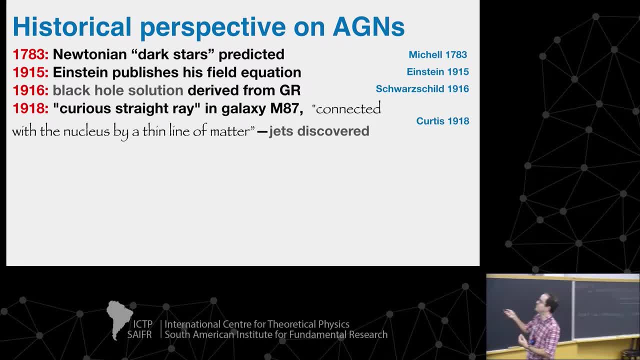 and astronomy took a while. once this observation was taken, So two years after Schwarzschild derived the Schwarzschild metric, the astronomer Curtis. he was looking with an optical telescope to the galaxy that we now image, the event horizon M87,. 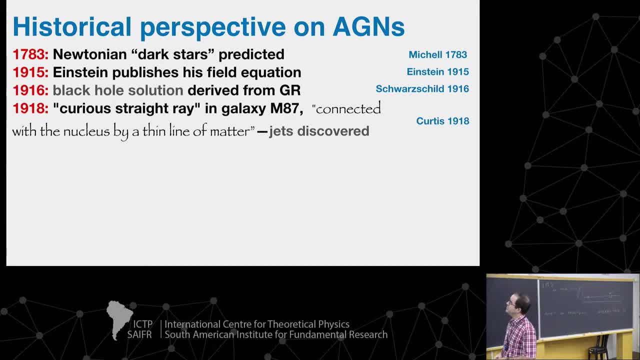 and he made a comment. There is a curious statement about a straight ray connected to the center of the galaxy, A very curious straight ray. Nowadays, when you see straight rays in some images, you think it's a cosmic ray or something damaging your image. 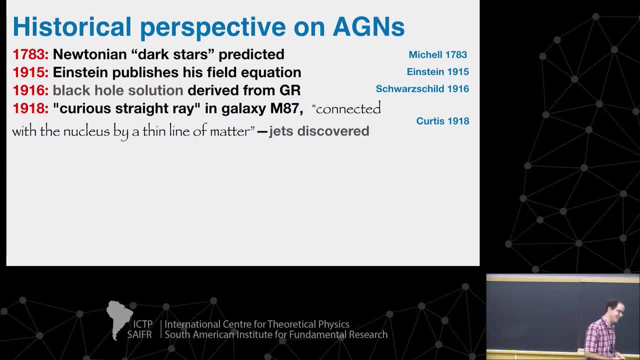 But back then there was not this concept of. He didn't really know what to say of this curious straight ray in galaxy M87.. This is a very important observation because this was a discovery of quasars powered by black holes. Then it took almost 50 years. 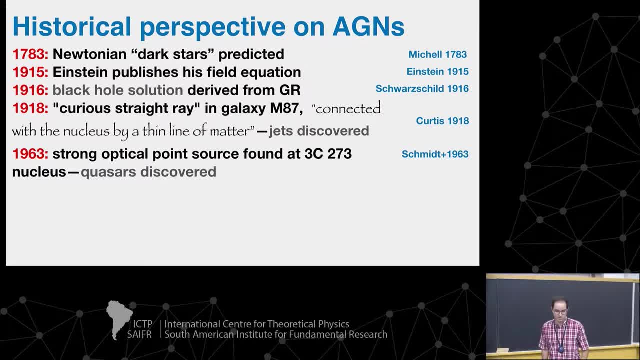 for the discovery of quasars. The Dutch astronomer Martin Schmid found a very strong optical source at the center of the quasar 3C273.. People thought it was a star, It was a crazy star, But then eventually they measured the red shift. 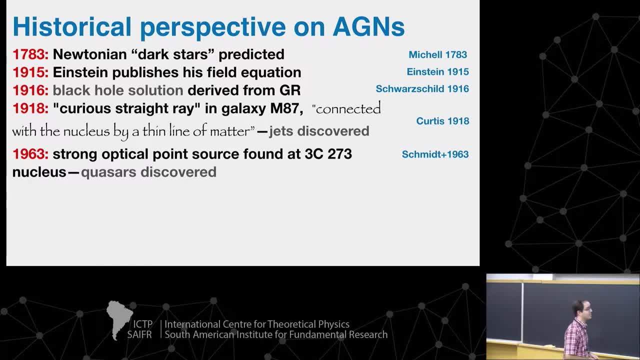 and they found out that this very bright astronomical source is actually located almost a billion light years away from our planet. So what is powering such a brilliant, such a bright object? This was the discovery of quasars and that they are at cosmological distances. 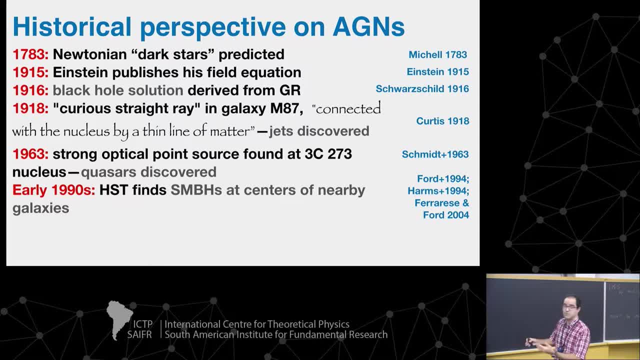 And then it took quite a while. Of course I'm doing a selection. I'm not listing here every single important historical development, Otherwise I would spend the rest of one month talking about the history of the field. Another very important historical event. 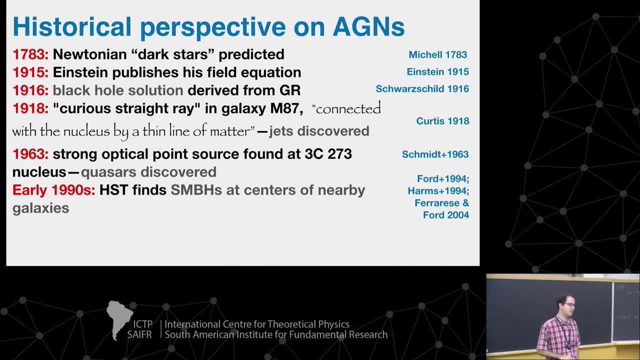 was in the early 90s, with the launch of the Hubble Space Telescope HST, And so Hubble was very important. besides giving an exquisite measurement of the Hubble, constant Hubble also found these dark, massive objects at the centers of nearby galaxies. 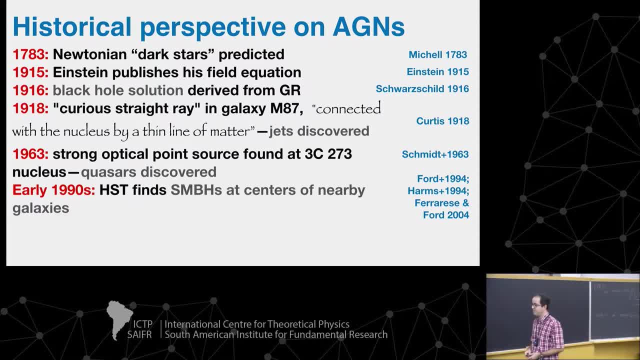 This was extremely important because then Hubble found and firmly established the existence of supermassive black holes at the centers of nearby galaxies. Here I'm listing the papers. If you want to have a look, you know a lot of papers, but this is the two first ones. 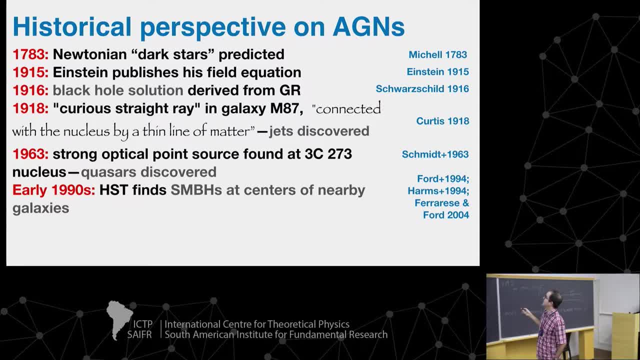 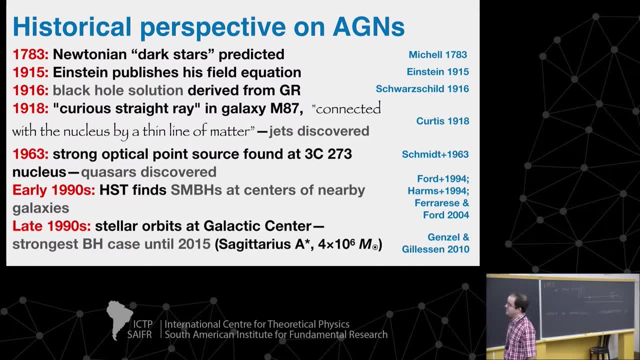 These are very beautiful papers establishing the existence of a supermassive black hole at the center of M87. And this is a review paper. And then, in the late 1990s, there was another breakthrough by the group of the UCLA, group of Andrea Ghez. 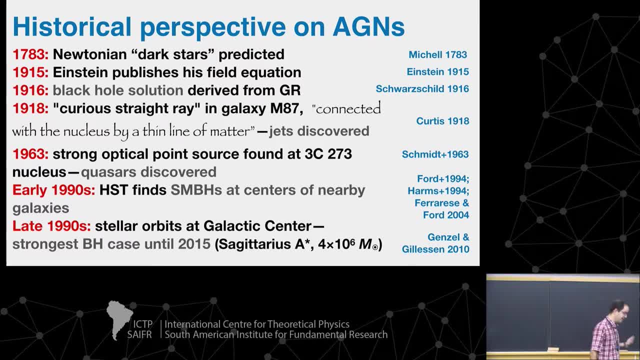 and also the group of the German group of Genzo. They were able to pinpoint, to image individual stellar orbits around the center of mass of the Milky Way And they were able to measure the mass, this dark mass, at the center of our galaxy. 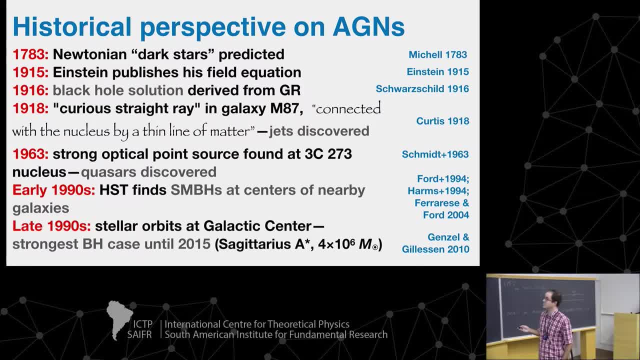 And they firmly established the supermassive, the existence of the supermassive black hole at the center of our galaxy, which we call Sagittarius, A star with a mass of four million solar masses inside the event horizon. And Sagittarius A star. 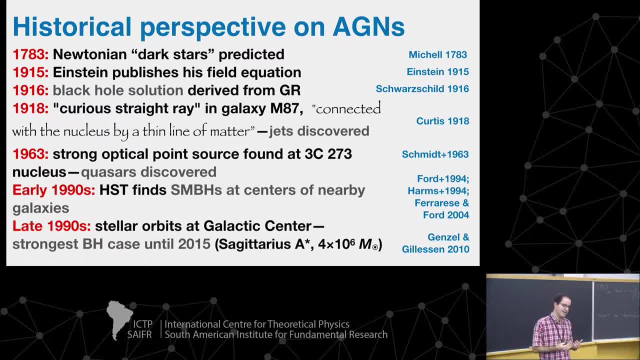 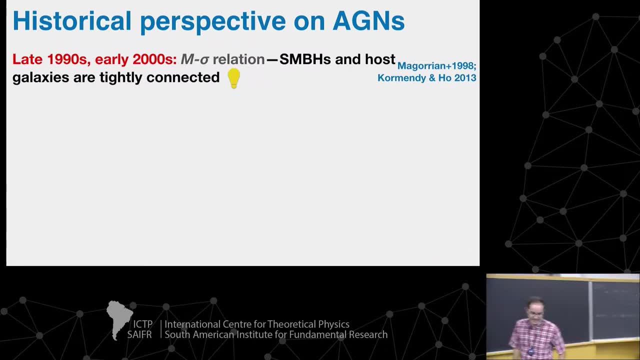 remained the strongest black hole, the strongest case for a black hole, until three or four years ago, with the gravitational waves That established the existence of, firmly established the existence of stellar mass black holes. I will try to go move a bit, a bit quicker now. 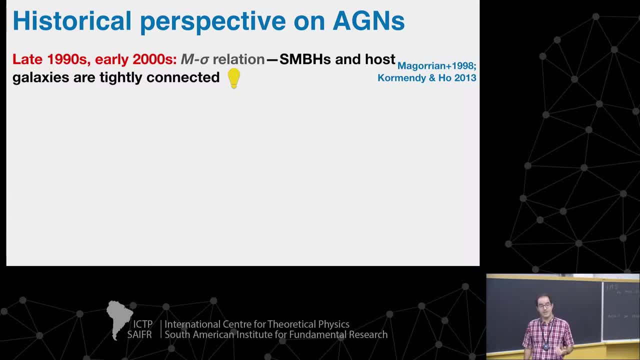 So, as you will see, things start accelerating, The rate of discoveries starts accelerating. In the late 90s, in the early 2000s, there was this very important discovery that we now call M-sigma relation. So M is a property. 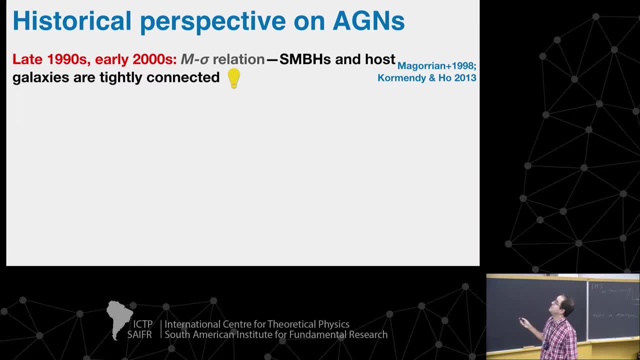 of the central black hole, and sigma is a property characterizing the velocity distribution of stars in the bulge of the galaxy, And so there was this discovery of this correlation. Somehow the host galaxy, in measured in terms of the sigma property, is talking to the central black hole. 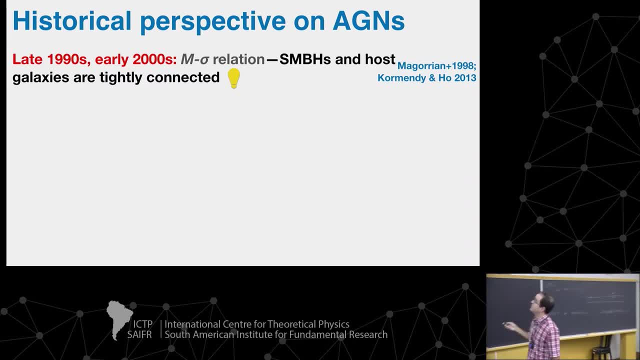 And this was not expected. I will give more details why. this was almost completely unexpected by the theorists. So this established the supermassive black holes and host galaxies are tightly connected. This was a major surprise to the theorists. They didn't see it. 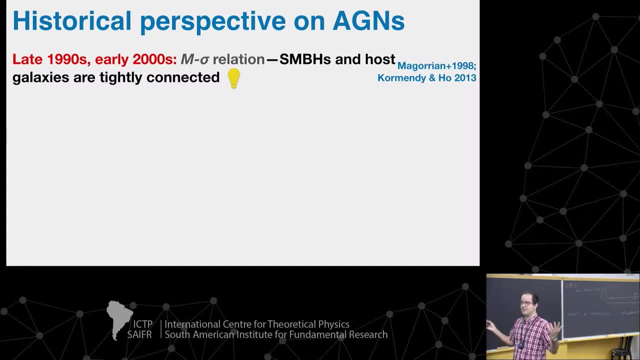 Almost 95% of them didn't see this result coming. This is the birth of the field we now call AEGN feedback, The feedback loop between the central dark mass and the host galaxy. Then, in 2000,, a few years afterwards, 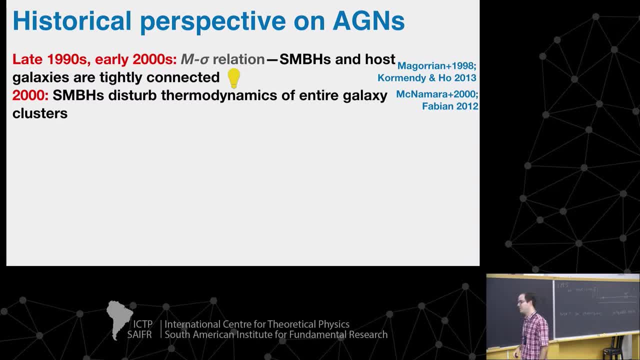 there was this other very important result that supermassive black holes. apparently they are able to substantially disturb the thermodynamics of entire galaxy clusters. This was a huge surprise. Then, in 2003,, this survey, this astronomical survey called Sloan Digital Sky Survey, 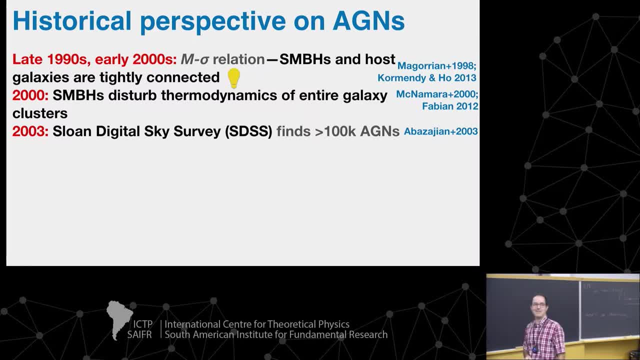 discovered more than 100,000 quasars in the sky, So this was a huge breakthrough. So supermassive black holes: they are not rare. Every galaxy basically has a supermassive black hole, But this was observations- concrete spectral. 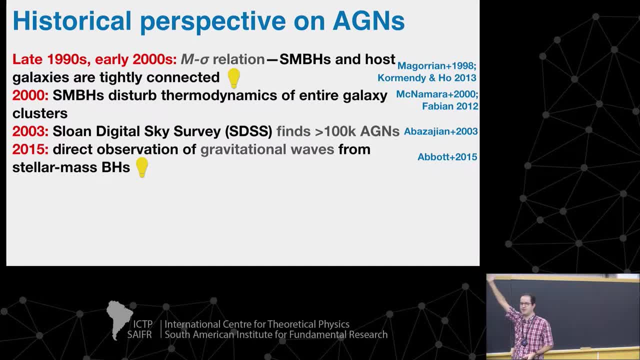 and imaging observations of this more than 100,000 quasars. And now we get to 2015 with the historical Nobel Prize winning direct observation of gravitational waves from the merging of stellar mass black holes. And why should I mention a result related to? 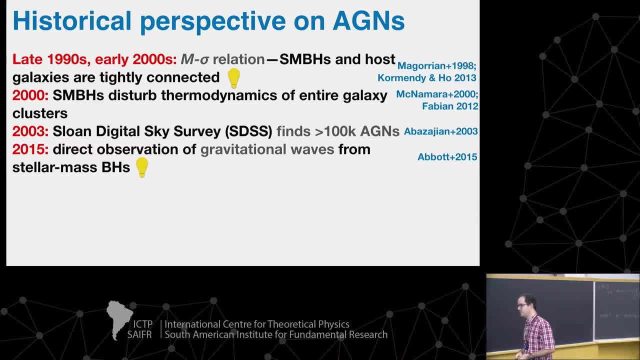 stellar mass black holes in a talk about, in a lecture about supermassive black holes, And the reason is that this was really important because this really you cannot really now question that there are no black holes in the universe. Nobody questioned in 2015. 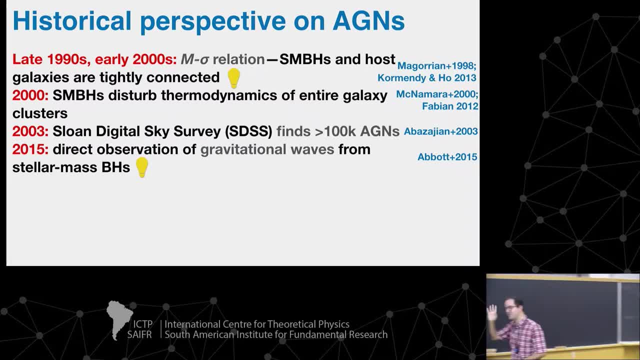 that there were no black holes. A couple of people still talk about gravastars and some other boson stars, some strange objects, But it's just a minority of the community that didn't really that questioned black holes. Black holes were already a paradigm. 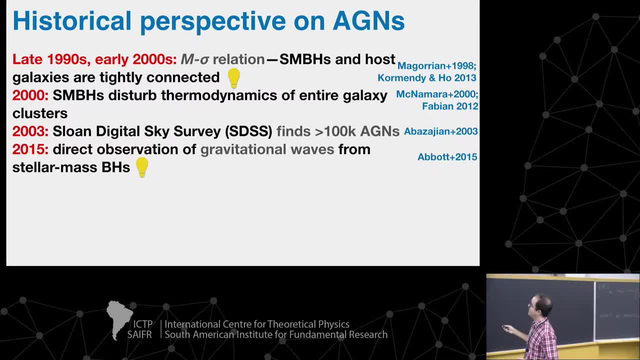 a scientific paradigm four years ago, But this really firmly established, using the sound of space time gravitational waves, that black holes do exist. You cannot explain the waveform without the black hole solution. Finally, we now have 2018, the first multi-messenger observation. 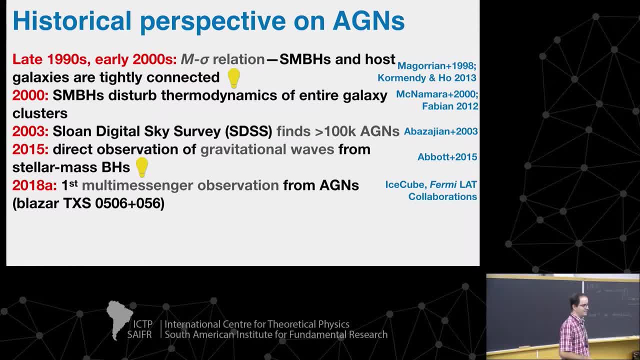 of an AGN, the blazer TXS. I will not pronounce the WhatsApp number of the blazer And, by the way, next week we will have a hands-on tutorial Where you will learn how to analyze the gamma-ray observations of this blazer. 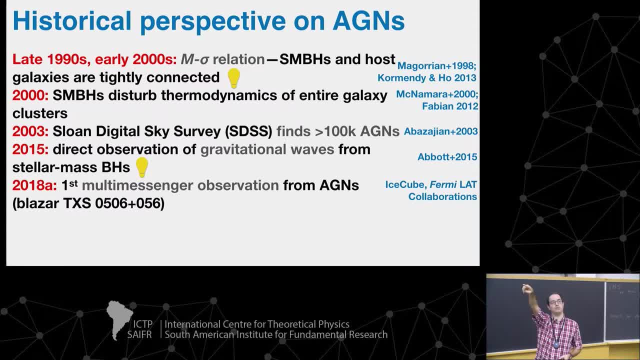 Right, Fabio. So Fabio, there will teach you how to reproduce the. Unfortunately, you will not be able to publish this again because there were already a couple of science papers with this result, But Fabio will teach you how to reproduce the result. 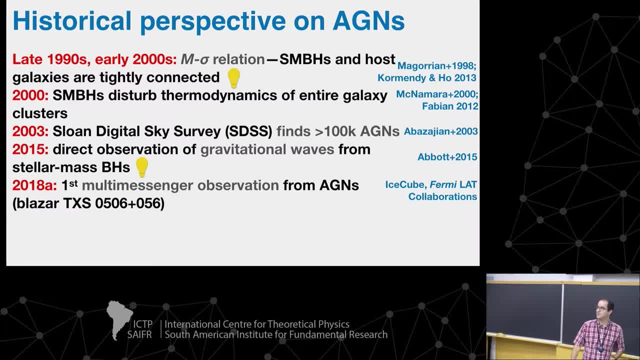 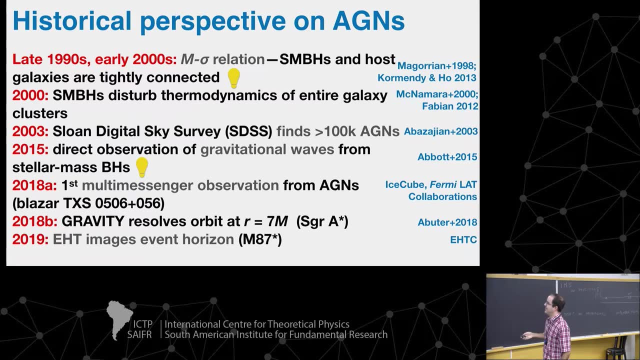 in the science papers. Okay, Right, Fabio. Okay, But maybe in another blazer you can still analyze and publish a nature or science paper, Who knows? Okay, so gravity. Okay, I will skip the result by gravity. I will go directly to now. 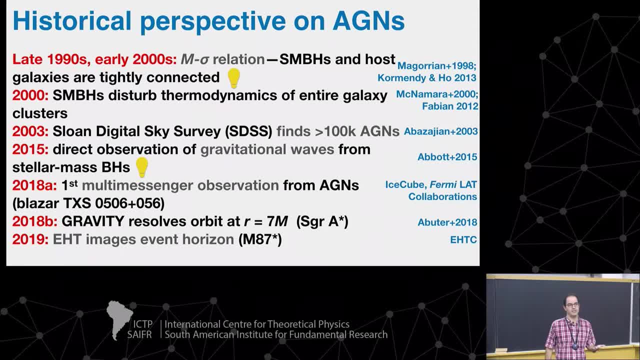 I am sure that all of you saw the EHT image five months ago, which was really a breakthrough in black hole physics and black hole astronomy, Where the first image of an event horizon in the history of science And precisely the first, Curtis observed the jet. 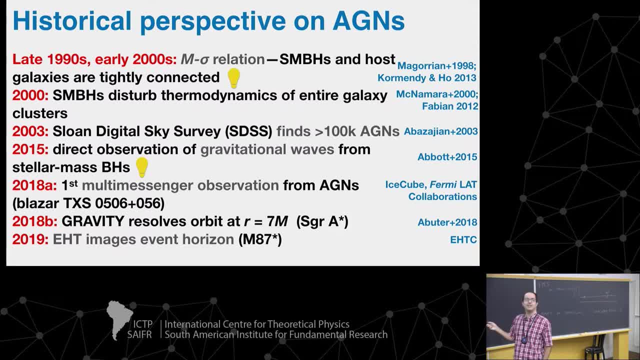 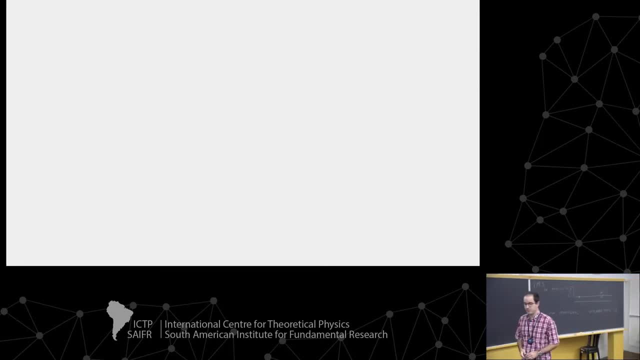 from this object 100 years ago And 101 years later we observe the event horizon. This is amazing: the evolution of science. So what are the lessons from this broad historical perspective on the study of? What are the general lessons we can learn? 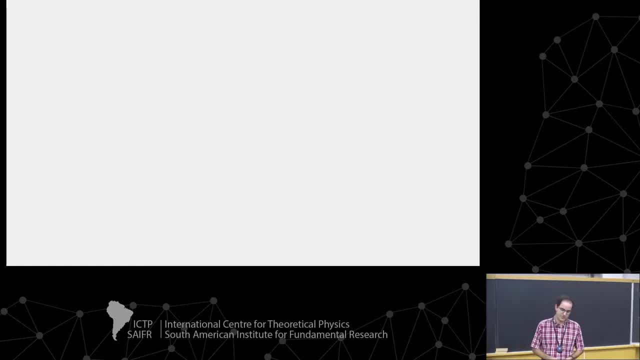 from this broad spectrum of discoveries. The first lesson is that we can write an equation. If you take the dot, product of new technologies, with engineering advances, Okay, You open. That equals new astronomical windows being open for science, Okay. On the other hand, 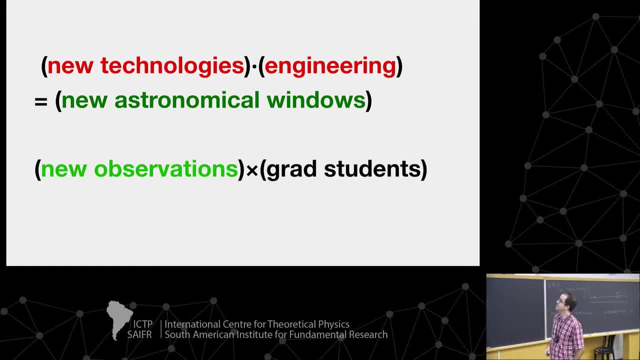 if you take the cross product of the new observations produced by this new astronomical windows. you take the cross product with grad students and you get paradigm-based observations. Okay, So we can write these two equations here. The lesson is that every time a new astronomical window. 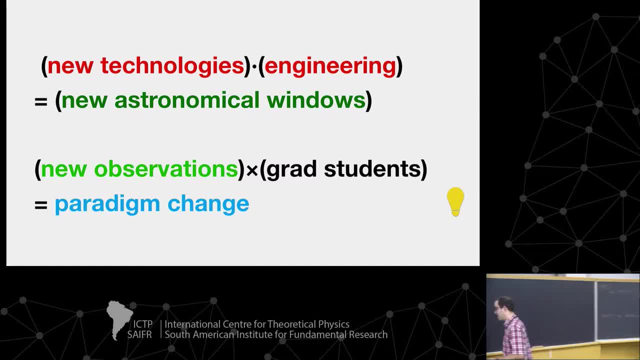 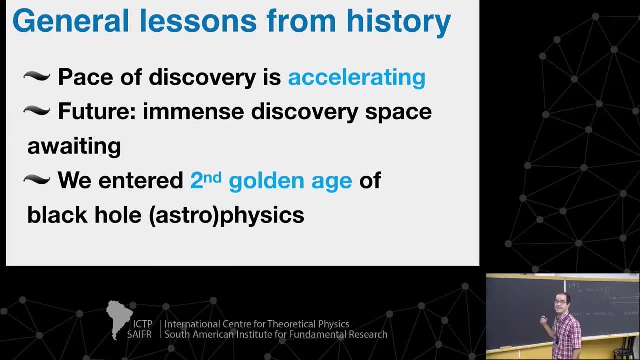 is open, the universe turns out to be far stranger than the wildest speculations. Okay, So this is one of the lessons we learn from these discoveries. We have a couple of other lessons. The pace of discovery is accelerating If you pay attention. 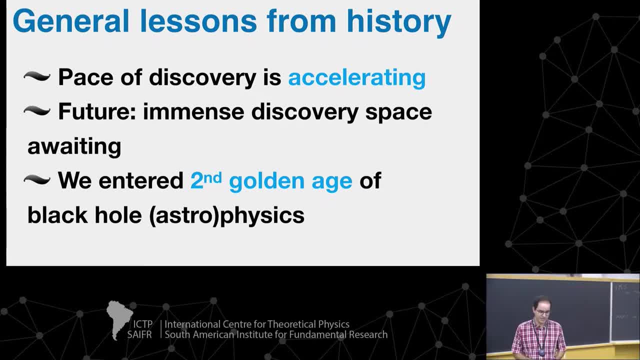 to what's happening in every field of science, in particular AGNs. there is a huge discovery space awaiting for you to participate in the scientific narrative And in my opinion, we entered a second golden age of black hole physics With the LIGO-VIRGO results. 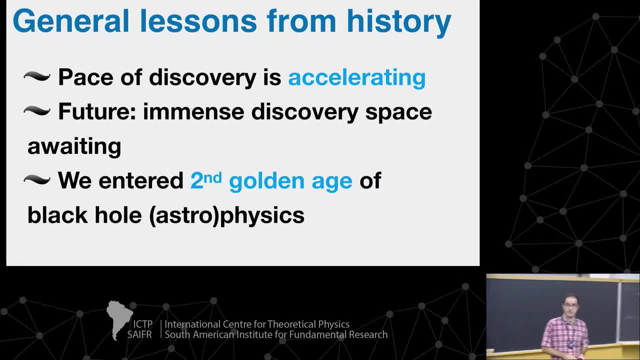 we entered a new golden age, The first golden age. the physicists that specialize in the field theory of GR they call the epoch of the 60s. they call it the first golden age. 60s to the 80s of the golden age. 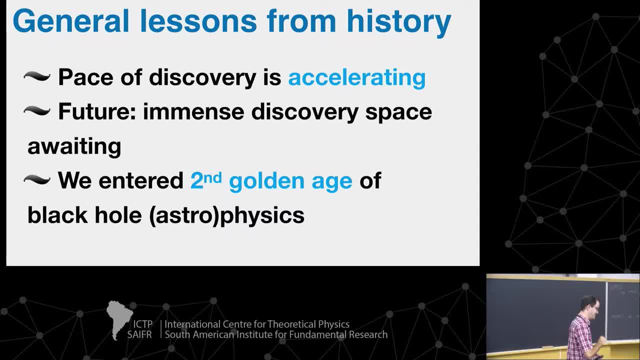 of black hole physics. So this is the golden age of black hole physics. This is the golden age of black hole physics. We entered the early 70s and I think we entered a second golden age of black hole physics driven by observations. 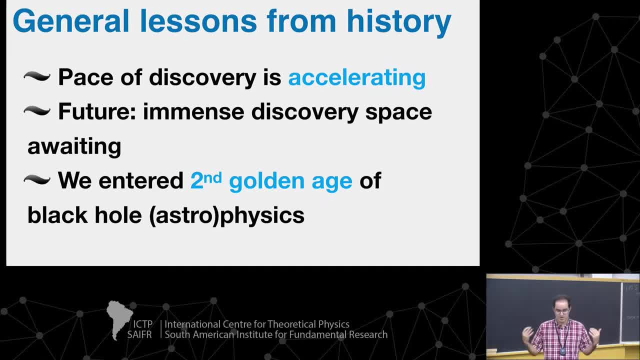 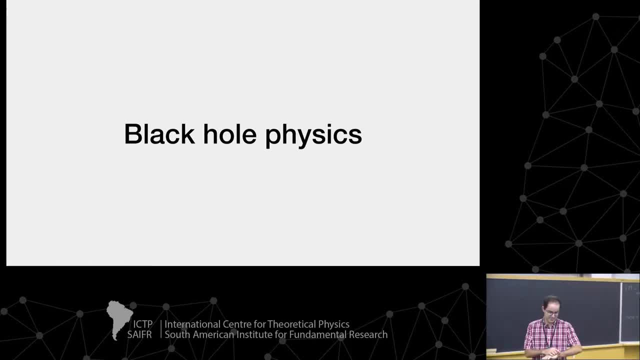 not only analytical calculations and simulations, but mostly observations. Okay, so now that we did this broad historical overview, let's talk about black hole physics. So my idea now over the next 20 minutes or half an hour is to talk about black hole physics. 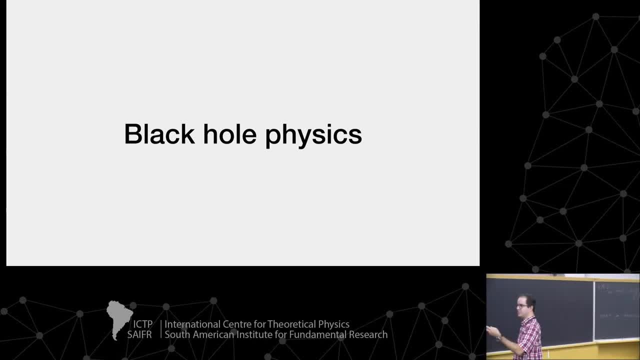 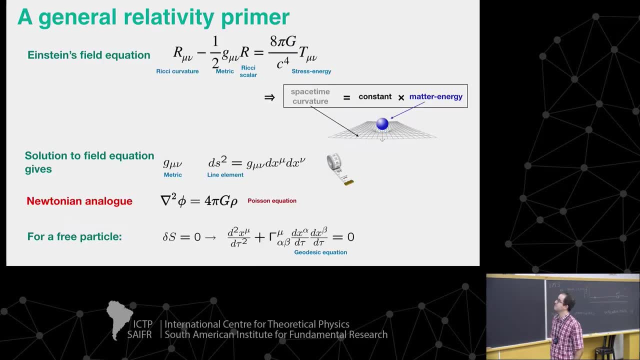 and the next two minutes is to give you. the next two minutes will be give you a very broad overview of black hole physics and if we want to understand black holes, we need to understand general relativity. I'm not sure how many of you took a course. 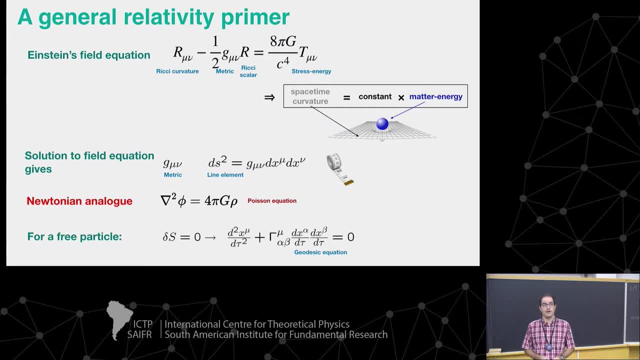 of GR as an undergraduate students or graduate students. I don't think I will ask: Okay, there is way more participation. Okay, so most of you good, Okay. so I'm surprised that most of you never heard or don't really know. 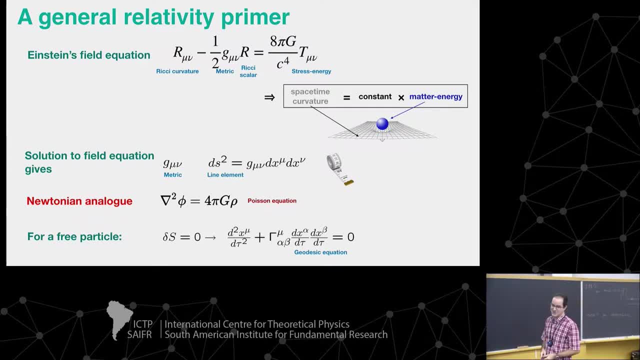 about AGNs. but good, It's really good. It really gives me motivation to continue this lecture. Right, so well. general relativity: this is a very advanced field. equation: Okay, we have all the well-known tensors there. 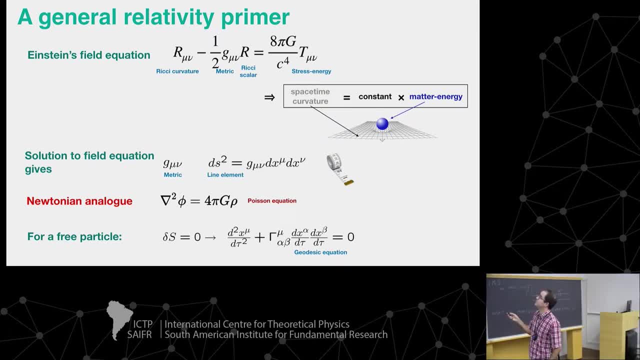 the Ricci curvature, the scalar contracting the tensor, on the left side the metric, And on the right hand side we have the stress energy tensor with the energy distribution of some system And you solve this equation. the equation will speed out what 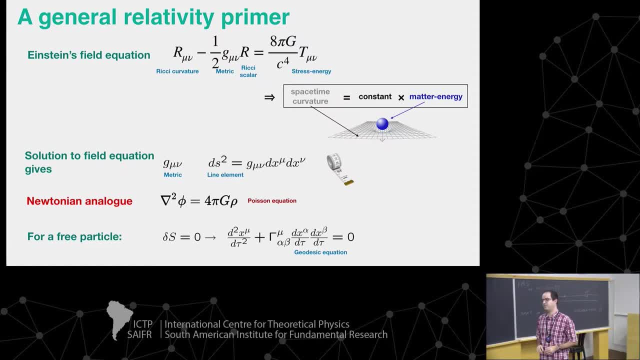 is the space time? what is the curvature? You can only solve Einstein's equation analytically for a couple of cases. If you start putting more astrophysically interesting things into the equation, you can solve the mass energy distribution with this tensor. 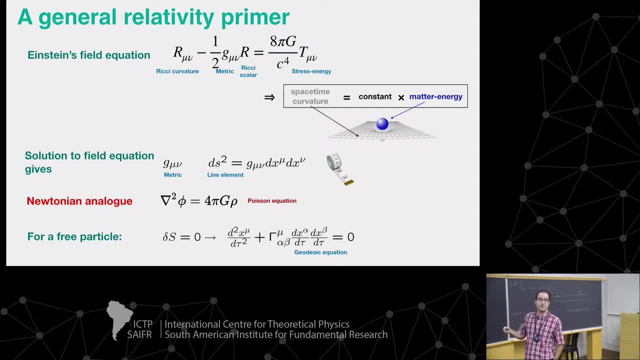 metric encapsulates the space time properties And then you can characterize geometries with the tools of differential geometry to learn about the motions of test particles in this curved space time. So this is a summary of GR in one minute, or perhaps two minutes. 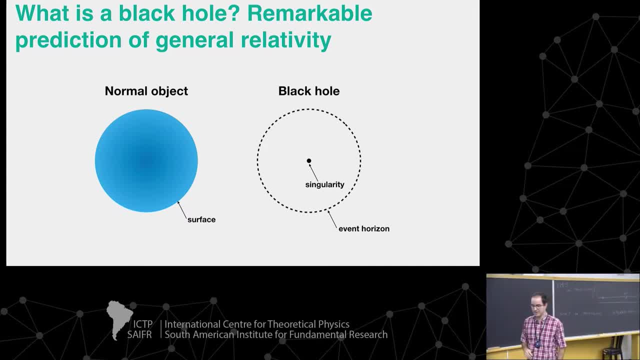 And GR predicts the existence of black holes. So black holes are these remarkable predictions of general relativity. The black hole is a black hole. This planet, or even a gaseous atmosphere like a star black holes? they don't have a solid 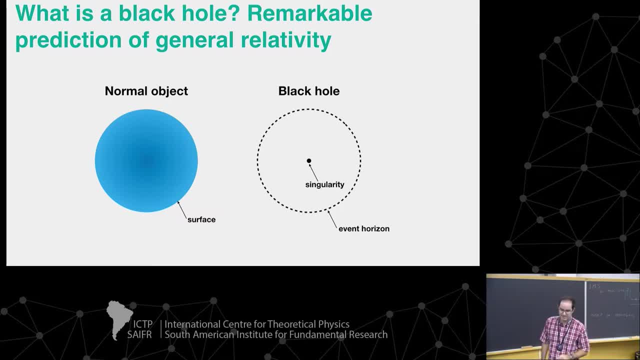 surface. So a black hole has no the surface of a black hole, or we can call it a black hole. So this is a very interesting hypothesis And we can actually test black holes in the universe by the tidal forces near the singularity. 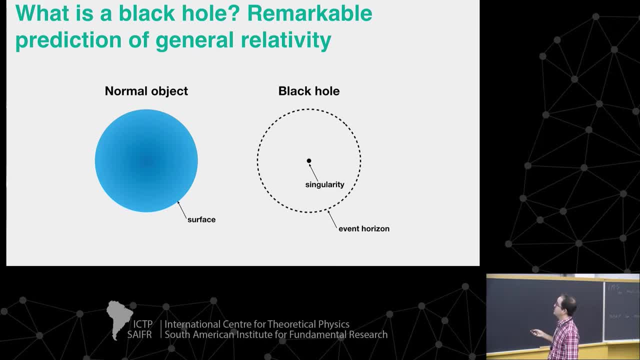 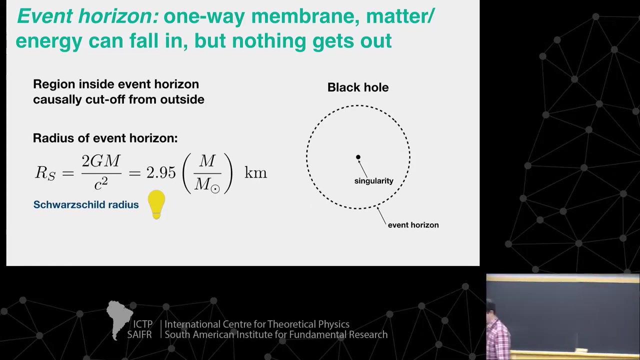 or even before you reach the singularity. So this is, this is the part of the universe And we can see. the particles will be converted to some other form of energy when the particles collide on the surface here, If you do the same with 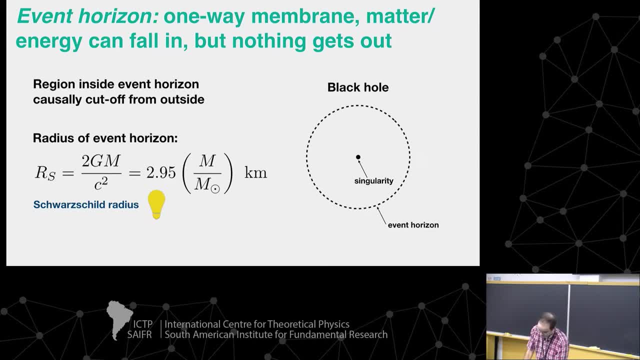 a black hole. they will go inside and they will not see this necessarily. light cone. You are doomed to meet the singularity in your light cone once you get inside the event horizon It's causally disconnected from the outer universe, from the solution. 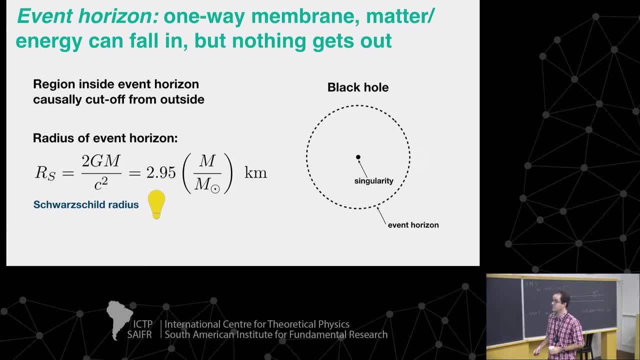 of the outer space time outside the event horizon From the square of the speed of light. So this is three kilometers for a black hole with the mass of the sun. Also, another meaning of the Schwarzschild radius is that the gravitational time dilation. 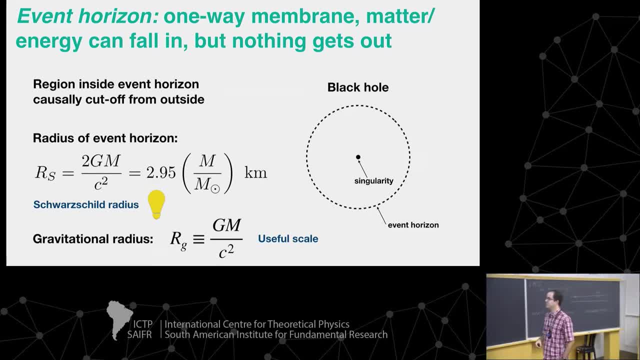 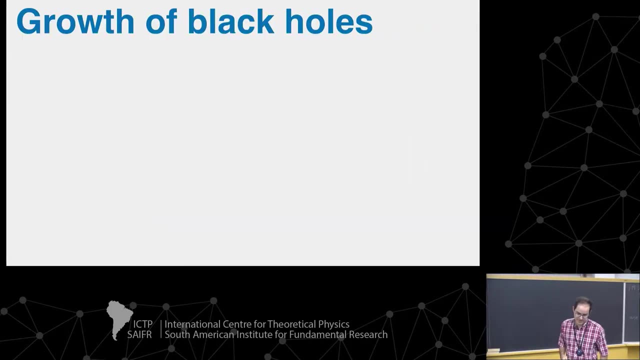 goes to infinity near the event horizon. Another important side in relativistic astrophysics is the Schwarzschild radius divided by two. This is a very useful scale when you are talking about black hole astrophysics. What happens when black holes? 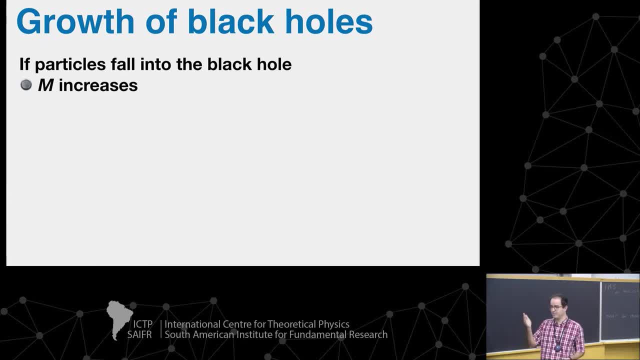 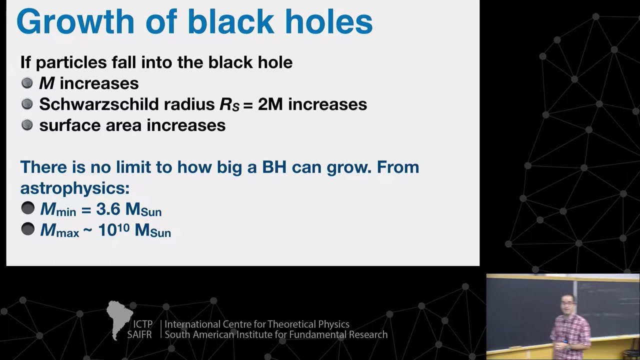 interact with their environments. If nature is a black hole, they will penetrate the event horizon And because the mass will increase, they will add up to the mass of the black hole. the Schwarzschild radius will grow as well, because the Schwarzschild 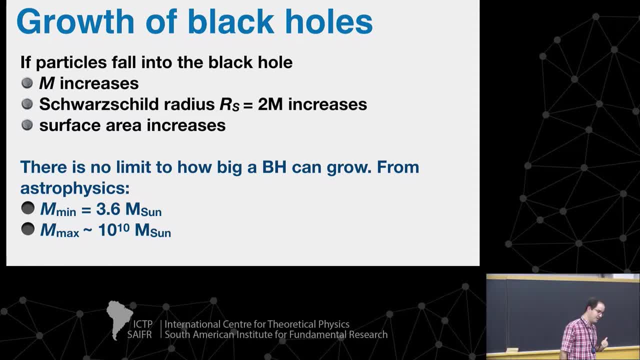 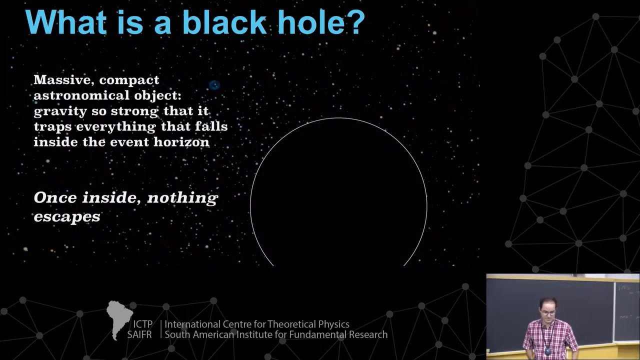 radius of the black hole is. the smallest mass that we have measured for a black hole candidate in astronomy is about four solar masses and the biggest mass ever measured for the black hole is the mass of the black hole, So the mass of the black 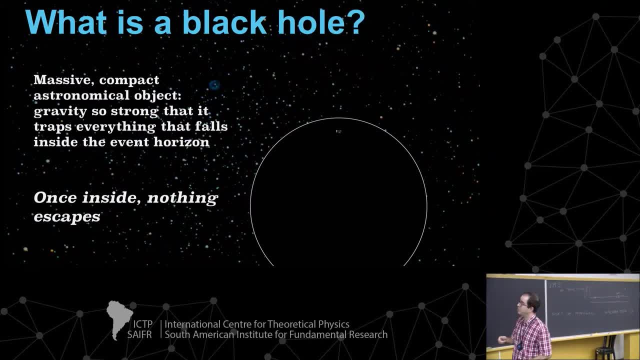 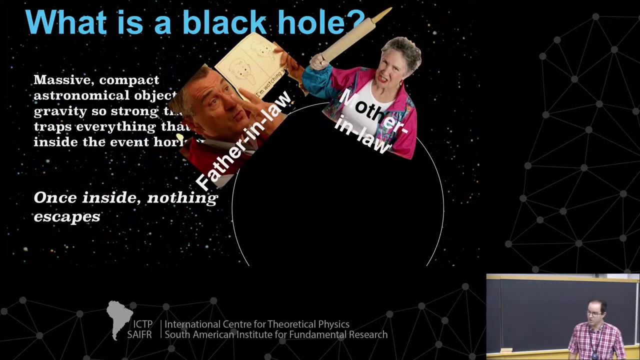 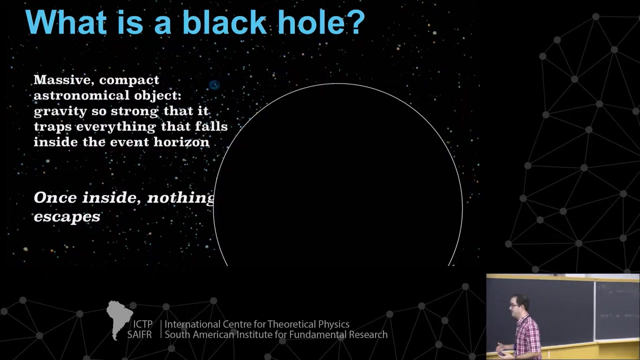 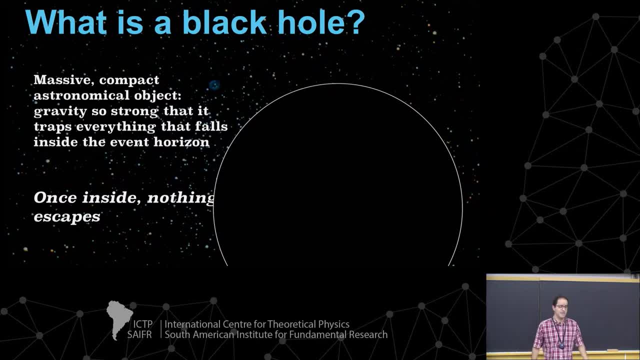 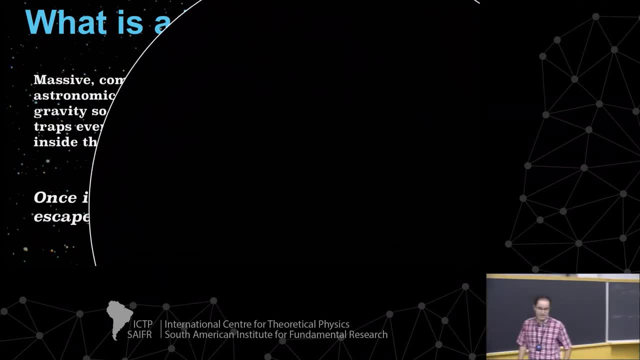 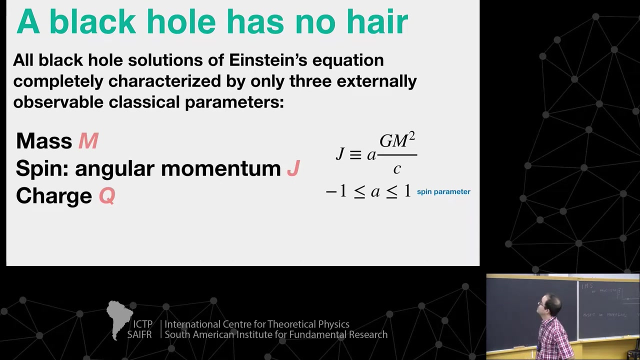 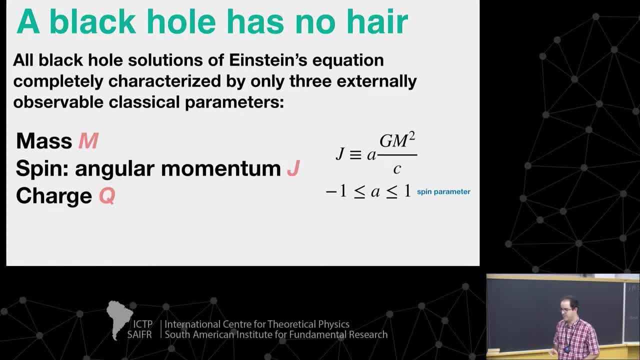 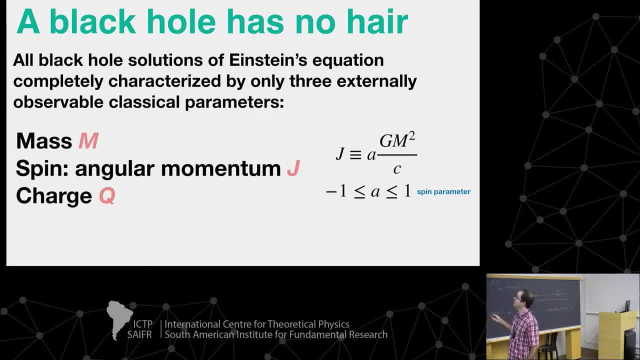 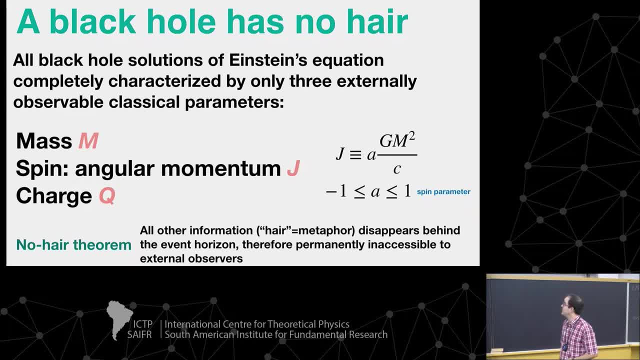 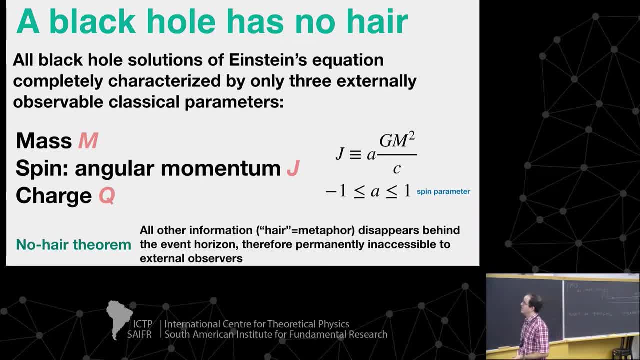 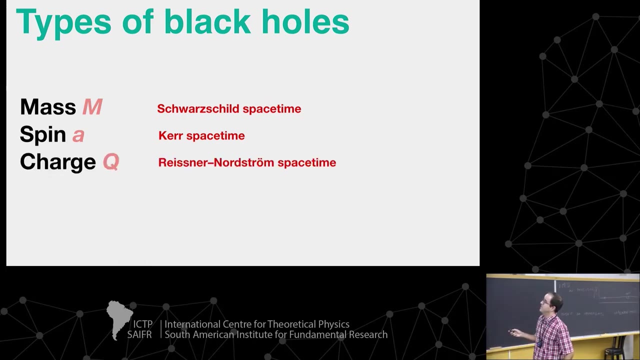 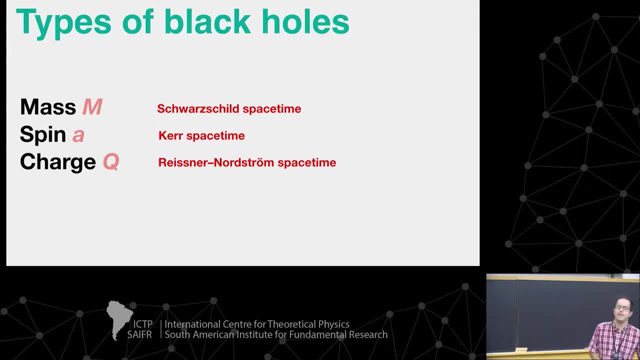 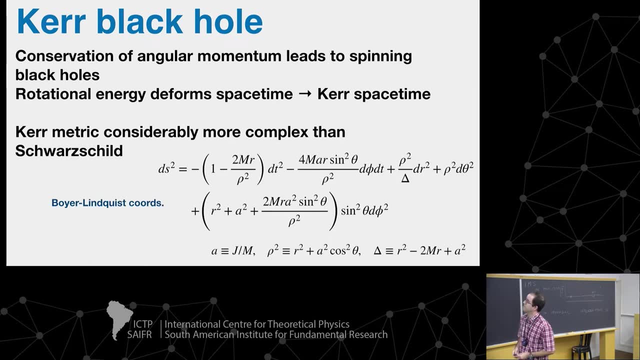 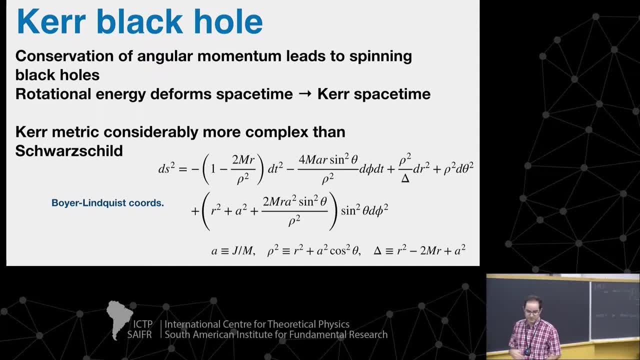 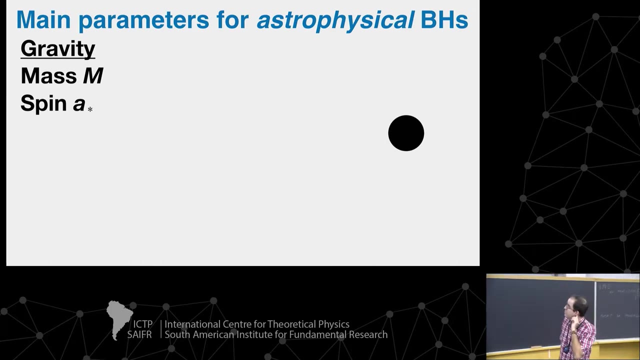 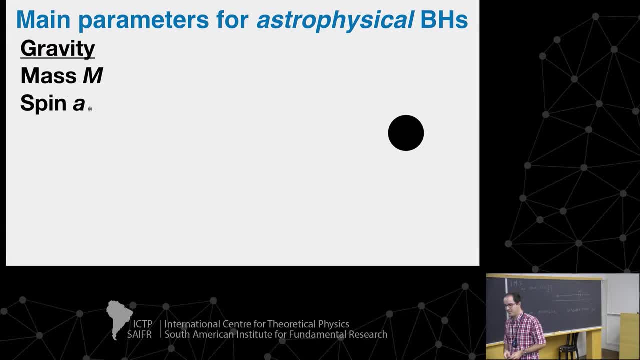 hole. So what fascinates me when I study AGNs, when I work with AGNs- I hope my students are also fascinated by this- is the fact. okay, so they are interacting. they are actively interacting with their black hole. 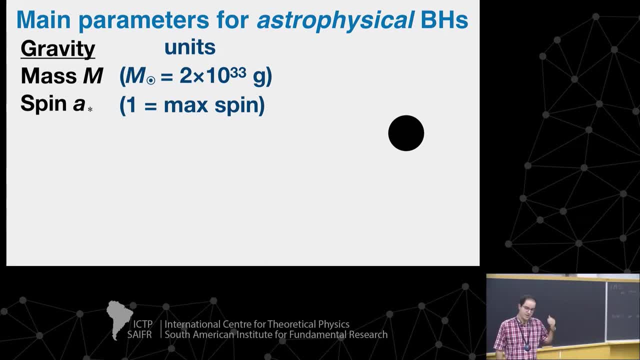 mass, So the units that we usually adopt to describe the mass we talk about black hole masses in solar masses. This is the standard unit in black holes. These are the mass of the black hole mass. All the mass is equal to one. 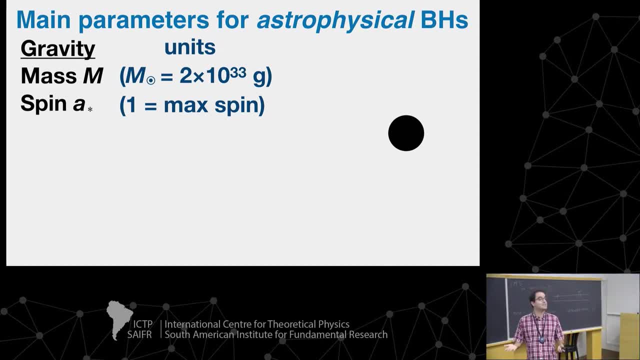 mass of black hole. So black hole mass is equal to the. Okay, now we need other numbers. Another number you need to describe an astrophysical black hole is this number here, which we call the mass accretion rate. It is the rate the units of this m dot is mass over time. 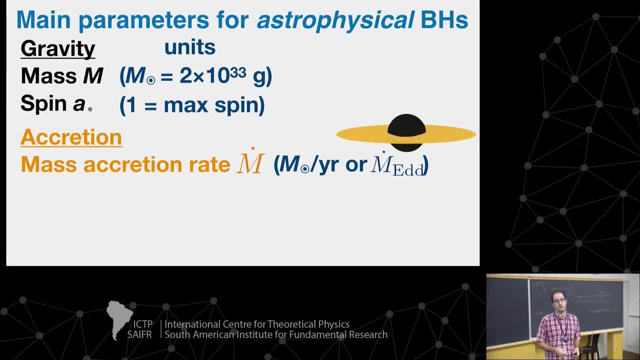 So this is the rate of falling of matter into the black hole. We call it mass accretion rate. Accretion is a word coming from feeding, from accreting, from putting matter onto something. The usual units of mass accretion rate- m, dot in astrophysics. 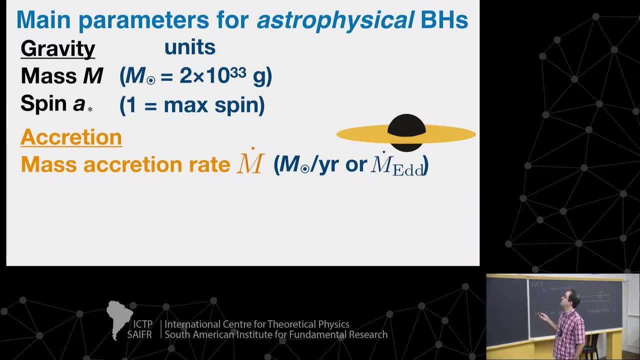 are solar masses per year. This is very common. Also, we like to characterize the mass accretion rate in units of this quantity, called Eddington mass accretion rate. I will describe what is the physics, what is the definition of this soon. 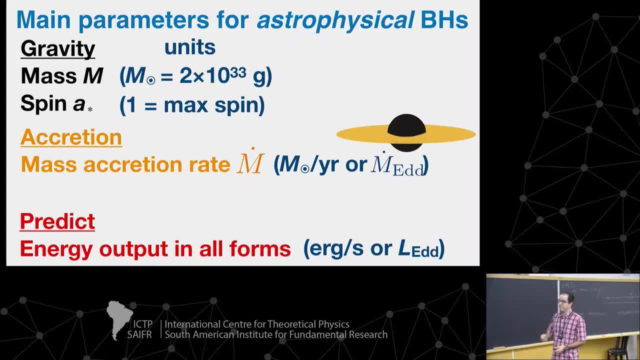 And our dream when I put my theorist hat, the dream of theorists working in this field is: given these numbers, given the mass, given the spin, given the mass accretion rate, we would like to predict everything about this system. 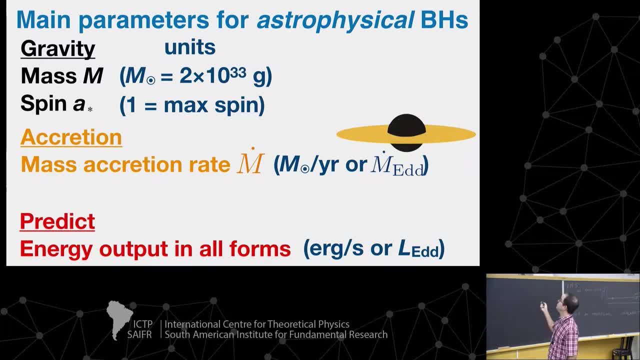 We would like to be able to completely predict the energy output from this system, And when I talk about energy, I'm talking about the energy flowing out from the accretion disk, but also energy flow Flowing out in kinetic form, in outflows and relativistic jets that we call in astrophysics. 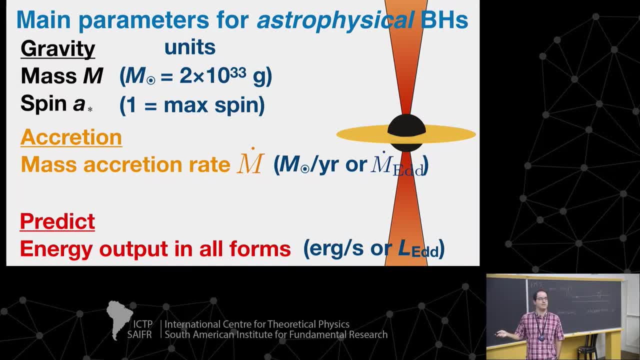 Suffice to say that we do not have a full theory for this, So there is lots of opportunities for theorists working to predict everything about the total energy output of the Kerr spacetime based on these three input numbers. And we prescribe energy output in astrophysics. 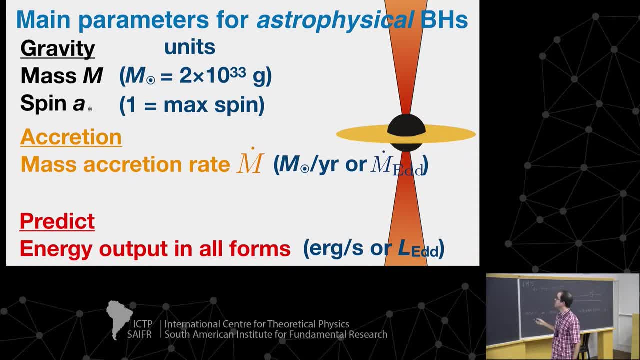 usually using ergs per second of power, Or in terms of the so-called Eddington luminosity, which I will define very soon. Okay, another thing I should mention is that some people, myself included, think that a fourth parameter necessary to describe astrophysical black holes. 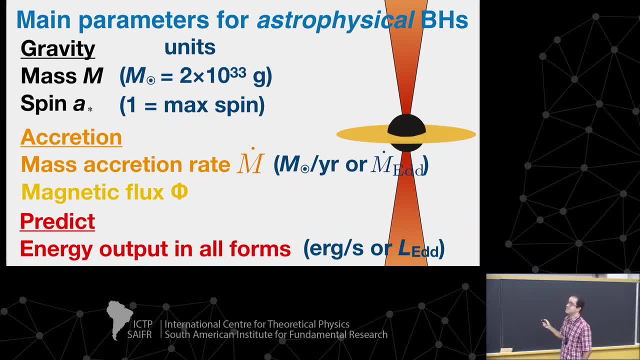 besides M A star and M dot is the magnetic flux. It is not very clear to us what is the role of the magnetic flux, but it turns out that the magnetic flux is the role of the magnetic flux. And it turns out that when you feed magnetized plasmas to Kerr spacetime. 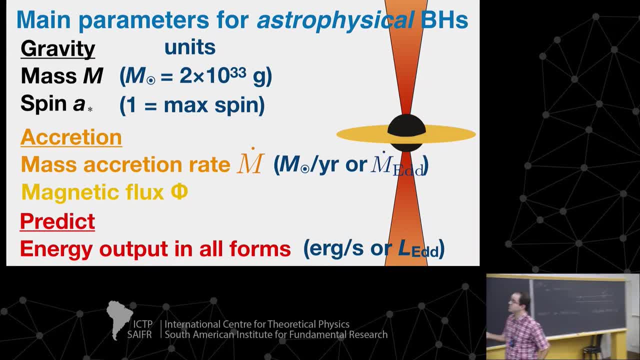 you can have very interesting consequences. So it seems to the theorists that the flux, the magnetic flux accumulated near the event horizon is an extra important parameter. But to first order, let's only worry about these three numbers. okay, Magnetic flux will come tomorrow. 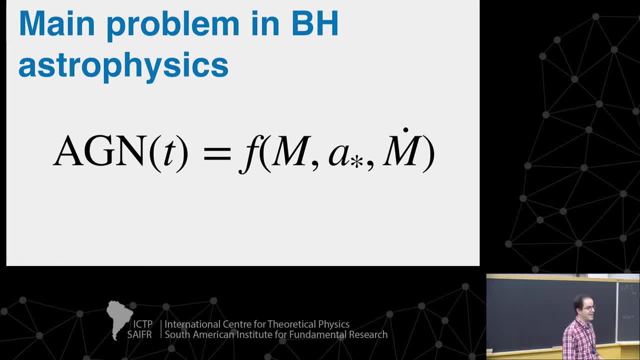 Okay, Okay, Okay. So this is the main problem in black hole astrophysics: We want to predict, as a function of time, the appearance and the behavior and the energy output of AGNs, Once we provide the mass, the spin and the accretion rate. 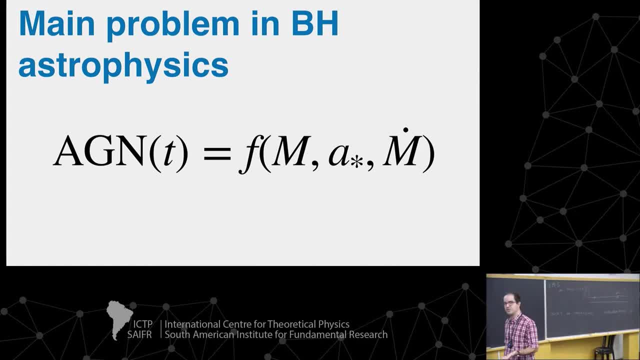 in practice this means specifying initial conditions and boundary conditions, putting the spacetime and trying to see if what we get is nature, is the observed universe. Also, people want to do a GRB over time function and a stellar mass black hole time function. okay, 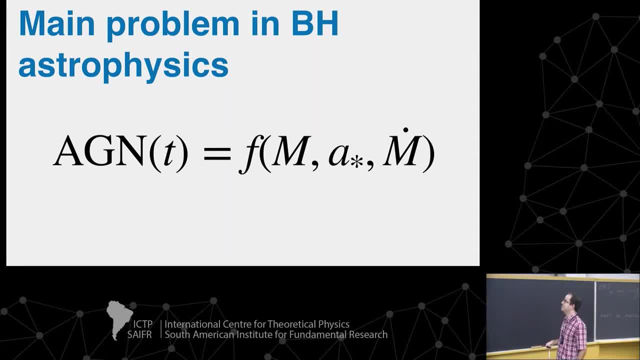 So this is not only AGN, but stellar mass black holes and gamma ray bursts Also. we want to describe them. This is the dream of theorists working in black hole astrophysics. We also want to. we want a function for AGNs, GRBs and X-ray binaries. 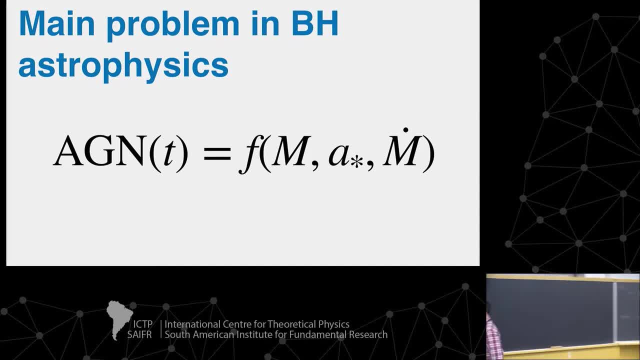 Okay, Fabio, Fabio, how much time do I have? I think we have 10 minutes for the class, 10 minutes, 10 minutes. okay, 10 minutes, very good, very good, very good. I'm very slow as usual. 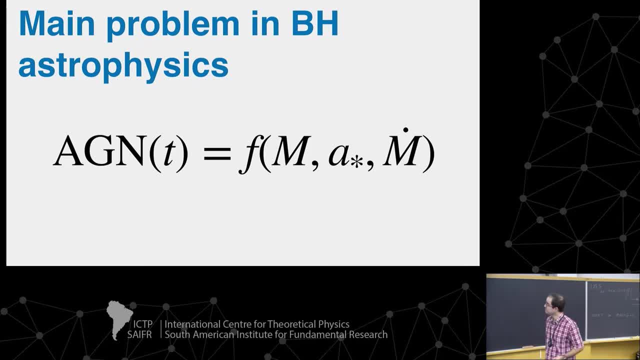 But I think it's important to get the basic concepts here. Okay, so let's begin talking about important, important quantities that you need to understand the literature and results. Okay, Okay, Okay, Okay, Beginning with this quantity called Eddington luminosity. 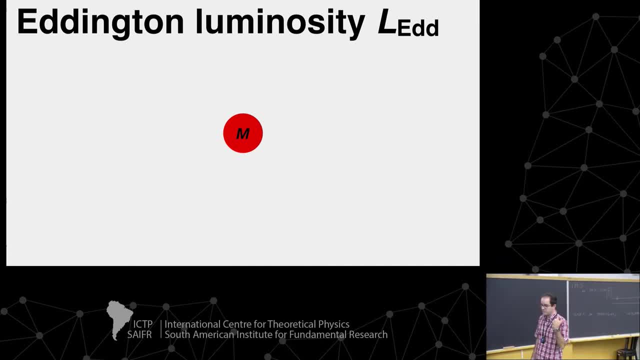 which I just referred to in the previous two slides ago. So what is the Eddington luminosity? The Eddington luminosity is the following: Suppose you have a central object with a mass m and this object is radiating away a photon field. 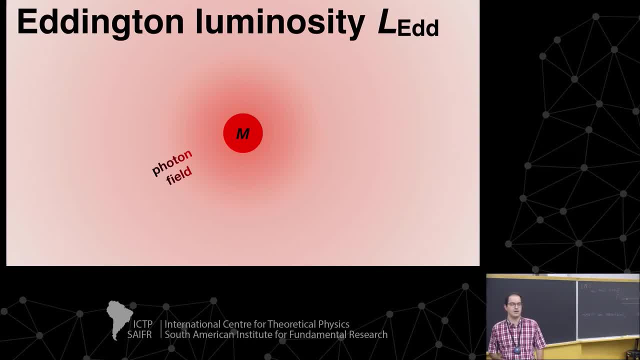 Okay, So the central object? it could be a star, It could be stars, It could be the energy flowing from cities on a planet. okay, It could be an accreting black hole, It can be anything. It doesn't really matter what the central object is. 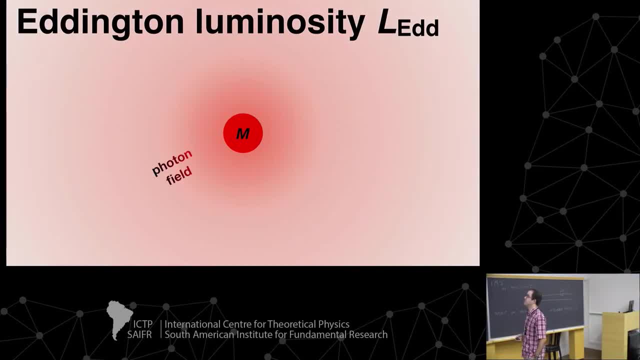 Suppose this object is producing a photon field, a radiation field, and we can describe this photon field with a luminosity, okay, A luminosity, the power in radiation emanating from the central object. As I mentioned, it can be a central black hole. 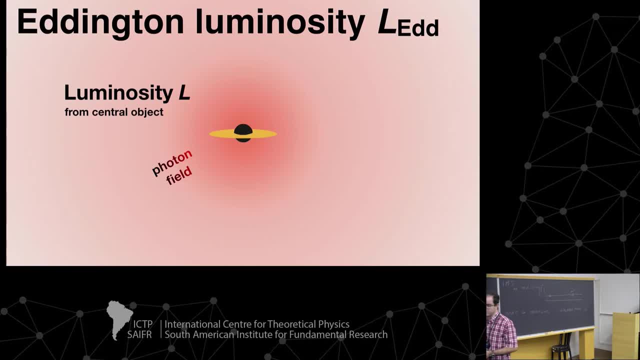 We can ascribe this concept to an accreting black hole And imagine that you have a plasma of electrons and protons that are surrounding, in a spherically symmetric way, the central object with a mass m. okay, So you have this plasma of electrons and protons. 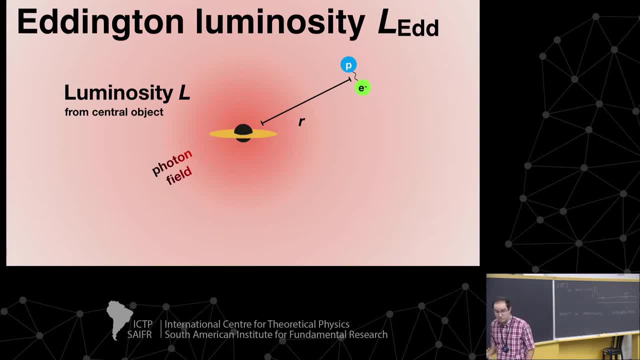 which are talking to each other with the Coulomb interaction And, let's suppose, a pair of electron-proton at a distance of r from the central object. okay, So the basic question to understand the concept of Eddington luminosity is: 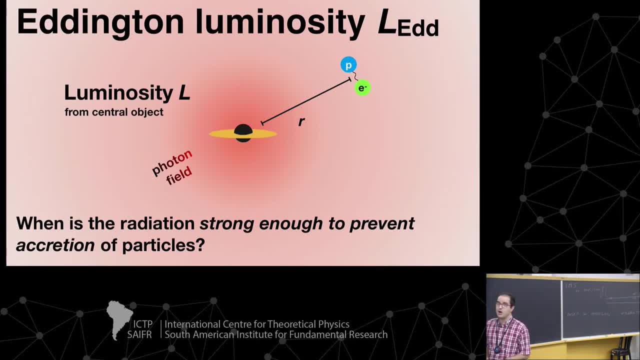 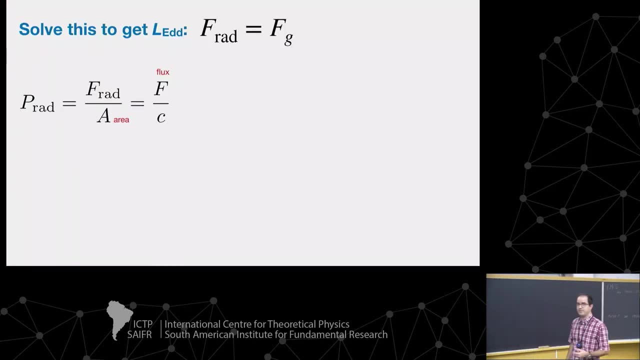 when is the radiation field strong enough to prevent the gravitational infall of this pair of particles? okay, This is the central question that we have to answer to understand what is the Eddington luminosity. So, in order to understand what is the Eddington luminosity, 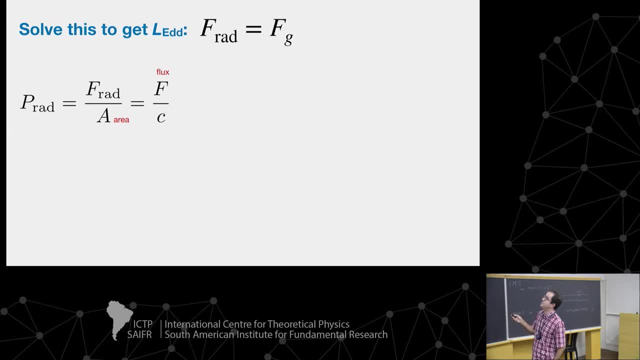 the Eddington luminosity is defined when we have the equality between the radiation force due to the radiation pressure and the gravitational force that is making it fall towards the central object. So we define the radiation pressure, okay, The radiation force over area where the force is acting. 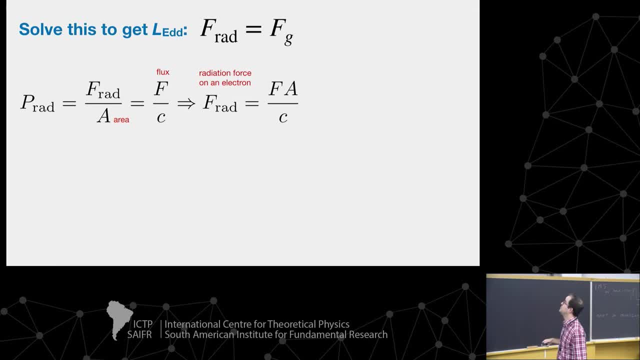 and the radiation pressure is the radiation flux divided by the speed of light. So you're writing this very nice way: the radiation force acting on an electron- okay, Potentially Thomson scattering doing Thomson scattering scattering to this electron, or the electron doing Thomson scattering to the photon. 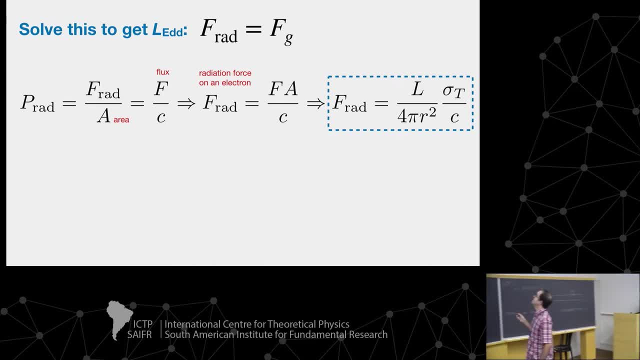 And then you write the radiation force acting on one electron in terms of the luminosity of the central system: okay, Sigma t is the Thomson cross-section. okay, The classical area associated to the classical radius of the electron. There is a simple way of understanding this result, okay. 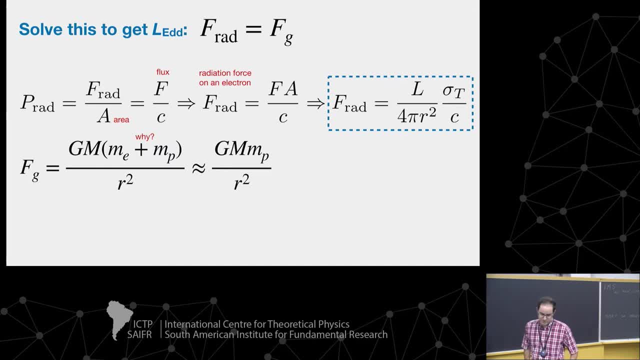 So now we characterize the gravitational force. okay, So we put the force. the gravitational force is carrying above both the electron and the proton. We have this approximation. So what we do is we solve this equation by putting this there and this there. 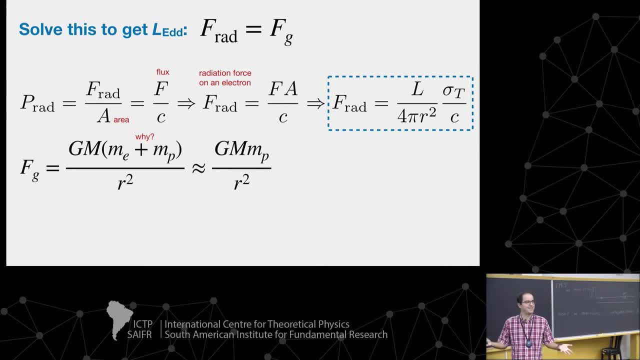 Very simple, much more simple than what you have been seeing the last week. okay, From what I heard, a little bird told me that you were having fun with the Vlasov equation. This is very simple. okay, So you solve this. 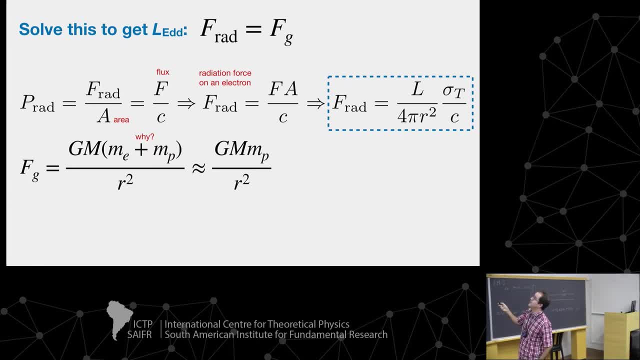 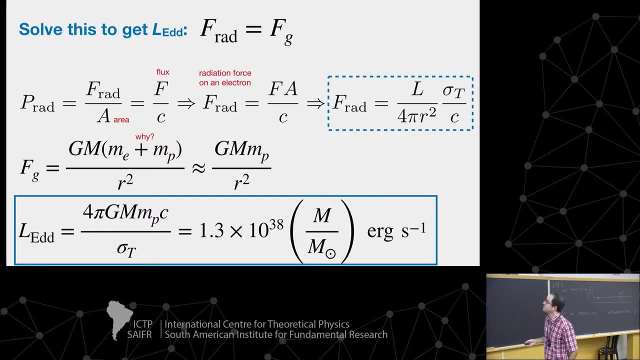 and you want to solve for the resulting L. What is the luminosity at which there is this equality? And the resulting L, the adding to luminosity, is this very simple expression. The expression has the property of the source of radiation, the mass. 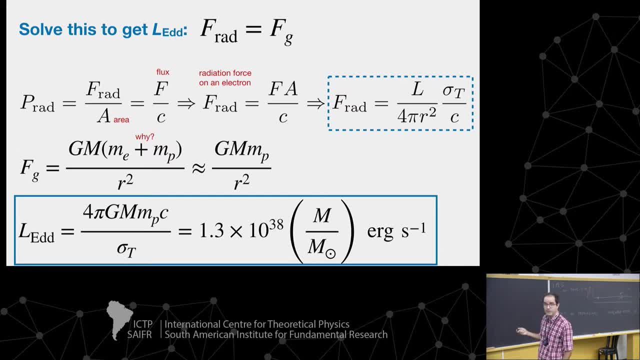 and the property of the infalling particle which feels the gravity, and the property of the particle receiving the radiation pressure in terms of the Thomson cross-section. If you write that in terms of the mass, this is the adding to luminosity as a function of mass. 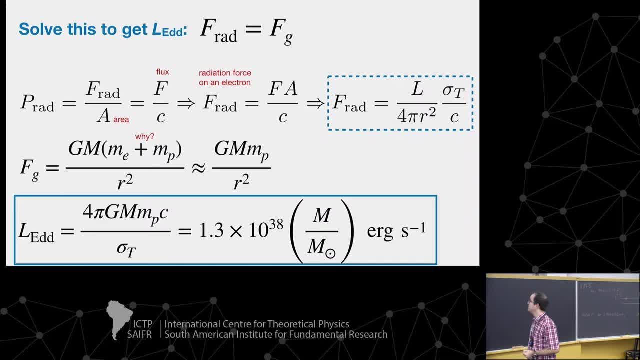 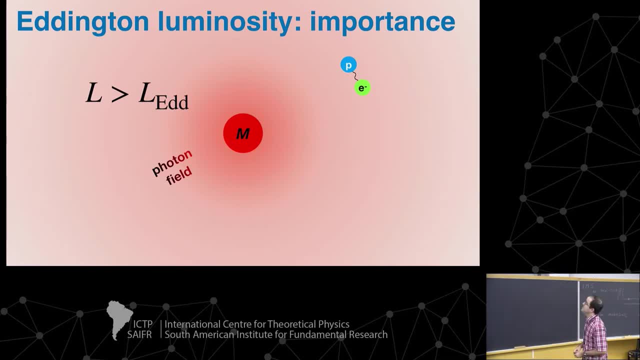 For one solar mass, for a central object of one solar mass, is 10 to the 38 Ergs per second. okay, What is the meaning of the adding to luminosity? now? The meaning is the following: If you have an infalling pair, 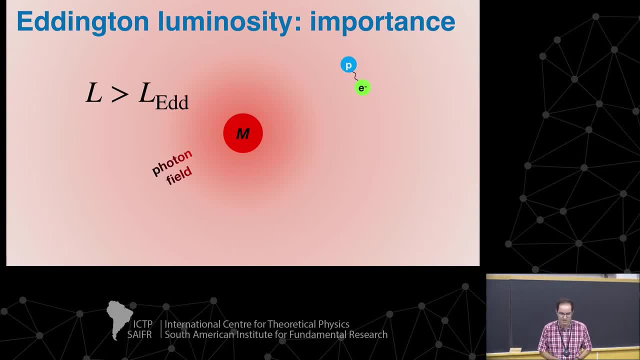 or if you have a plasma, of an ionized plasma of electrons and protons, okay, If the central object is radiating at above the adding to luminosity, what will happen with this pair If the luminosity of the central object is above the adding to luminosity? 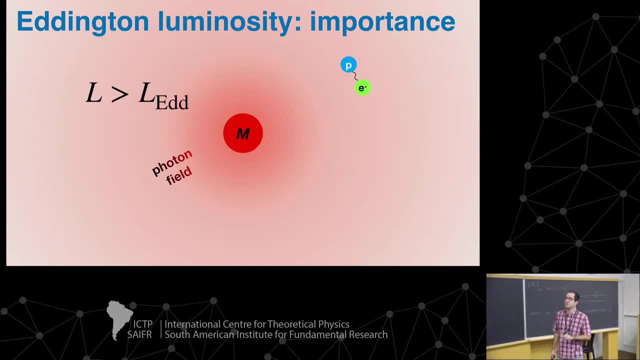 given the concepts that we, the simple concepts that we just described, what will happen with this pair? It will be like: oh, no, no, no, no, no, no, okay, It is there already. okay, So this is what happens, okay. 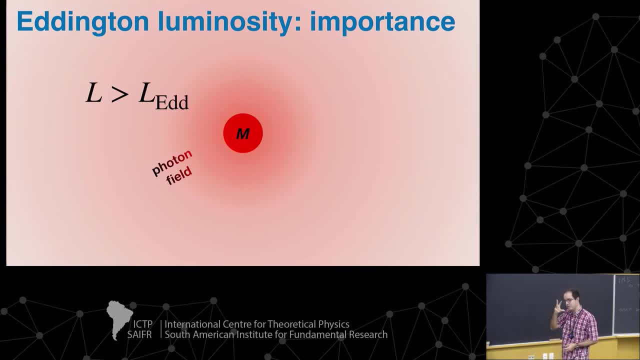 The importance of this concept is that it's giving you an interesting physical scale for the luminosity attached to the gravity of the central object. okay, In the sense that you know if the object is shining at above the adding to luminosity. 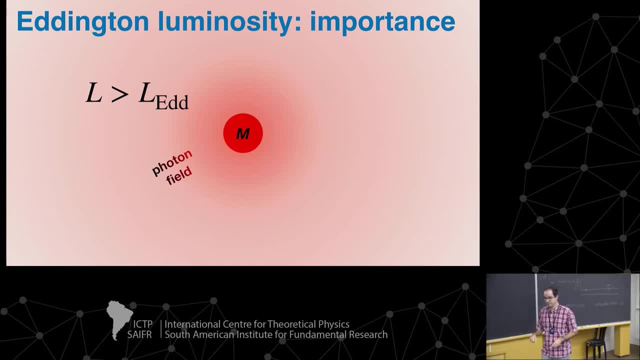 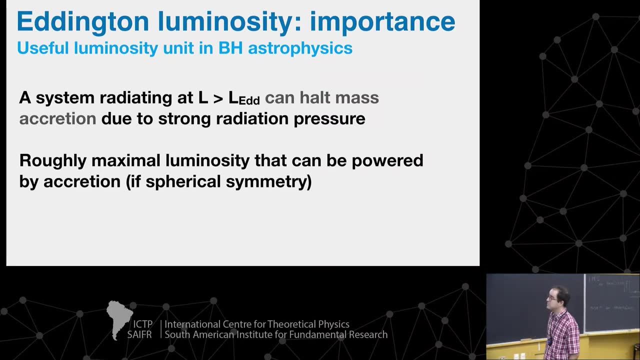 it will maybe impede further accretion. Okay, so this is what. this is the main importance. It's a very useful luminosity unit in black hole astrophysics And the adding to luminosity gives you roughly the maximal luminosity. 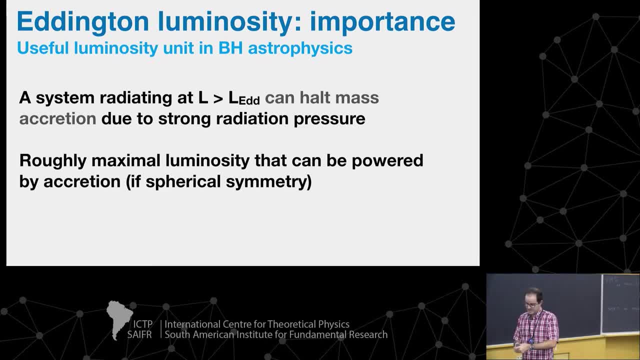 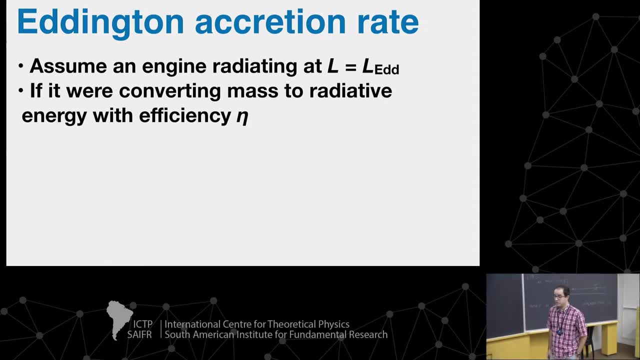 that can be powered by uh accretion. Now we define another object, another concept, which is very useful in black hole astrophysics, which is the Addington accretion rate. So to define the Addington accretion rate. 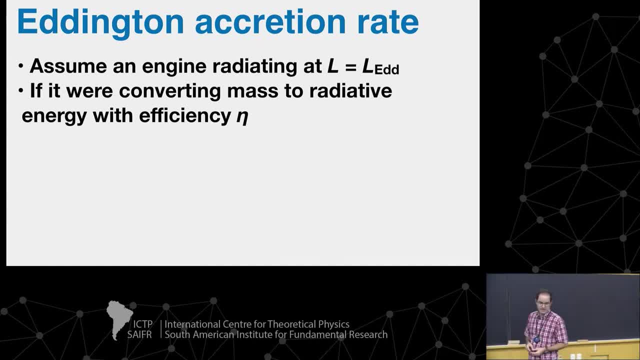 we have to assume there is again a central engine which is shining exactly at the Addington luminosity- okay, This is our working hypothesis to derive the concept of the Addington accretion rate. And we ask ourselves the question: what if this central engine were converting the infalling mass? 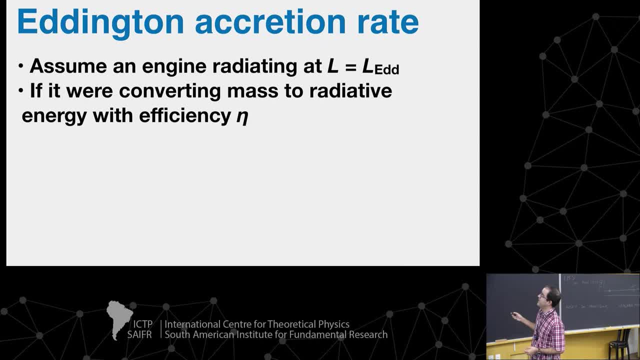 to radiative energy with an efficiency eta, let's say It can be 10%- 10% of the infalling mass being converted to luminosity mass to luminosity conversion. So the way we frame this is that we write the Addington luminosity. 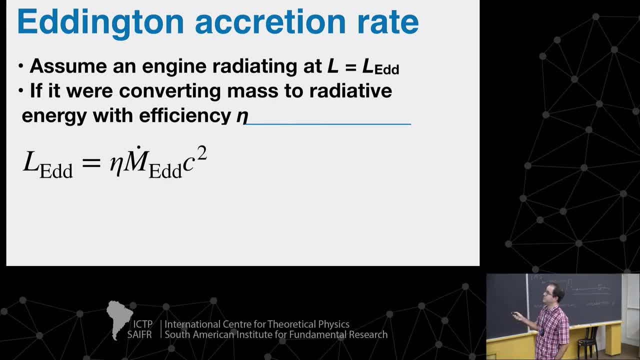 in terms of some efficiency of conversion of the rest mass associated with some influx of matter. So this is what we define as the Addington accretion rate. So the Addington accretion rate is precisely this concept, from doing this construction, this abstraction, okay. 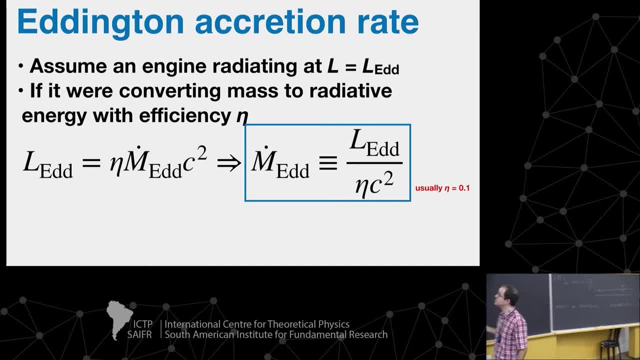 The Addington accretion rate is the Addington luminosity divided by some efficiency of conversion of mass to luminosity. Usually this eta is assumed to be 10%. Okay, Because quasars, most of lots of accretion black holes. 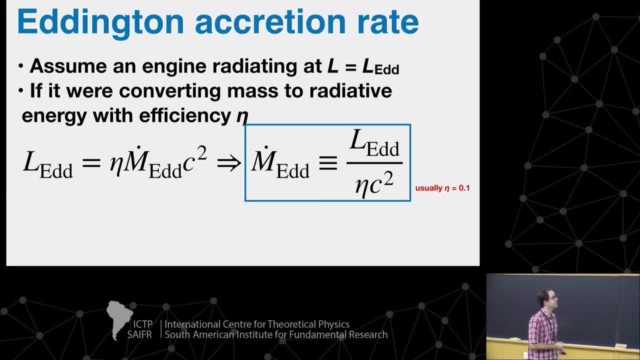 indeed have this efficiency of mass to luminosity of 10% And writing. in practice, the Addington accretion rate for a 10 to the, for a 10 to the 8 solar masses black hole for a 10% efficiency it is 3 solar masses per year. 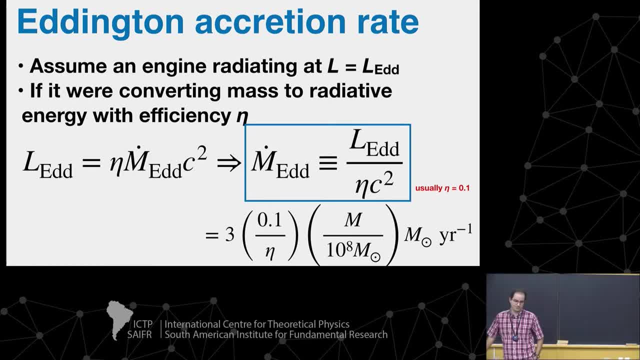 If you give 3 suns over an year to to a supermassive black hole with 10 to the 8 solar masses, it will shine at the Addington luminosity. okay, The accretion process will make the black hole shine. 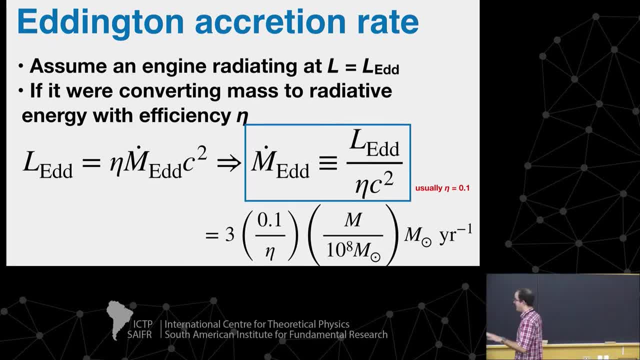 at the Addington luminosity. When I say shine, I'm not talking about Hawking radiation. okay, Forget about Hawking radiation having any interesting astrophysical consequence that we can measure now. okay, Maybe it has in the early universe. 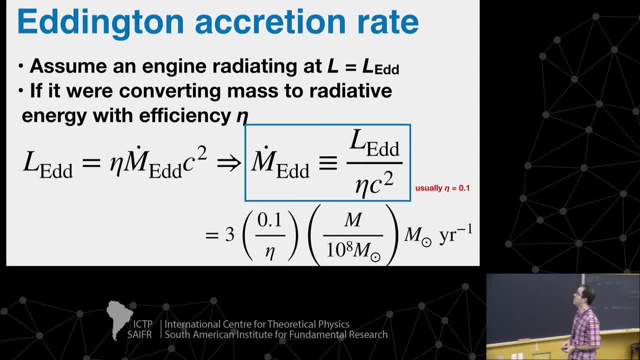 but astrophysicists don't usually worry about Hawking radiation. Okay, so Addington accretion rate. I think I'm almost over, right, The Addington. the Addington accretion rate is a very useful scale for feeding of black holes. 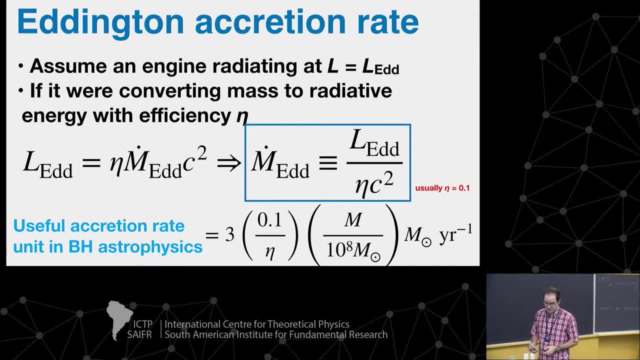 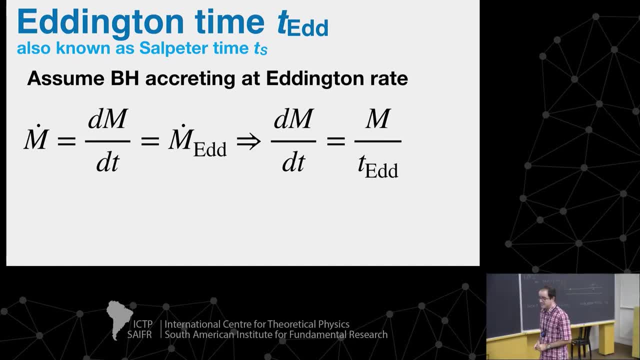 in the universe. And I will finish with a final concept here, very simple concept. before I move on to to questions, There is a. the final concept that I will talk about here is something that we call Addington time, or some researchers call it Salpeter time. 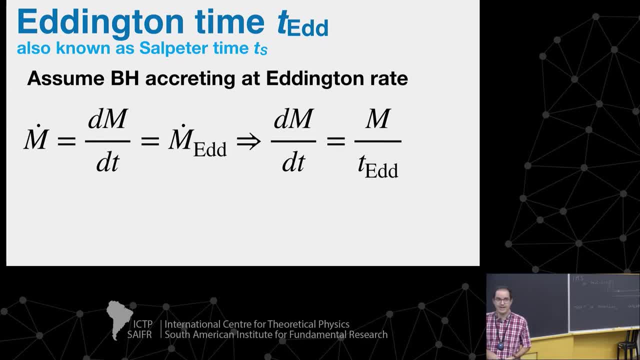 I will call it TED. Okay, Addington was a very, very good astrophysicist in the early, the early 20th century. okay, There was. there was a clash between Arthur Addington and Chandrasekhar, and Chandrasekhar mostly won. 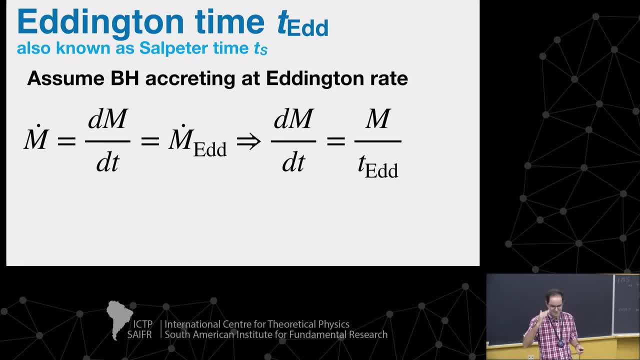 The clashes that they had about neutron stars and other things and white dwarfs. Okay, so Addington time is the following: How do let's assume there is a black hole? accretion at the Addington rate that I just defined. So we write the accretion rate as the time derivative. 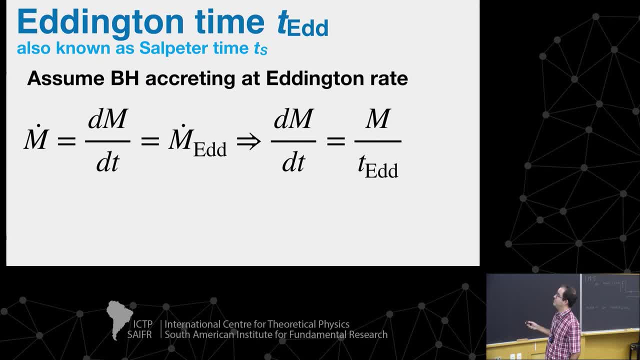 of the of the mass of the central object. okay, So if you keep feeding the central object its mass will go up. So we assume it's accreting at the Addington rate. so we make this equal to the Addington accretion rate. 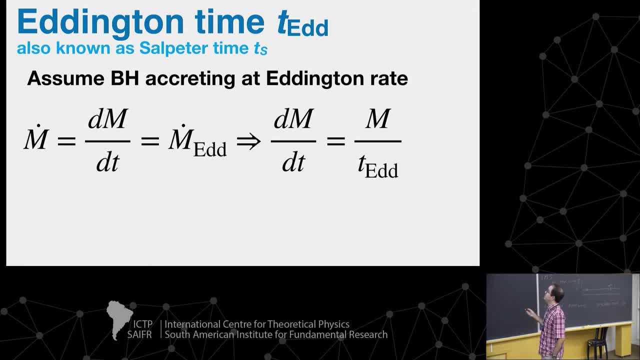 and we solve this differential equation and we define the Addington, the Addington time, as this time scale that shows up here on the right hand side. Okay, this is the Addington time scale. What is the solution to this differential equation? What is the mass evolution over time from this equation? 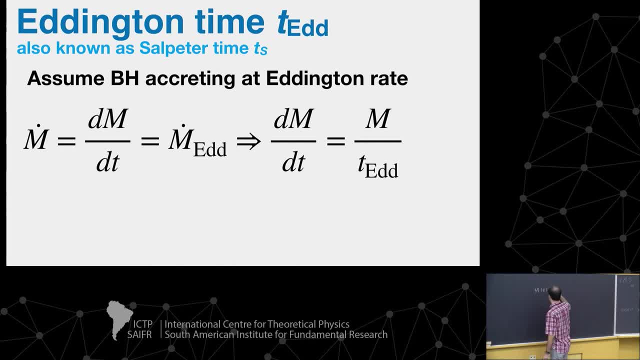 Well, you know what is the mass over time evolution, right? So if the black, if the black hole is accreting at the Addington rate, it will, its mass will go up exponentially with an E folding time of the. why am I using a laser here, 10 centimeters from the? 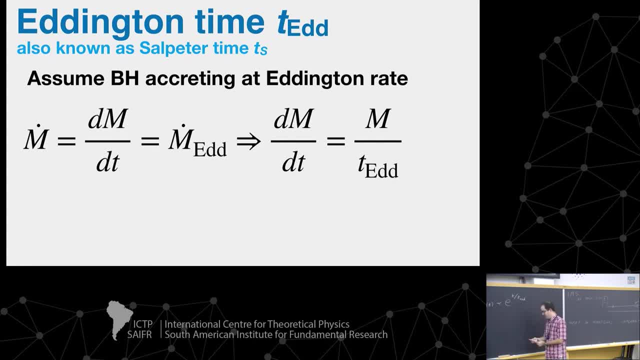 Sorry, sorry, sorry. So the E folding time of the black hole is the Addington time scale. It means that the mass of the black hole will double every two years, more or less. okay, And this is the Addington time scale for 10 to the 8th. 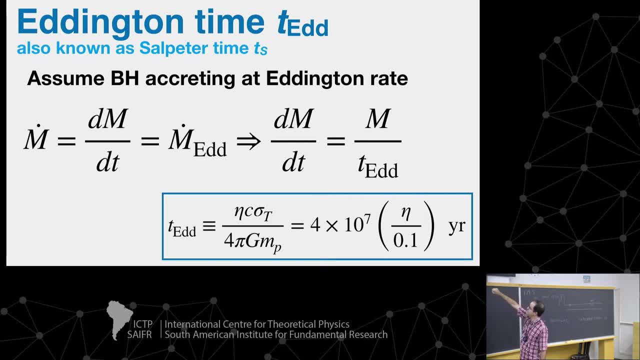 for the mass should be here. No, no, no, no. okay, So this is the Addington time scale. It's for 10 to the 7 years for a black hole accreting at the Addington accretion rate. 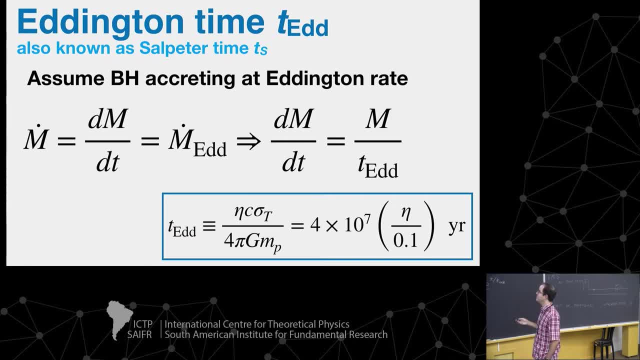 This means that the mass will double every 10 to the 7 years. This is an important time scale for cosmological understanding of the growth of black holes. okay, And that's it for now. Thank you very much. Any questions? So I have two questions. 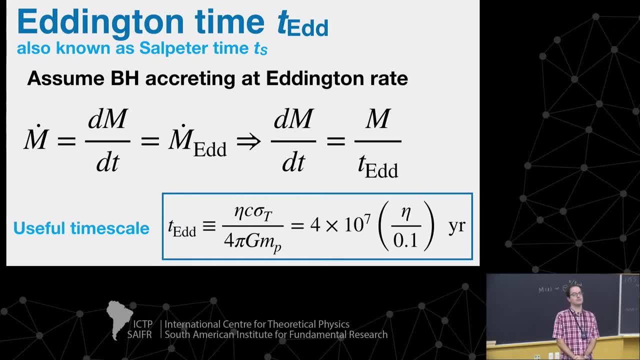 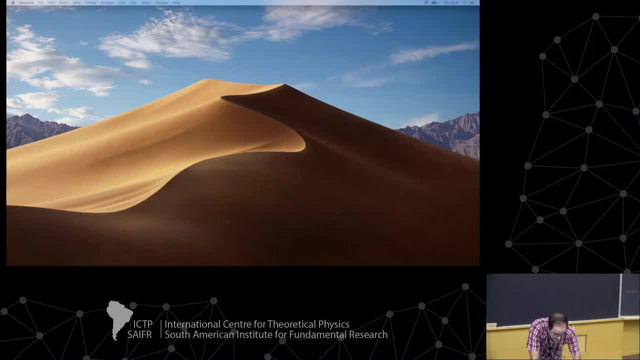 The first is: what classifies a black hole as supermassive or not supermassive? Ah, yes, okay. So what classifies? I have a slide for this, but I will describe you. It's the mass. it's only the mass. 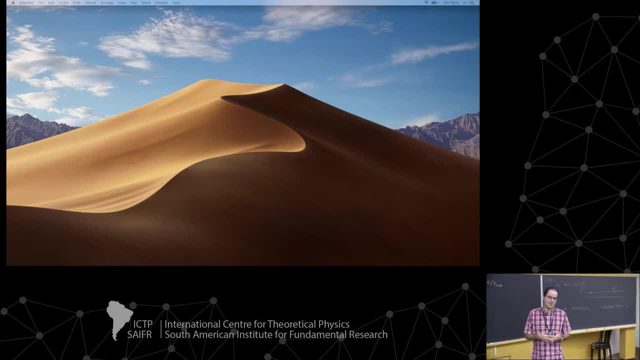 So supermassive black holes- it was kind of an arbitrary notation, okay, But supermassive black holes they have masses above roughly one million solar masses inside the event horizon. okay, So if you look at a galaxy and you measure the mass of the central black hole, 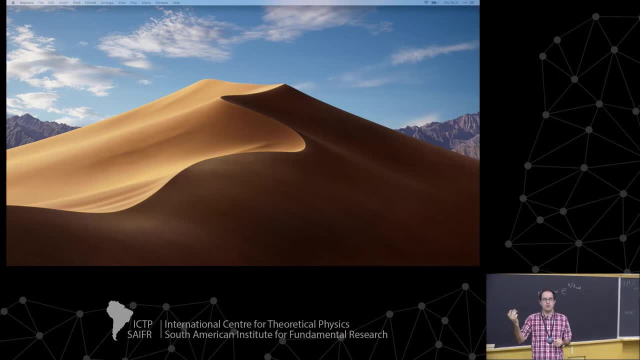 and it has over a million solar masses. we call it supermassive black hole, like the song by Muse right. There is a song by Muse right. Yeah, Fabio, you are laughing, don't you know? If it were a Ramon song, you will know. 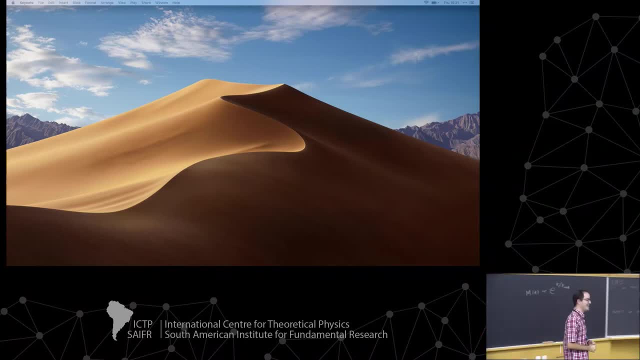 Okay, And a stellar mass black hole. it's usually stellar mass black holes we define as having a mass very close to one solar mass. okay, So if the mass of the black hole is close, very close, to one solar mass, between- okay above- between three solar masses and 60 solar masses. 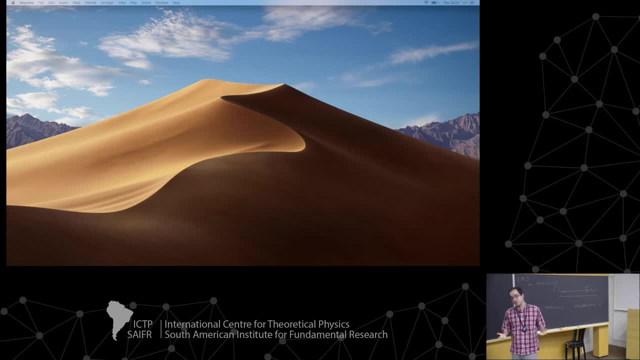 we call it a stellar mass black hole And there is also a putative class of intermediate mass black holes which should have. they are in between the two extremes, okay, So usually a thousand solar masses, ten to the fourth solar masses. 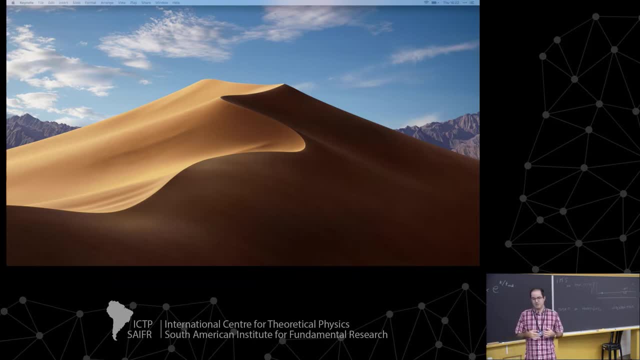 So these are really we want to, we like to classify things, and so we put these different tags for them, depending on the mass scale. And it turns out that actually these tags are relevant for astrophysics because the, apparently, the growth modes of these black holes are different. 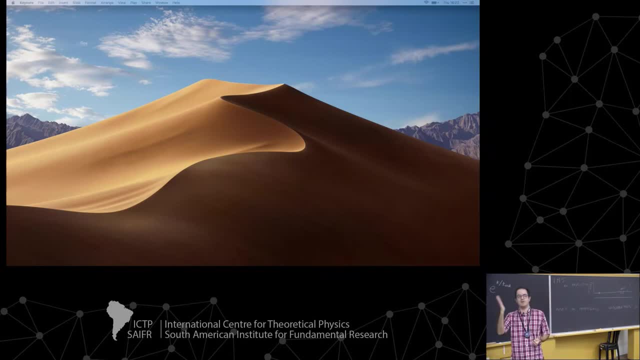 depending on whether they are stellar, mass black holes, supermassive or intermediate. okay, What's your question? Was your question more related to how you form them or just how you define them? Was your question more related to how they happen to exist? 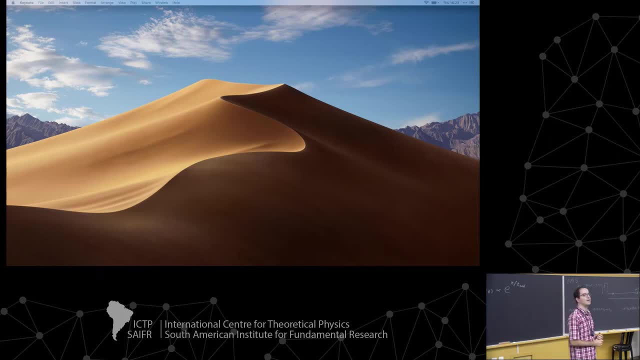 or how do you define them? How do you define them? Ah, okay, Yeah. well, the question by Fabio is: how do you form this supermassive? well, it was not a question, but I will. how do you form supermassive black holes? 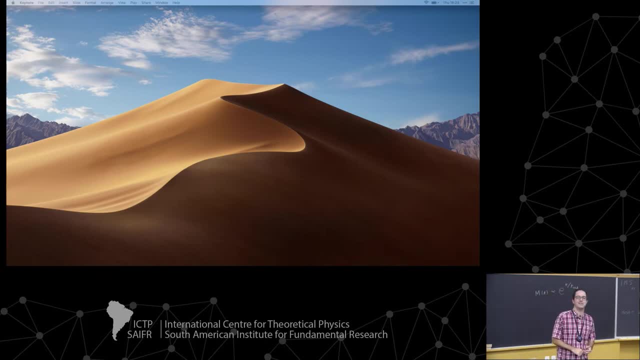 We don't know. okay, This is one active area of research here. Yeah, it's one active area of researchers and one active area of research. Suffice to say, we don't know. There are three channels that we think there is some kind of instability. 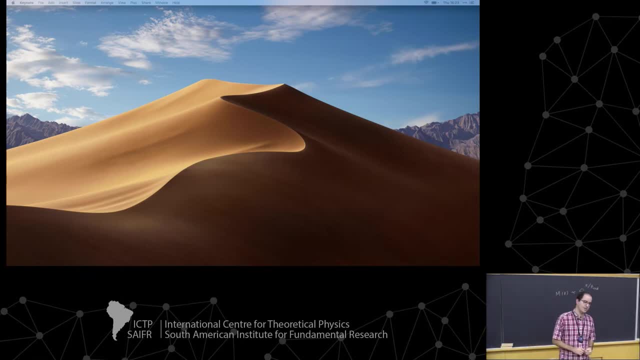 that produces something very massive at the early times of the universe. By early times I mean in the first billion years of the cosmological evolution of the universe, And there is somebody here on this audience which is an expert in the seed masses of the first supermassive black holes of the universe. 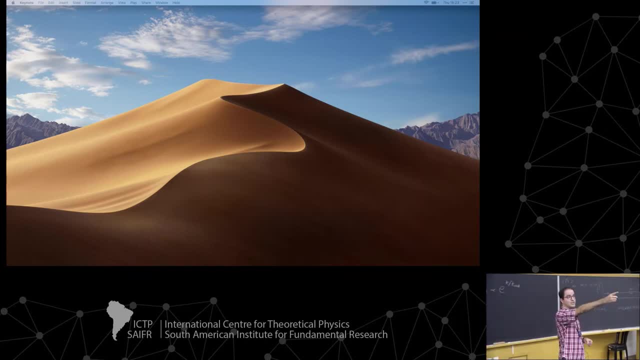 And this person is there with a very nice shirt with pandas. It's very easy to recognize him, So we can chat about this. It's a very interesting topic, Yeah, And the second question is: you said that AGNs have occurred in space-time. 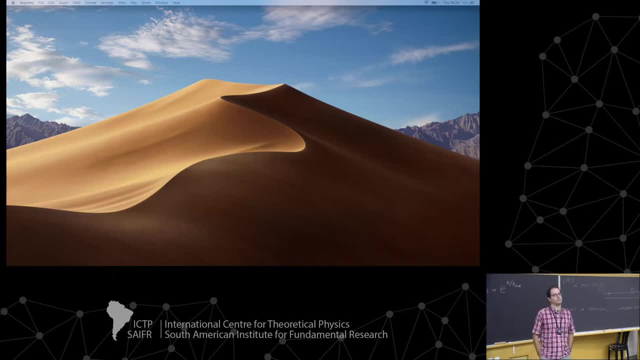 So that means the black hole is just space-time. It's spinning but have no charge. Can you have charge in the black hole of an AGN with Kern-Newman space-time? I forget what is the Kern-Newman. The Kern-Newman is the space-time where you have charge. 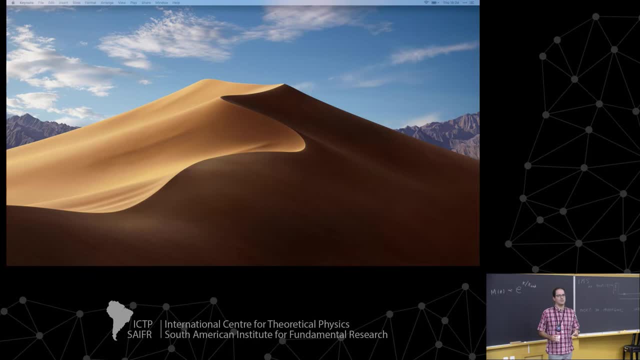 and no spin. right, The spin is zero, but the black hole is charged. No, it's spinning and have charge. Spinning and have charge. Ah, okay, Kern-Newman. Well, so this is the thing We know, that black holes must spin. 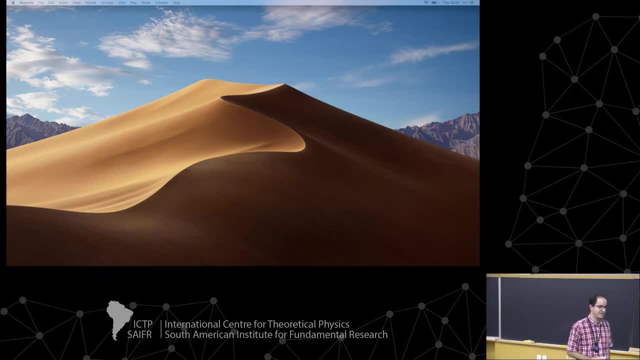 Every black hole in the universe must spin at some point in its history because of conservation of angular momentum. okay, Let's think. okay, the origin of small, tiny, cute black holes in our galaxy? Our galaxy has millions of stellar mass black holes. 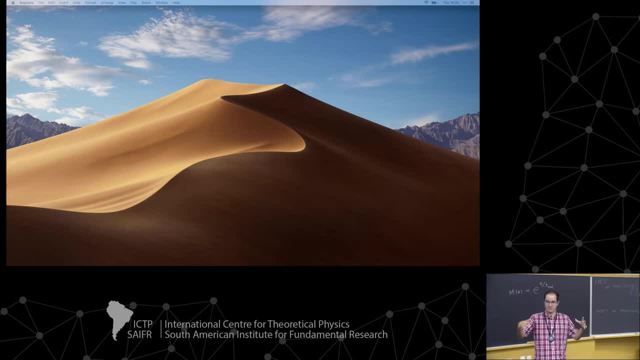 And many of them. they are born from the depths of massive stars with masses above 10 solar masses or something like that. okay, So the thing is, stars are usually rotating, okay, To different degrees. they have angular momentum. okay, I don't think you will find a star which is completely static, okay. 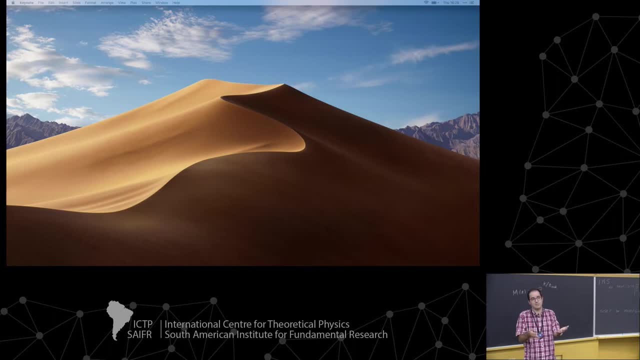 And as the star collapses, what happens with the spin of the star? okay, This is very easy. If you dance ballet, I probably suck. I never tried dancing ballet, But all of you saw this example in Physics 1, where there is a ballerina. 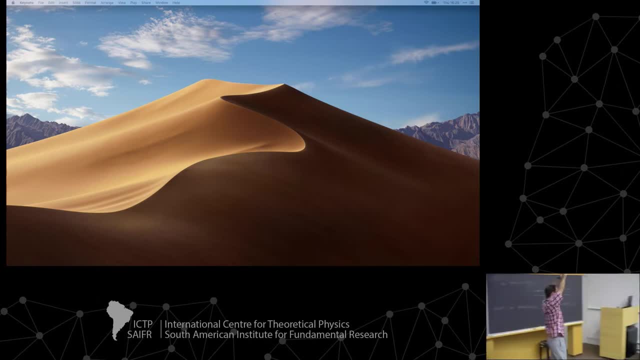 and then the ballerina is doing this and then she's just like and spins faster, right. The same thing happens with a collapsing star. It will start spinning faster And the resulting black hole will be born spinning okay. So spin certainly is important. 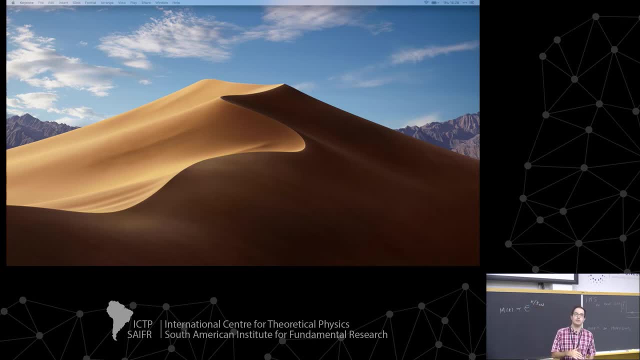 at some point of the life of black holes. We do not know if supermassive black holes are rapidly spinning or not. That's a different question, Charge, we know it's irrelevant, okay, Because what happens If you take a black hole? 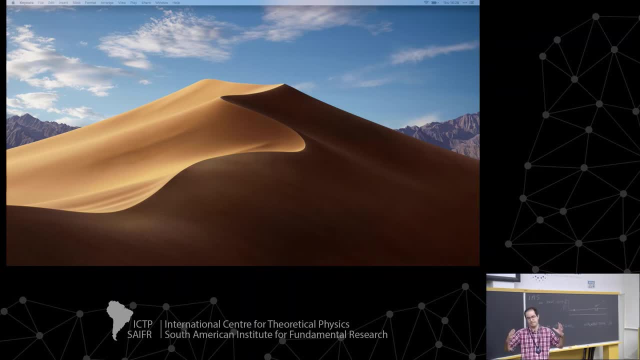 and you throw a lot of electrons. you take a block of pure electrons and you throw in a black hole and you try to add negative charge, a global negative charge, to the space-time. The thing is that it will put a temporary negative charge, but then this negative charge. 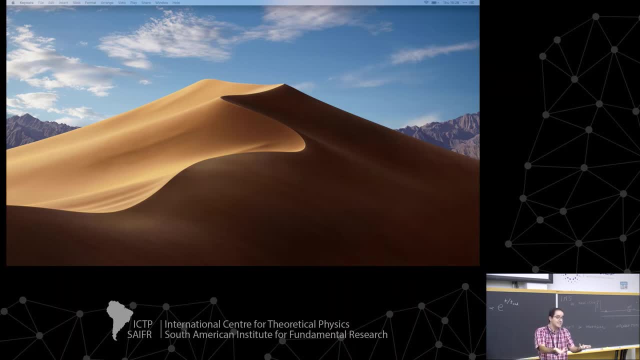 will start pouring out, It will start pulling positive charges, okay, And that will result in the discharge of the black hole in a very quick time scale. okay, So this is a qualitative argument. of course, The relativity physicists, they already proved. 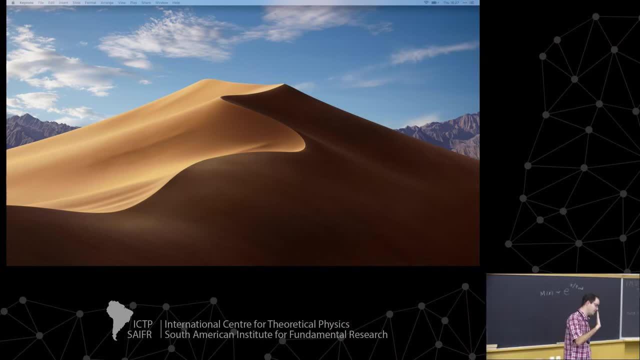 they have arguments, very strong arguments, why we do not. black holes will discharge very quickly. They will get neutral very quickly, okay, And don't be remember this thing called pluralistic ignorance. okay, Sometimes you think that everybody understands what's being discussed. 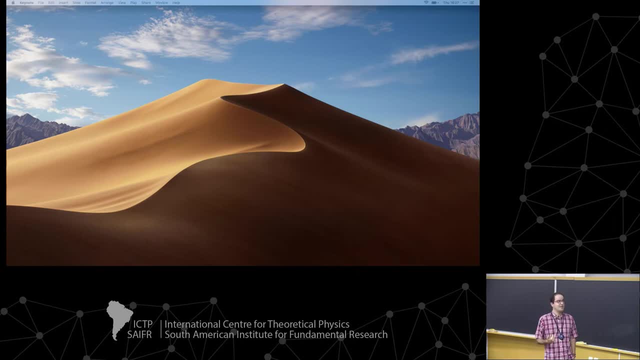 and you are afraid of asking a question to embarrass yourself. but this is your. what is pluralistic ignorance? It's an asymmetry between what you think and reality. okay, But usually people are as lost as you. okay, So if you are the brave first person, 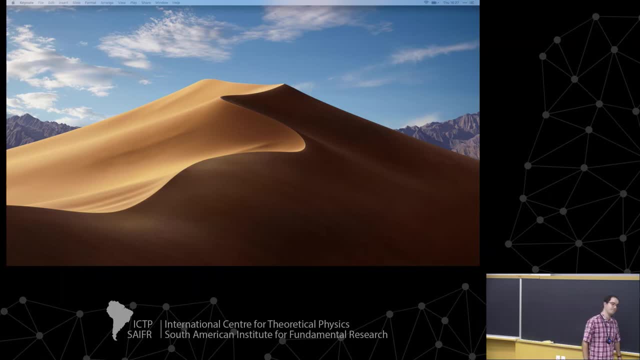 to ask the first question. more questions will follow, okay, Hi Here. Okay, At the beginning you mentioned that accretion disks are collisionless plasmas and should be properly attacked with kinetic theory. but people use MHD codes. 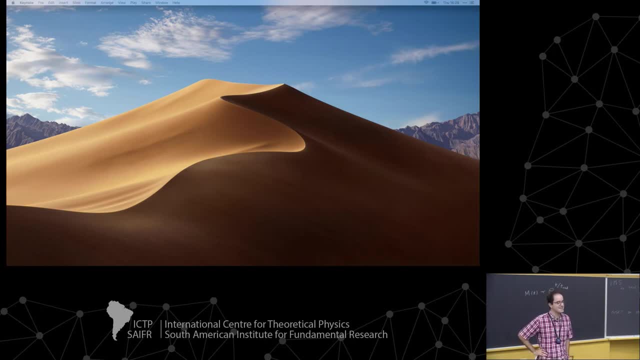 to perform simulations, and how much wrong could the results be? I love it. How far I love it. I love it, Thank you. Thank you for this question. Well, we have, when you talk with plasma astrophysicists. 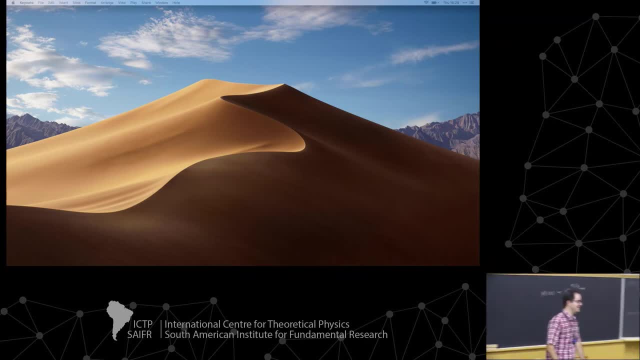 they love to do MHD. All the universe is MHD, The atmosphere of a galaxy cluster. let's use MHD to tackle that. Let's use MHD to tackle black hole accretion disks In many cases, as I mentioned. 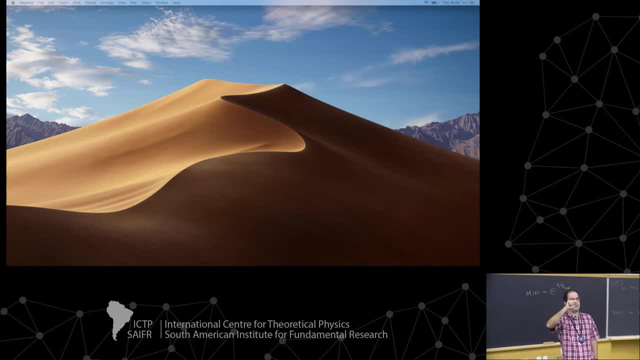 you can do a plot of the mean free path versus. you can make some nice plot to characterize the plasmas of this low luminosity agents and they are in the collisionless regime. okay, And quite honestly they might be. they're probably doing close to. 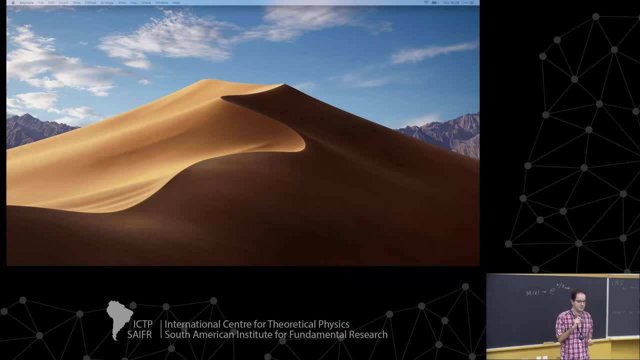 okay, I will not call it a zeroth order approximation to the physical truth, first order approximation, but this is not really answering you anything. I will give you some more concrete examples. okay, So for instance, for non-thermal electron heating. 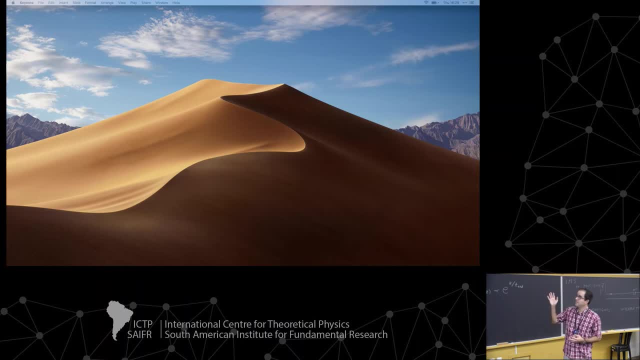 in these accretion disks, in objects like M87, nobody knows how to do it, so you cannot really trust anything about non-thermal that is happening in the community If you hear somebody talking that everything is MHD. everything in black hole astrophysics is MHD. 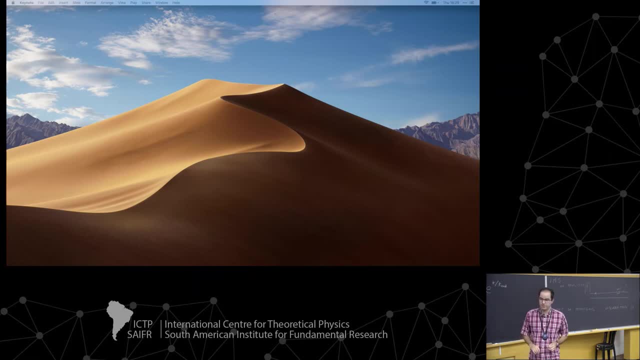 that's a red flag. okay, Be very careful. A more intellectual, honest is saying: look, you know we are doing, we know this is. I will not call it wrong. okay, because I don't want to buy fights with colleagues. 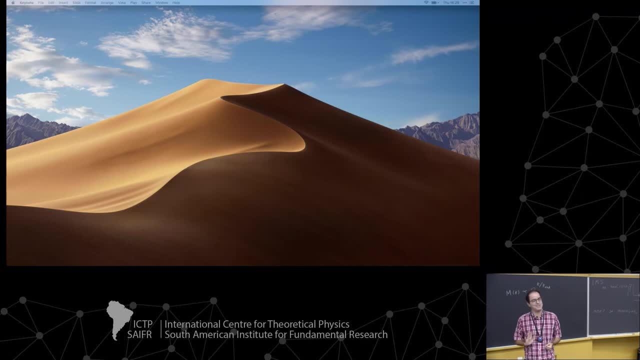 but it can be missing a lot from the physical truth. okay, But be suspicious of people that claim that MHD solves everything. It's just an. it's an approximation, which is there. are you have a lot of codes that do MHD? okay? 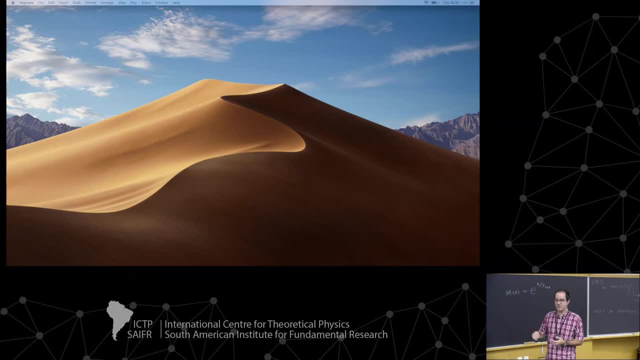 And basically one or two codes that do kinetic, general relativistic kinetic theory. so my advice is: be suspicious, okay. if you hear somebody saying that MHD is the answer to life and the universe, okay, I can give you a more concrete answer. 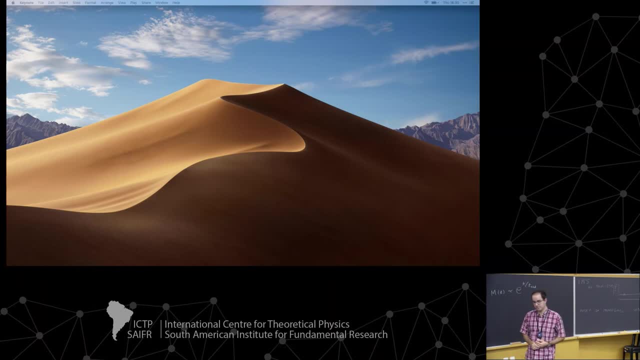 in a one-to-one talk. okay to your question. Sorry for being vague at this point, Hi. My question is: what is the origin of those jets and why do they exist? Next lecture Curve: space-time with magnetized plasma and large-scale magnetic field lines. 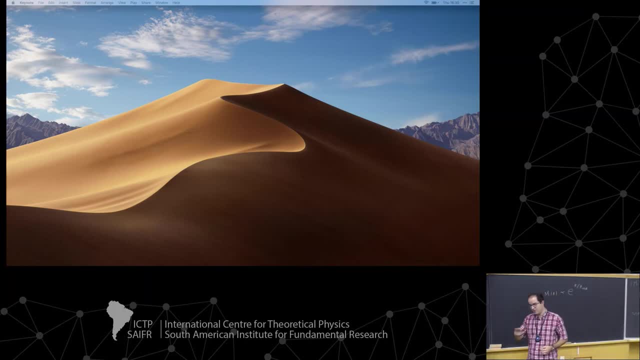 For now. Tomorrow, the more complete answer. So, hi, It's more like a curiosity. So you mentioned Hawking radiation. Is there any way to measure it, directly or indirectly? No, No, No, No, I want to prevent my computer from sleeping here. 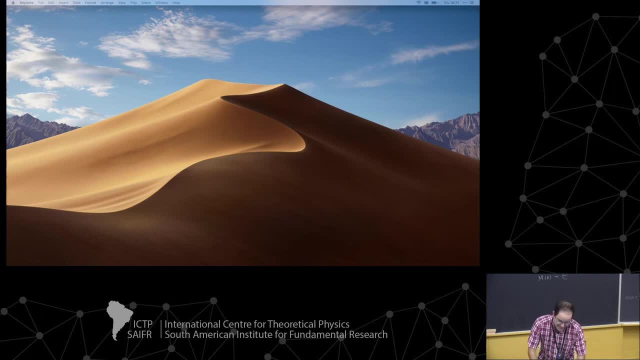 The full answer is the following: It is reasonably. it was not easy to derive the Hawking radiation. It was not easy for Stephen, even for Stephen Hawking it was not easy. Maybe it was easy, I don't know. I don't know. 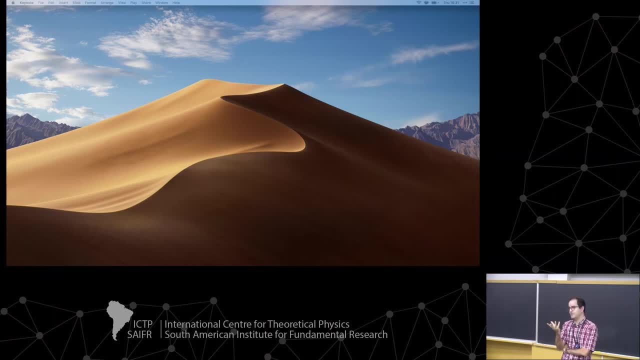 But the result is very simple to use The resulting formula for the temperature, the black body temperature of the near horizon, of the near horizon surface, near the black hole. It's a very simple formula of black hole thermodynamics And you can compute as a function of mass. 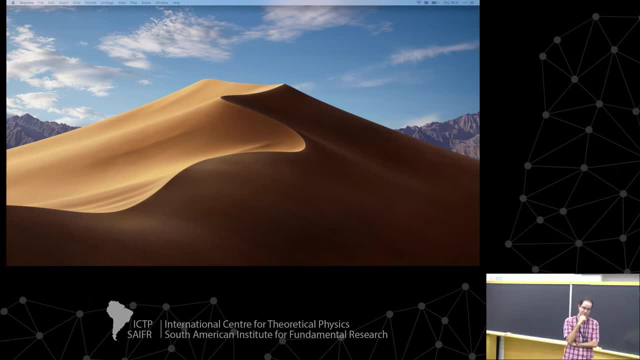 the temperature of the resulting radiation- the thermal radiation that has a very nice black body shape- from the close to the event horizon. And if you do this calculation for the temperature of the resulting radiation- the thermal radiation that has a very nice black body shape. 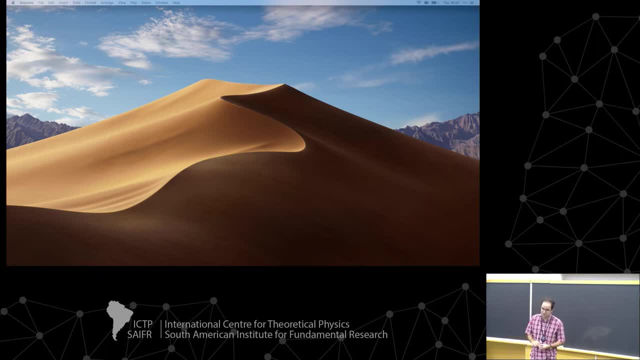 and if you do this calculation for a supermassive black hole, I have to. I get this question very often and I never remember the result. But I think the luminosity is about 10 watts, It's something like that. It's of the order of watts. 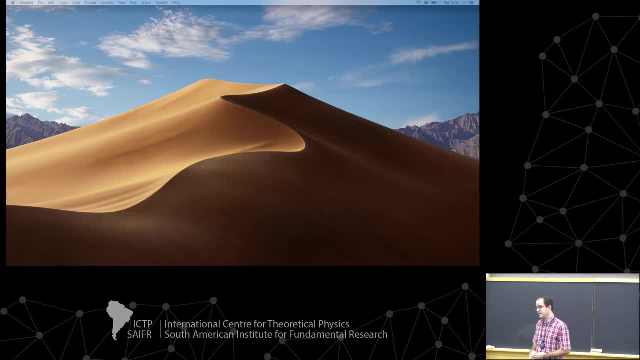 comparable to the luminosity of one of these lamps here And that's impossible to detect. If you were God, if you believe in God, God can probably detect. I'm an atheist, let's make it clear. But if you were God you could probably measure. 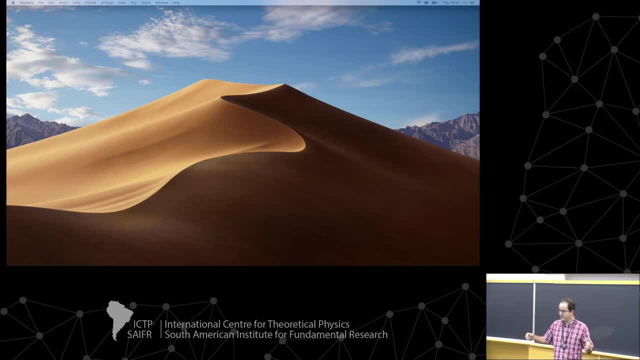 this Hawking radiation. But if you give one kilogram of gas in the accretion disk it will probably shine brighter than this Hawking radiation If you just give the tiny bit particles and they have enough density to start having magnetorotational instability. 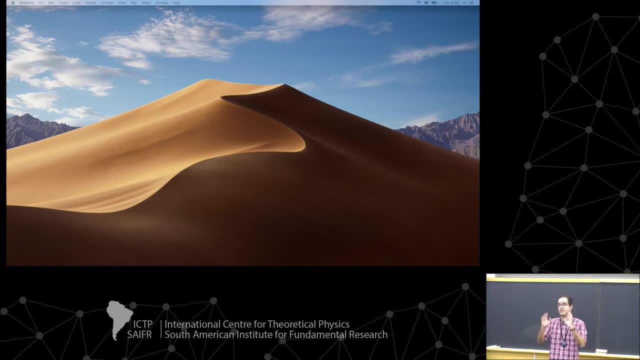 have friction and release heat as radiation, it will shine brighter than the Hawking radiation. That being said, there are some heroic efforts happening in at least one place of the world in an Israeli lab led- I think it's- the Hebrew University, led by Jeff Steinhauer. 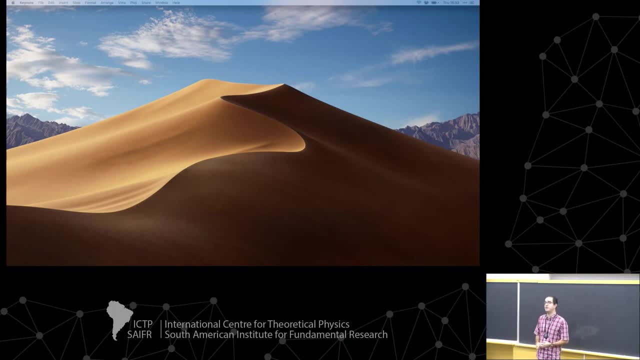 And Steinhauer is doing some very interesting results. that were some very nice calculations by always Bekenstein, Jacob Bekenstein, very famous physicist in relativity the golden age of GR, And he noticed very interesting that you can, depending on how you frame the equations- 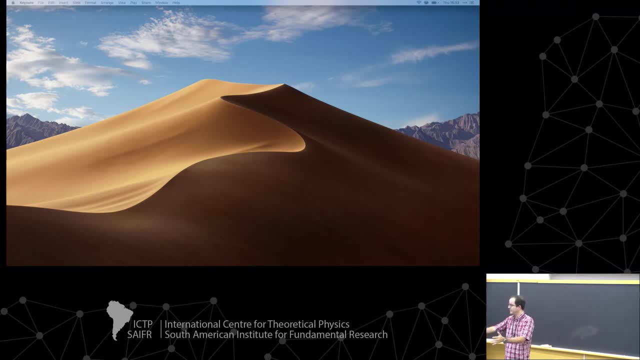 you can make a system with a fluid without gravity that follows the same equations as a black hole with a gravity Fluid-gravity correspondence. I'm not talking about ADS, something, something dualities, which fascinate most of the physicists in IFT, this duality. 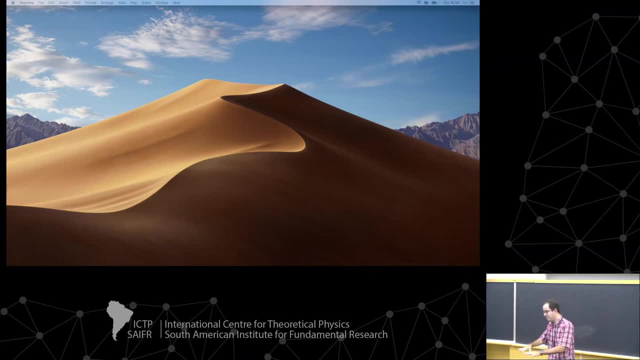 And then the hope of Steinhauer is: by playing with the speed of sound in the fluid, with a Bose-Einstein condensate and by playing with the speed of fluid, his hope is to create some kind of analog horizon. It's not an event horizon. 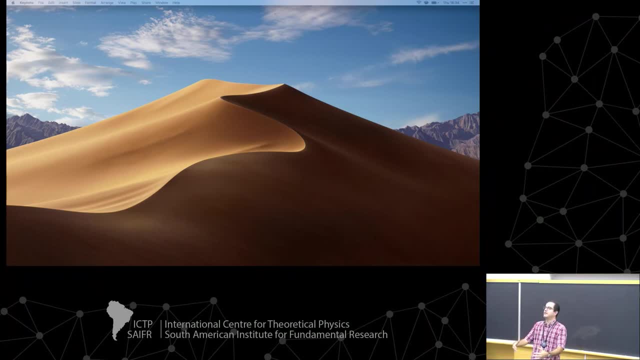 in gravity. It's an impostor. It's an impostor. It might be fake news in the sense that we do not know if that will really teach us about gravity, But they claim there was a Nature paper a couple of months ago and they claim they're seeing the. 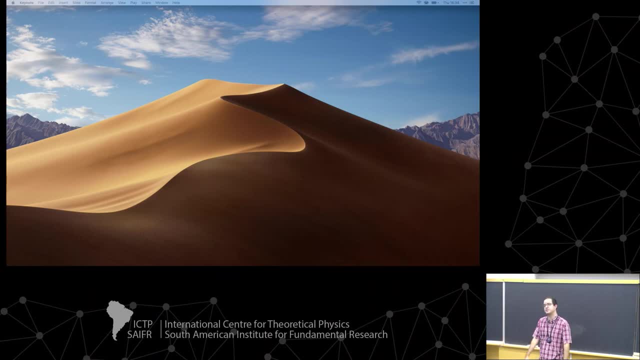 analog of Hawking radiation in this table-top Bose-Einstein condensates. Again, word of caution, that's not gravity, that's not a black hole. It's a black hole analog. It's the same thing that I'm trying to give an analogy. 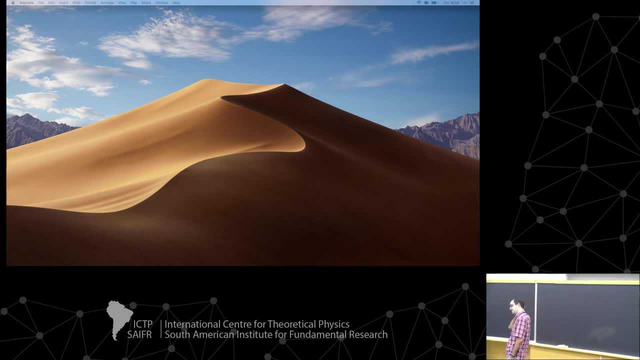 I'm trying to come up with an analogy here Is this: I cannot come up with a cool analogy, I'm sorry. It's the same thing as you dating. let's say you want to date Chris Hemsworth if you like, Chris Hemsworth, the Thor. 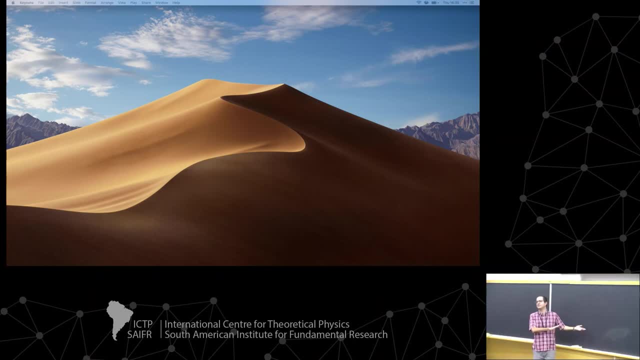 And you are dating somebody that kind of looks like Chris Hemsworth, You say, oh, this is Chris Hemsworth. I can figure out things about the life of Thor by dating this person. This is the kind of comparison we are doing here. 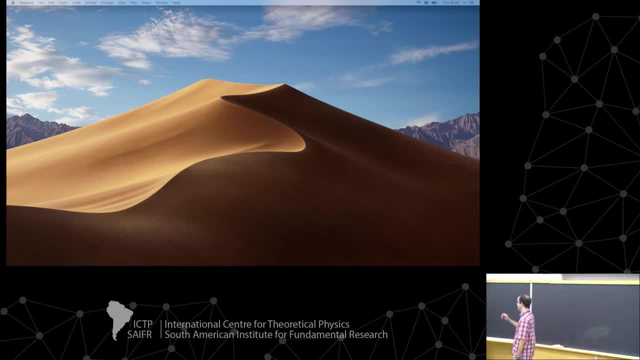 It's not Thor Or, I don't know, Gisele Bündchen. I'm not sure I'm following the argument. Anyhow, You are not doing the real thing. You are not doing the real thing. That's my analogy. 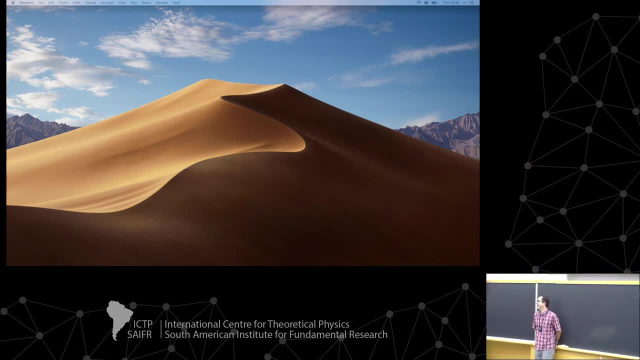 We got to that, talking about the Hawking radiation and the creation of an imposter What Event horizon from which the Hawking radiation might supposedly escape. That's how we got there right To do the analogy. Yeah, Did it answer your question? 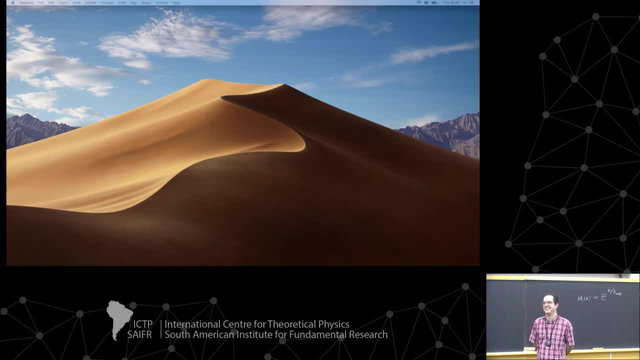 Oh good, Is there any other question? It was a terrible analogy. I'm sorry. I really tried. It was the first thing that came to my mind. It wasn't appropriate to talk here. There was another analogy that was not appropriate to talk here. 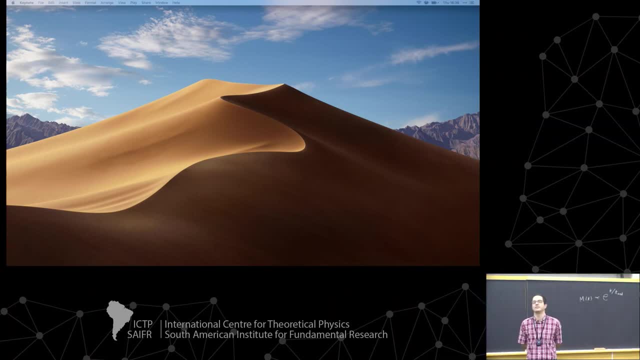 No, it's being recorded. Regarding the angular momentum, describing the black hole. what does A equals zero mean? A equals zero. A star equals zero. A star is the spin of the black hole, as we learned. A equals zero means that the angular momentum 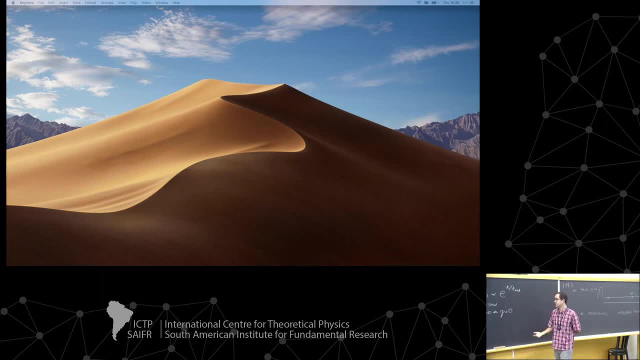 of the black hole is zero. The black hole is not spinning. That's the same as saying that this is the Schwarzschild solution. The spacetime is not doing any kind of frame dragging in general relativity. But you said that every black hole 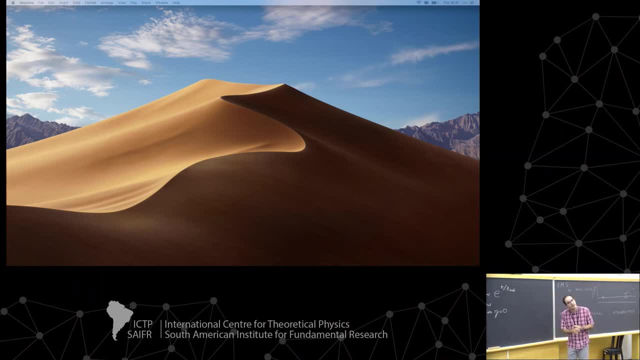 that has been observed is spinning, so this is purely theoretical. Okay, okay, So I have to be careful here to phrase things carefully. Physically speaking, we can expect most black holes to be born with some amount of spin, So they will be born. 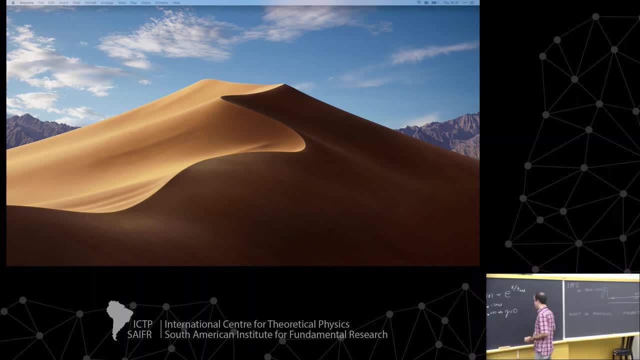 with some spin that is more or less different than zero. Okay, But we do not know what is the long-term evolution of the spin parameter for a given black hole, Especially for supermassive black holes. The reason is that you have a nice 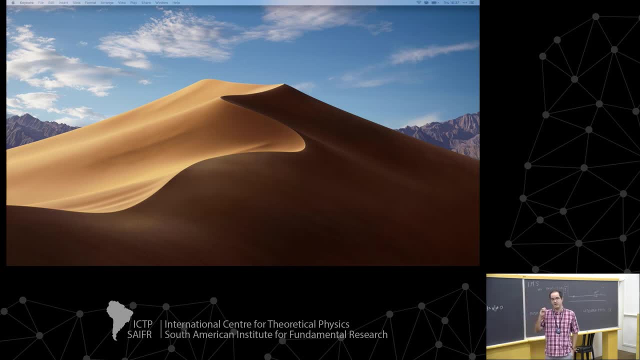 or not so nice black hole sitting at the center of a galaxy, and the galaxy is feeding that black hole with gas that is losing angular momentum for different reasons, falling towards the center of the galaxy, and the gas is carrying angular momentum to the spacetime. So, depending on how the gas arrives, 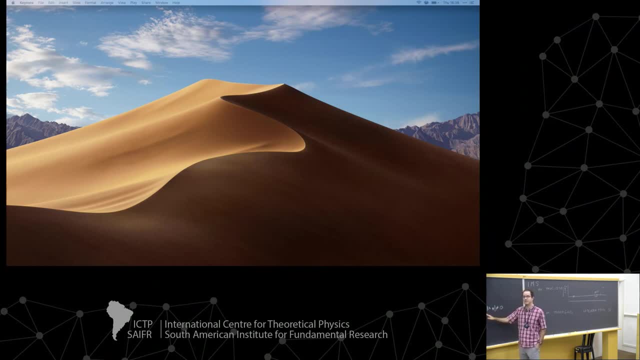 at the center of the galaxy. it can either do it retrograde, negative or positive. But there is another thing that changes: if there is a whole planet, if that star is being created by the black hole, I don't know, depending on how that star works. 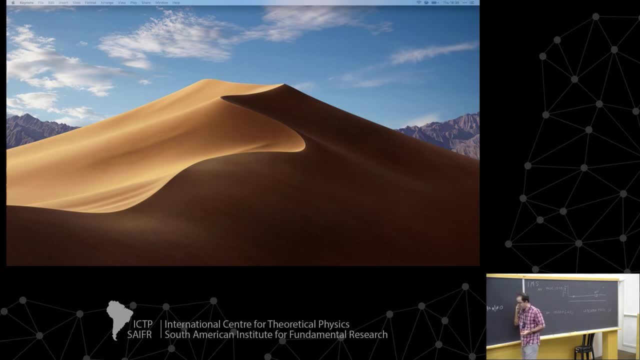 it will change significantly the spin of the black hole. If there is another black hole crashing in that black hole, it will completely mess up the spin. So that's why I say they are born with non-zero spins. but we do not know the long-term evolution.